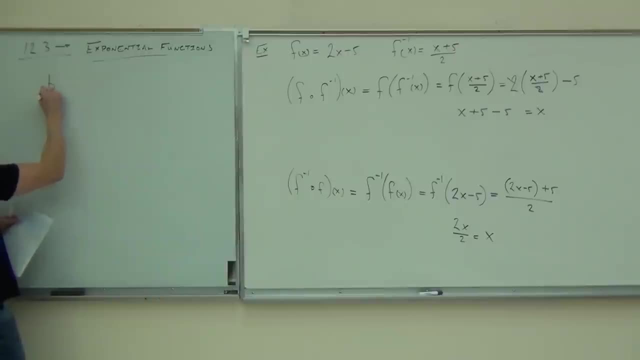 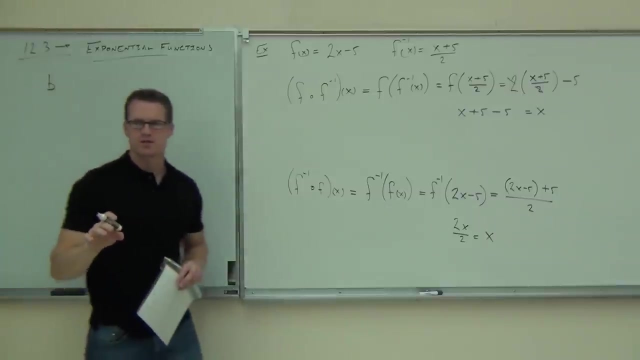 So we got to talk about an exponential. Every exponential is of this form. You're going to have B to now. this is going to be weird, right? Because normally we have. we have, like X raised to some power right, X to the one-half power will be a square root. 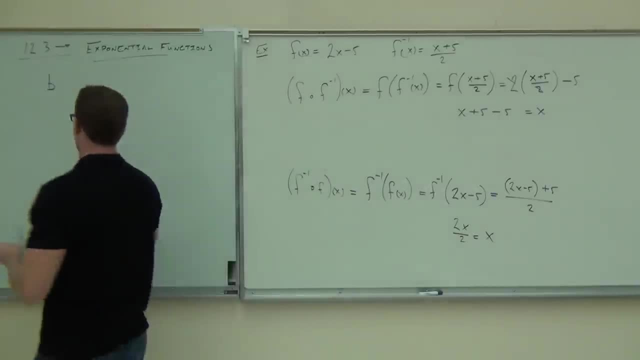 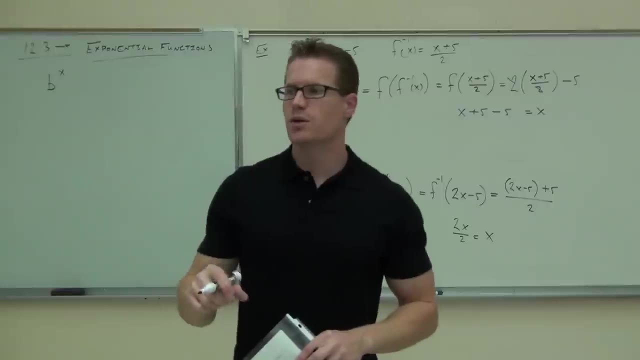 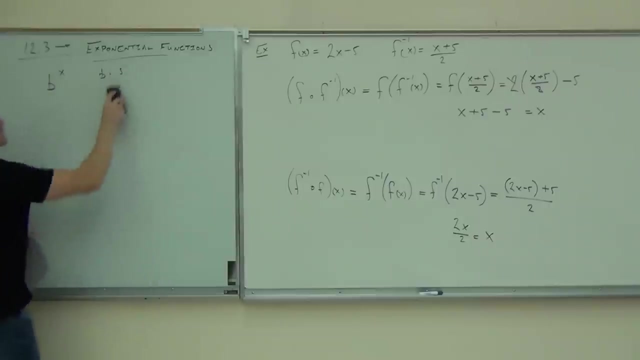 X to the third power will be a cubic. X squared is a quadratic. Now we have this, We have some exponent. that is our variable. B is called a base. It's a number like two or five or one-half. B is our base. 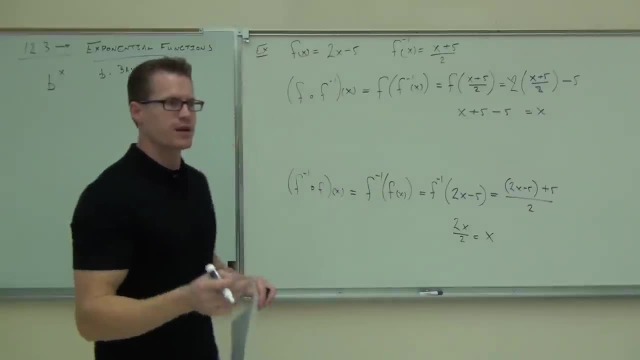 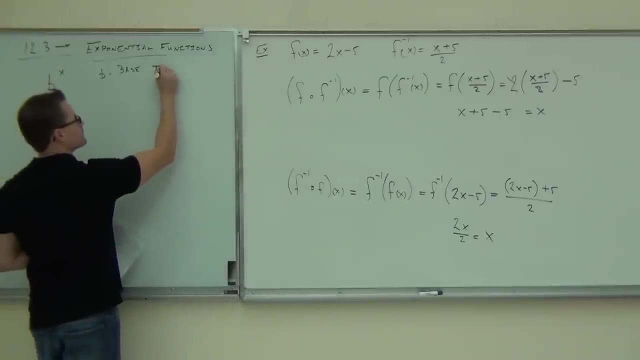 B does not change for your exponential, for whatever I give you. So if I say B is two, it's going to be two for as long as I tell you. Can I do the KAI? I get it right Again. question. 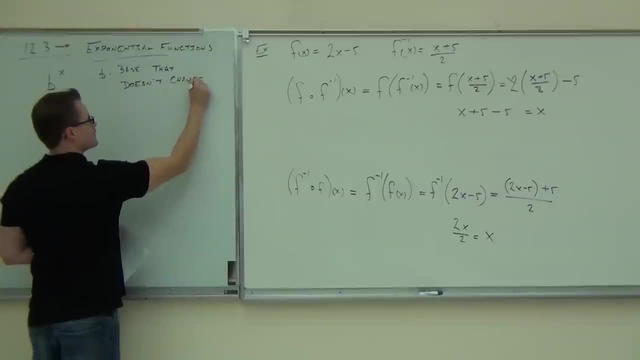 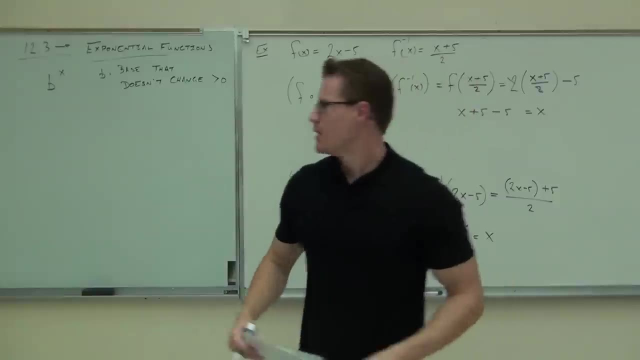 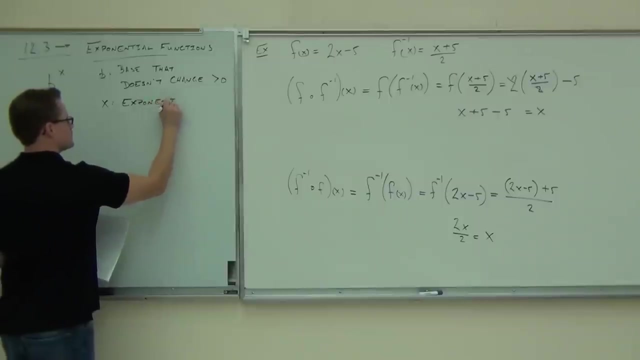 They don't get A, When are they gonna get A? It's only possible when their B is equal to A. Now why would everybody say that? Why is everybody answering A there instead of A? Also, it'll be greater than zero. Won't be negative. X, our variable, is actually our exponent, Which is με and cos. It's very interesting to me. Okay, We also have letter A and nota, So I don't read it again for other people, but I'm pretty sure I wrote the part without that in my herramient is a duty of mine. 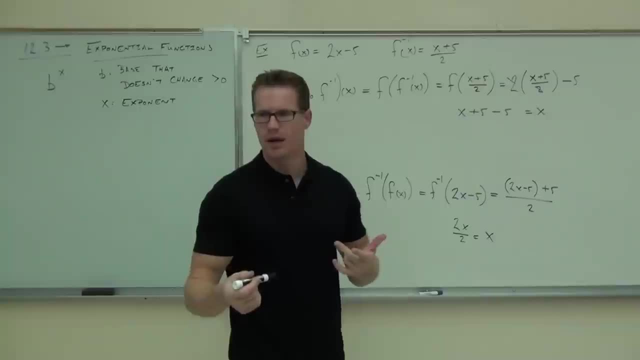 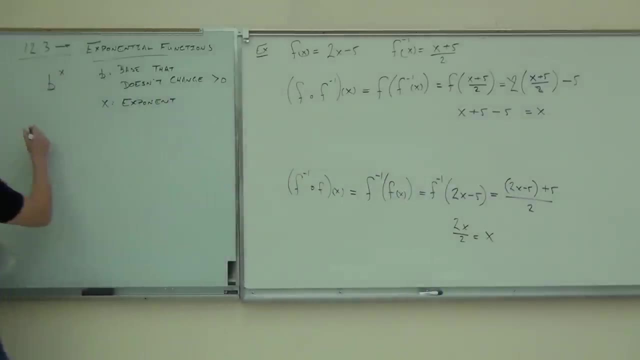 number. we now have a number raised to a variable. That's a weird idea, right? We've got this number raised to something that's changing, So an exponential function is going to look like this for us. We're going to have: f of x equals b to the x. 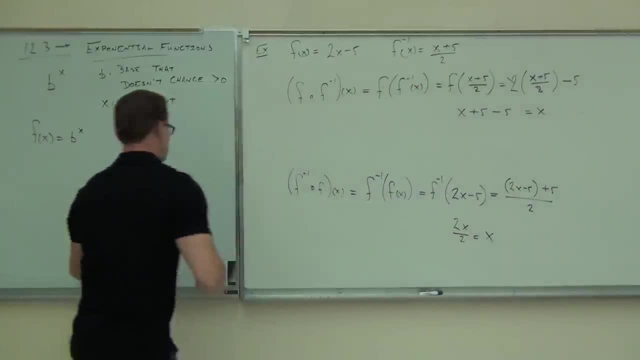 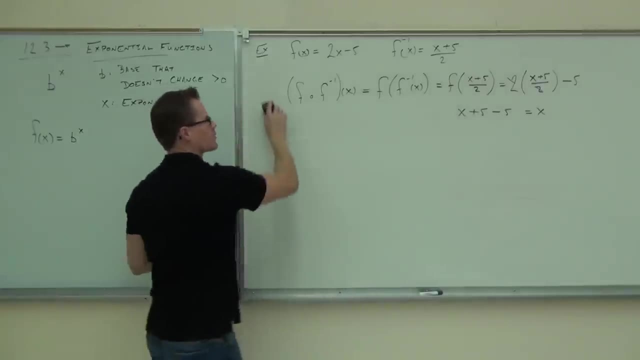 Now I would like to show you a couple graphs to see the difference between these things. I'll put them up on this side of the board so we can see the difference between them. We're going to find out how exponentials actually look graphically. 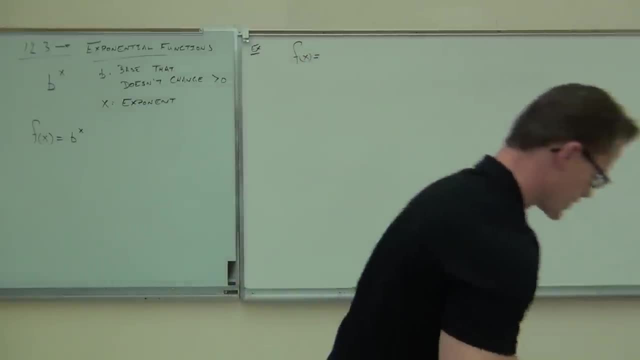 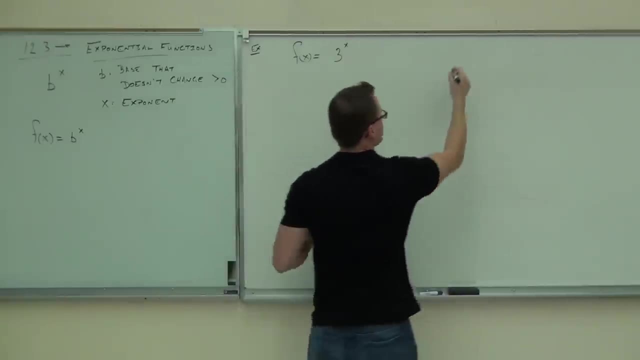 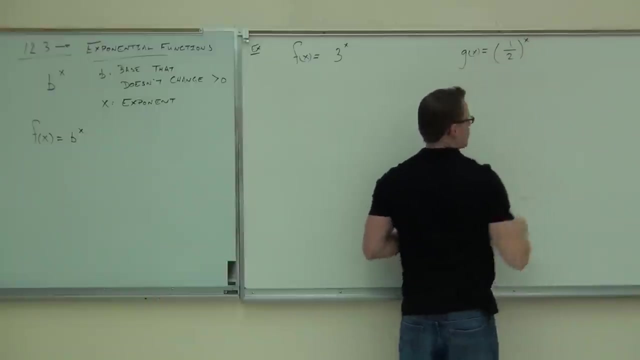 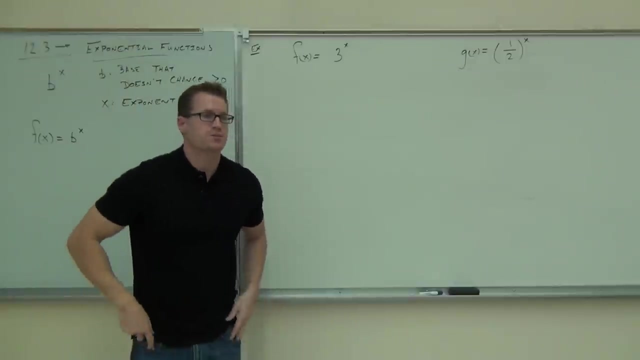 So I want to graph two functions. We're going to do them on two sets of axes, so we can see the difference here: 3 to the x and 1 half to the x. Hey, first things first. can you identify that these two functions are in fact exponentials? 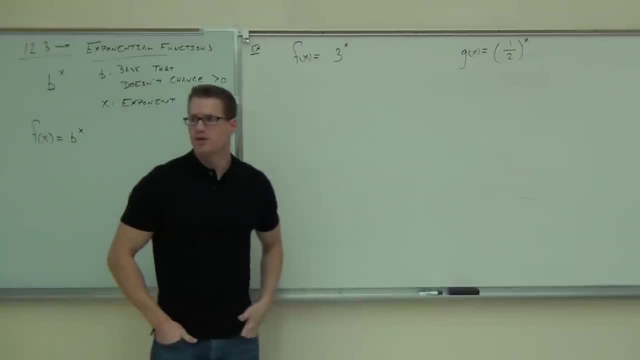 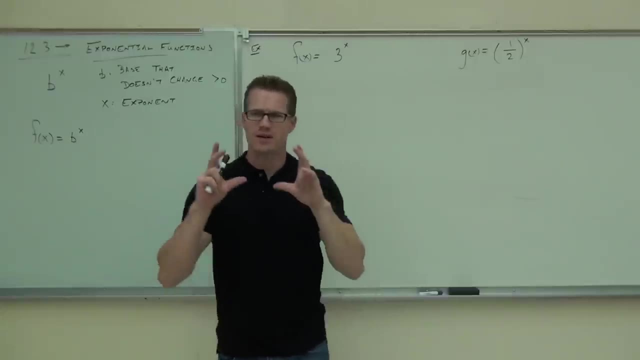 Yes. What's your base here? 3. Good, What's your exponent? x, That means exponential, It's a variable. The other one: what's your base? 1, half Good To the x. You'd have to have that fraction in parentheses saying: 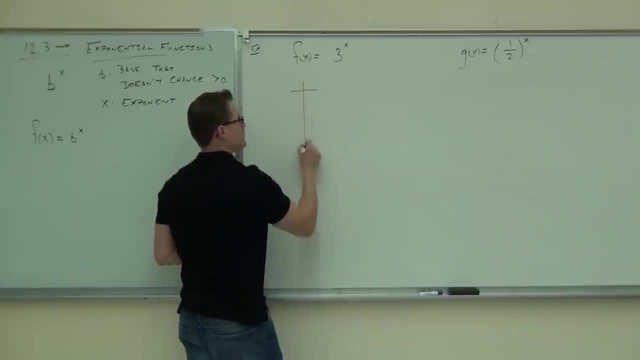 the whole thing's being raised to the x power. Now we're going to make these with a table because we have no other way to do it. right now, We don't know what these look like. Okay, So x, g of x. 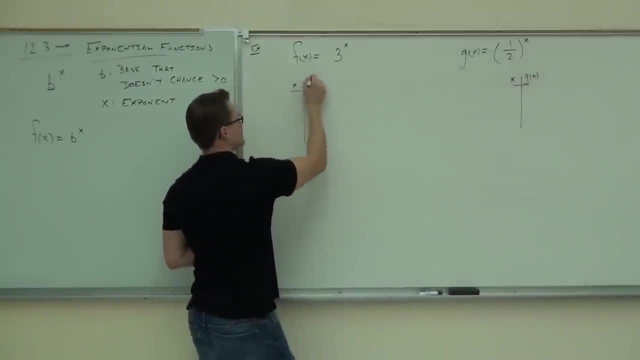 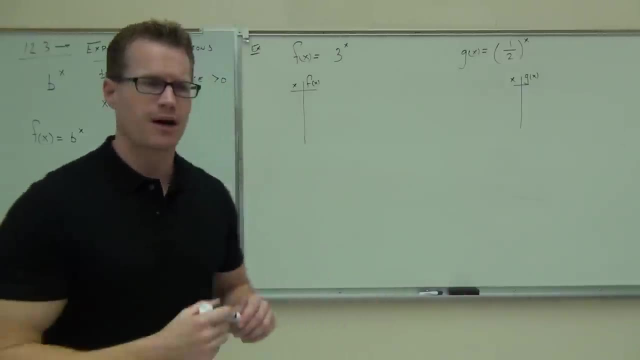 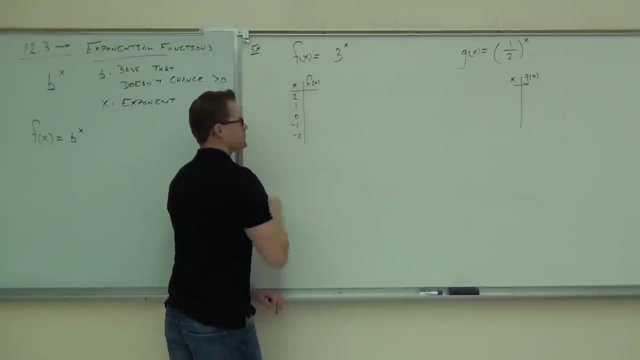 x, f of x. Now, typically we'll pick five numbers. Pick five numbers on each of our graphs. So let's pick. We'll start at the positive side first, so it'll be easier. 2, 1, 0, negative 1, negative 2.. 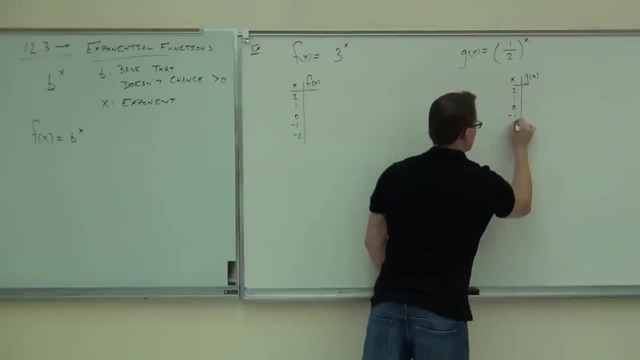 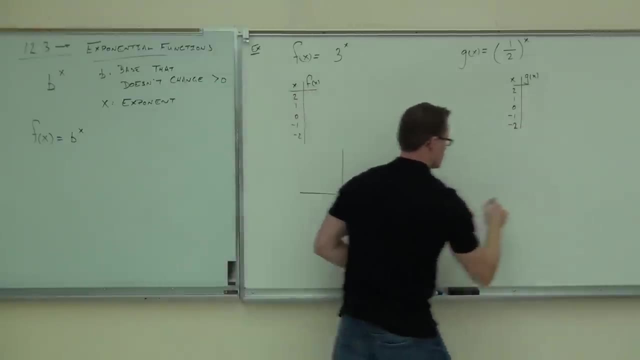 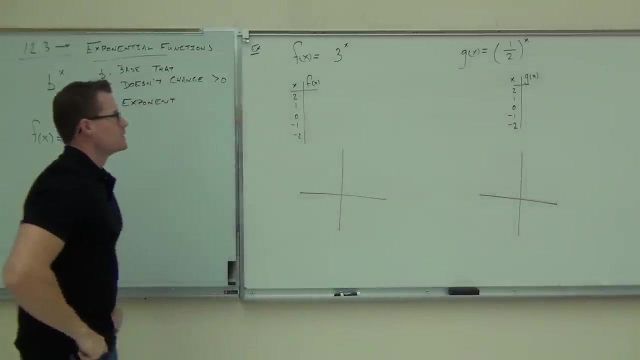 And the same thing over here: 2, 1, 0, negative, 1, negative, 2.. Oops, that's not a 2.. Now help me out with this. If I say my variable takes the value of 2,, 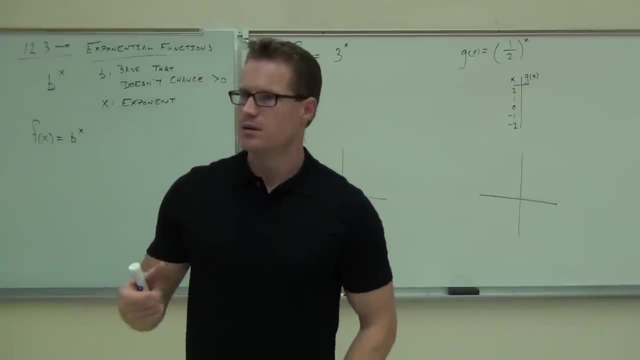 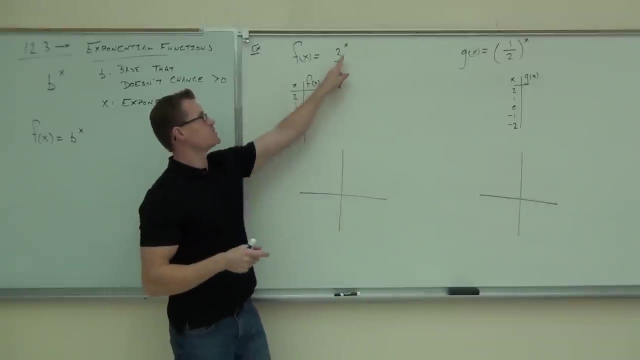 what's that mean for my function? How can you represent that? So I plug in 2.. What are you going to do? It's going to be squared. How much is it going to be if I plug in 2 here? It's going to be 9.. 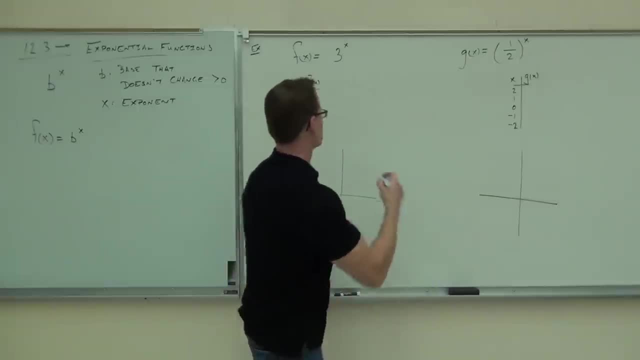 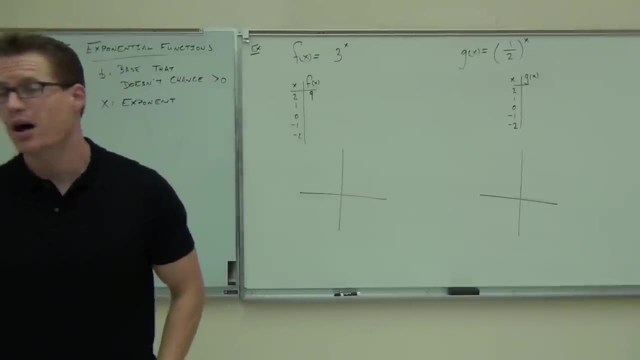 2 squared is 9.. You follow that? Yeah, 2 squared would be 9. 9.. How about 1?? If I plug in 1,, how much am I going to get? That would be 3 to the first power. 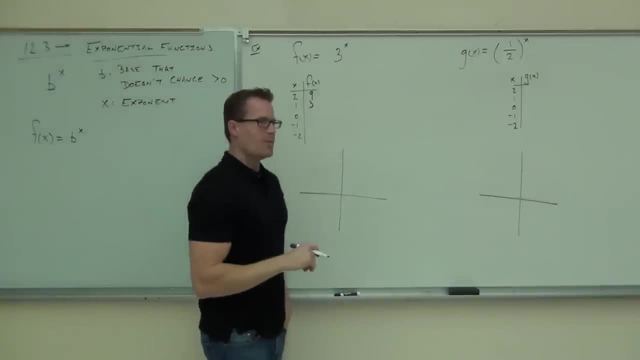 How much is that? How about 0?? If I plug in 0,, what's 3 to the 0? 1. Yeah, don't tell me 0, right, It's not, It's 3 to the 0.. 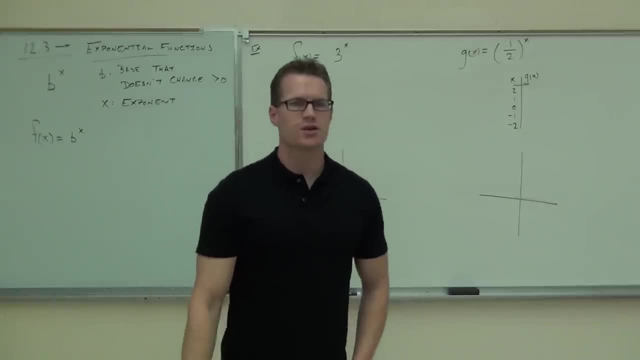 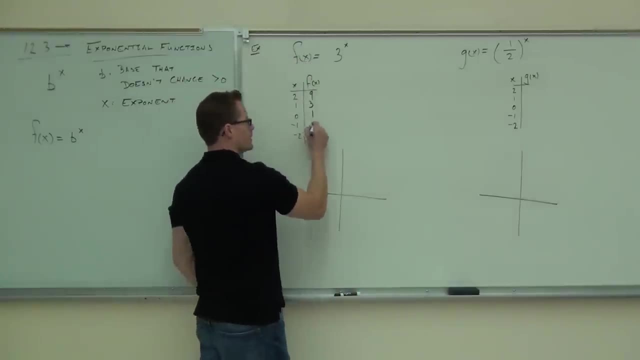 Anything to the 0 power gives you 1.. That's interesting, right there. Now, here's the cool ones. Ready for the cool ones: Negative 1. If I plug in negative 1. I'm going to actually do the work here for you. 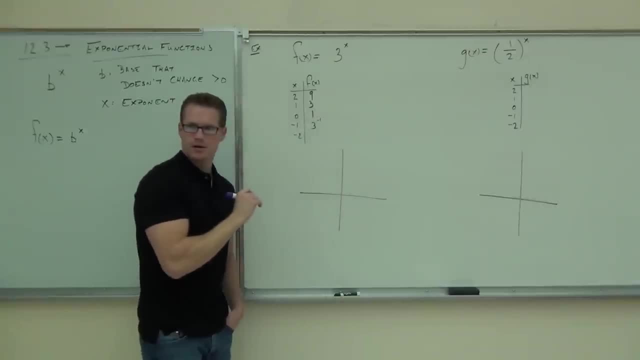 If I plug in negative 1, that's 3 to the negative 1.. Do you follow that? 3 to the negative 1 doesn't mean negative 3.. It actually means 1 over 3.. With me there, That's weird, right. 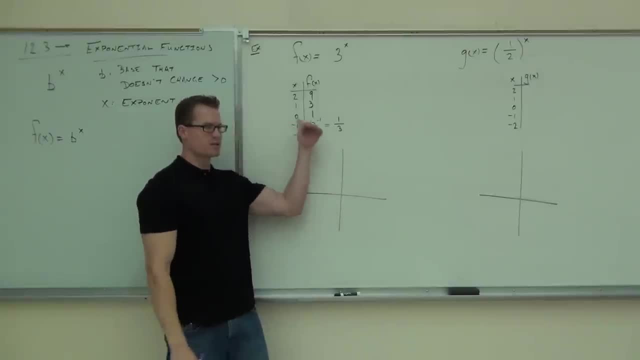 Is it negative? So does a negative number being plugged in actually give you a negative answer? No, That's strange. That's kind of cool, That's weird. Actually, here's what this is going to do for you. Check it out. 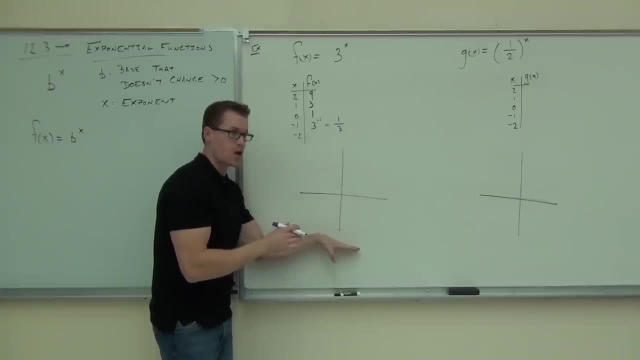 Is this graph ever going to be negative? No, Not, unless you have a negative in front of that. Then it would. It would be reflected, But no, And negative 2 would be 3 to the negative 2.. That's going to be 1. ninth. 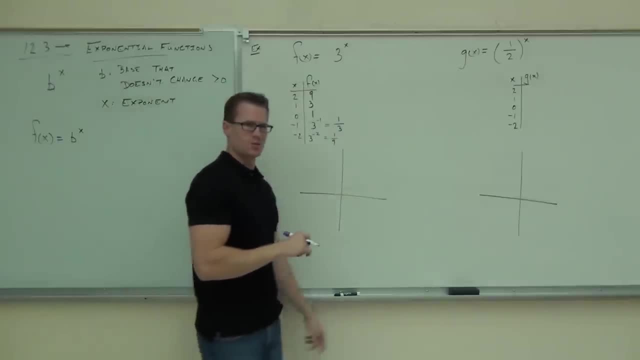 It should be a relationship. Look at 2, 9.. Negative 2, 1. ninth, That's cool, That's kind of interesting. If you plot these points, notice that I do have points. I plug this in. I got. let's see 1, 2, and 1, negative 2.. 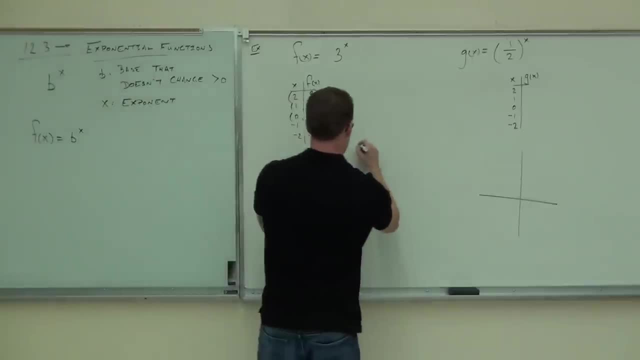 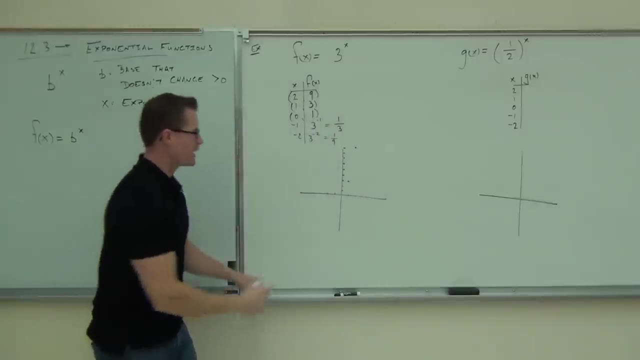 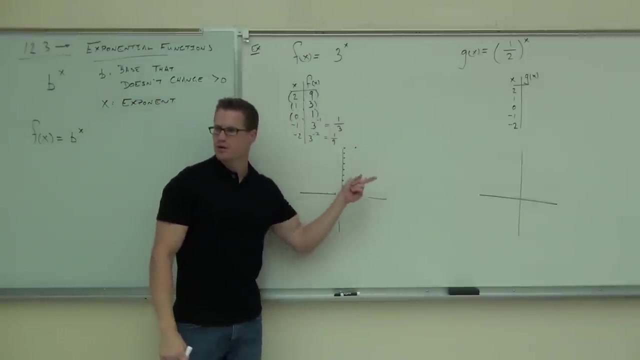 If I plug in 2, I got out 9.. If I plugged in 1, I got out 3.. If I plug in 0, I got out 1.. Are you okay with these three points? folks Nod your head if you are. 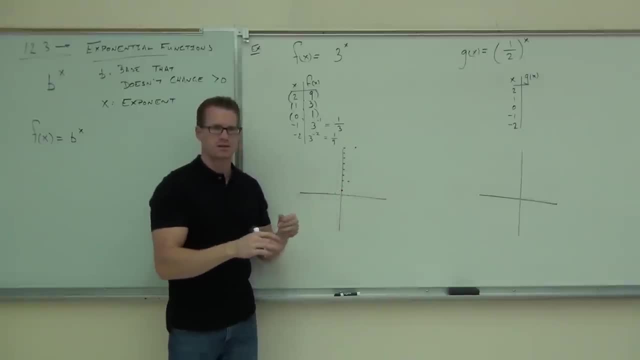 Are you okay with that? I'm not getting a whole lot of head nods. It's either yes. well, I mean I did that backwards. It's either yes or no. It's either yes or no. Are we yes or no? 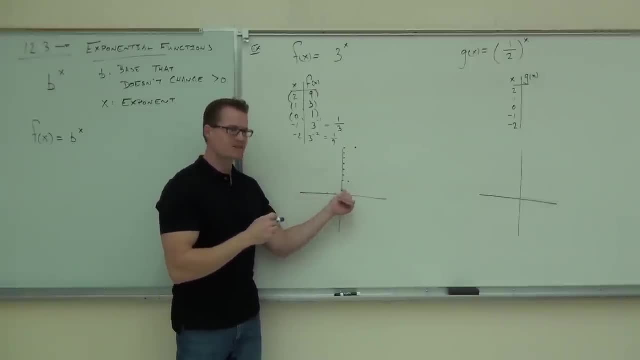 Yes, Okay. so these are just our points here, This side of the graph. do you see what it's doing? Is it straight? No, No, it's going. In fact, if you plug in 3, plug in 3, what's 3? to the third. 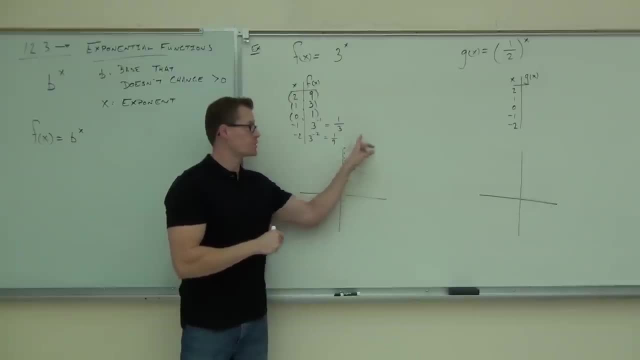 27.. You know we're going to get 27.. Plug in 4, what's 3 to the fourth, 3 to the fourth, 3 times 3 times 3 times 3 is 81.. 81.. 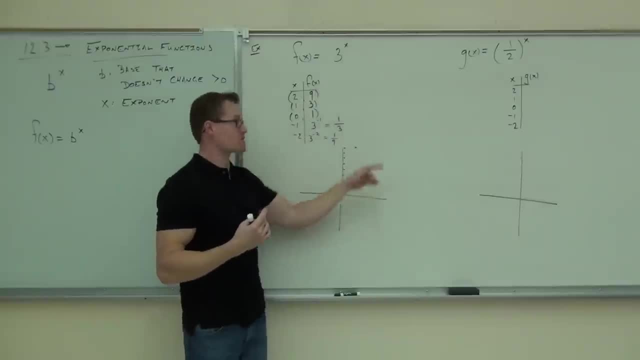 If you plug in the number 4, you're going to be at 81 already. That's off the charts. That's way up there. That's way up there. Are you seeing what it's doing? It's growing so fast. 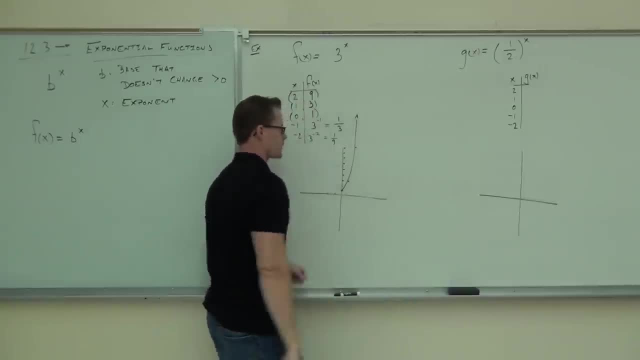 This side of the graph looks like this Way up there, really really fast, Faster than a quadratic. Quadratic is always a power 2, right, But this one is saying you're taking a number, you're increasing the power. 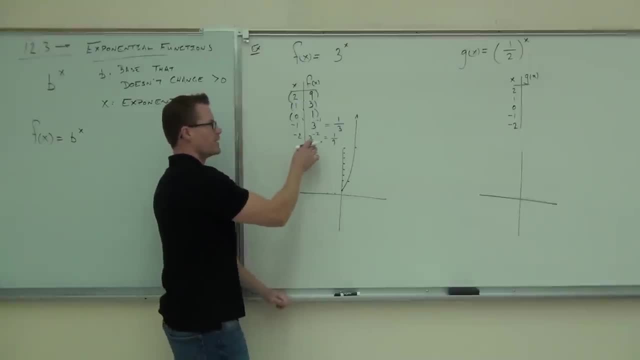 Man, that's growing fast. That's really fast. Now on the other side, though, check it out. Can you plot negative 1 comma 1 third? What's negative 1?? 1 third is up or down, Up. 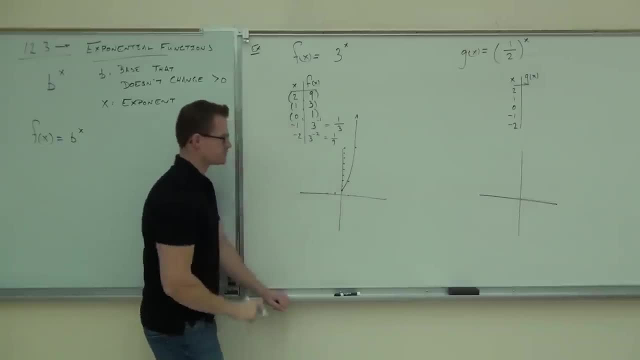 Up, but just a little bit. That's like: right there, That's 1 third, You with me, Negative 2, we got 1 ninth. That's almost on the x-axis. Now let me ask you a series of critical thinking questions. 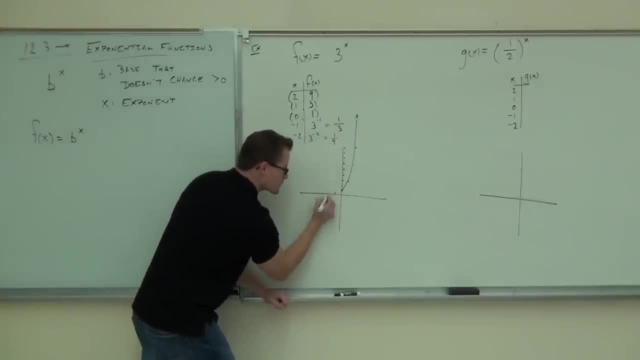 Firstly again, are you ever going to have something below the x-axis? No, No, not unless there's a negative in front of it. Second one: is this ever going to touch the x-axis? No, No, No, No. 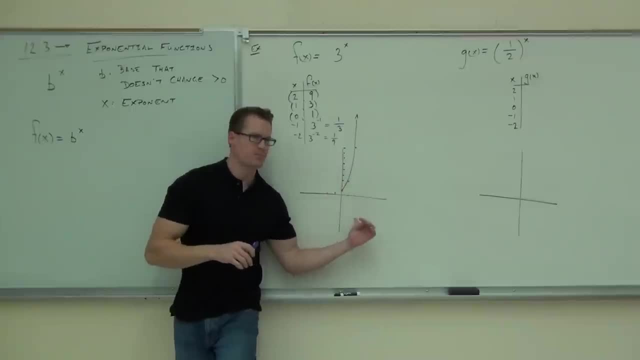 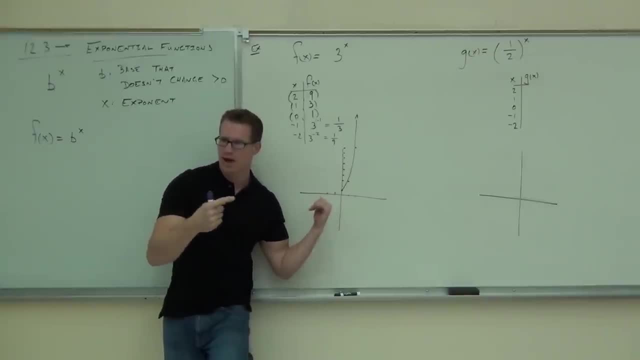 Four is going to be 1 over 81.. 5 is going to be 1, I don't even know anymore. but you take 3 to the 5th, put a 1 over that. It's going to be really, really, really close. 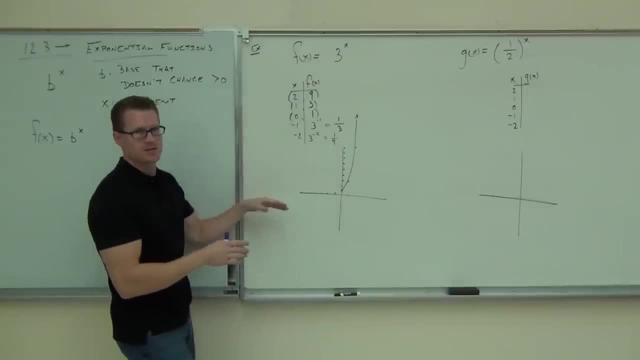 But it's never going to touch it. This is called being asymptotic to the x-axis. It has an asymptote here: It's never going to. it's going to get really close, but never touch it. This side looks like this: 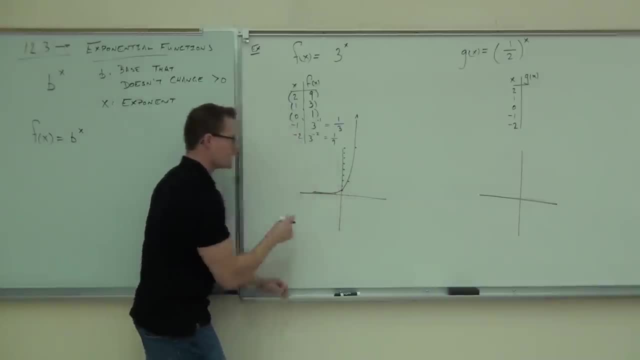 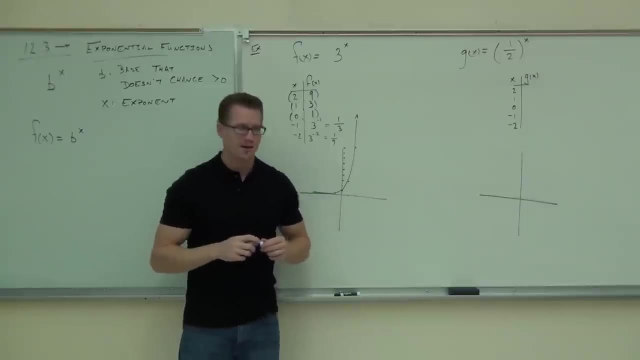 It doesn't go back up. That's a mistake. It keeps going along. The x-axis is getting really, really, really close. Come on close to it. Here's the sound effect for a exponential function. It goes: My upper register is a little gone on that one. Try one more time. It's so dry, Do you? 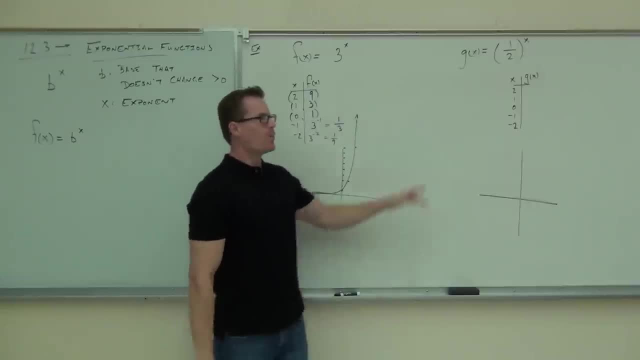 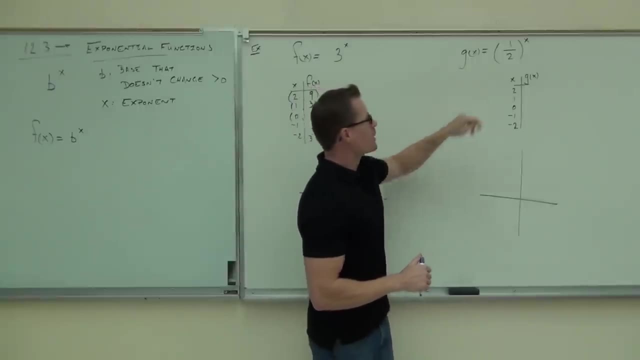 hear it. It goes up like that. I want to see what the fraction does and then we'll call it a day. We'll be out of here. Remember that clock's a little bit fast. So if I plug in one half, check it out. Two to the one half gives you that would be one half squared. 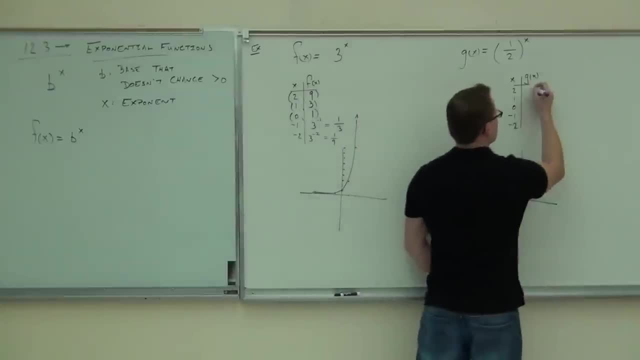 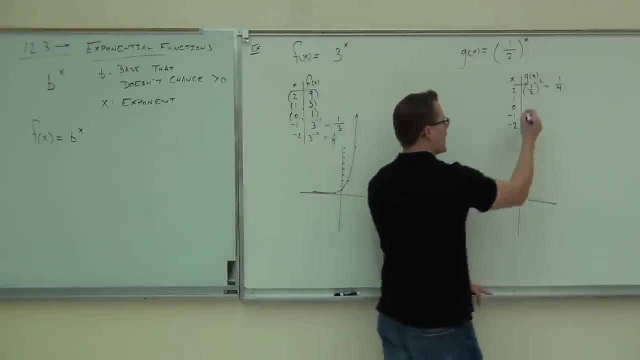 I did that backwards. I said it backwards. One half to the second, One half to the second power is going to give you one fourth. Do you see how we're getting one fourth out of that? One half to the first power. well, anything to the first power just gives you that back. 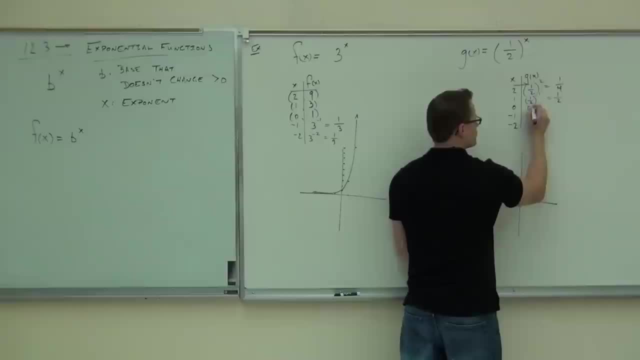 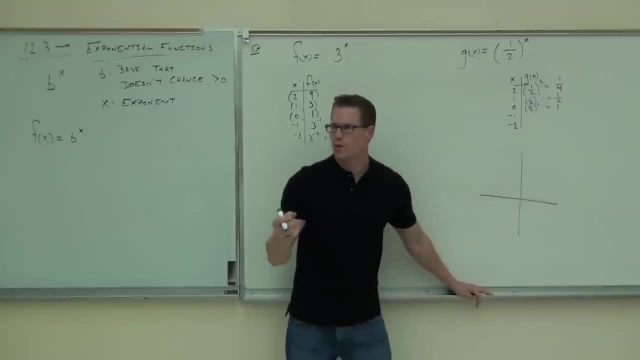 again. How about zero to the one half, to the zero power: One, one, One one. Yeah, Oh, that's weird. We're going to get zero comma one again. Can you imagine this for every exponential? If you have an exponential up here to the zero, you're always going to. 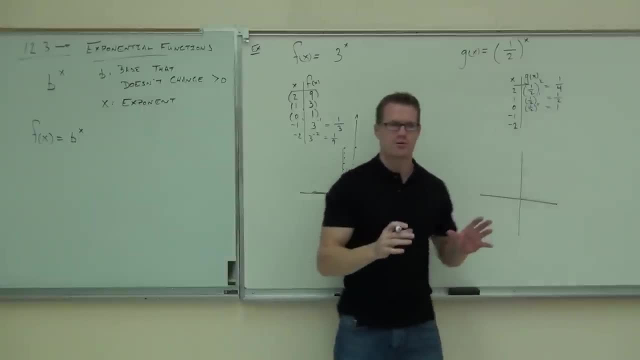 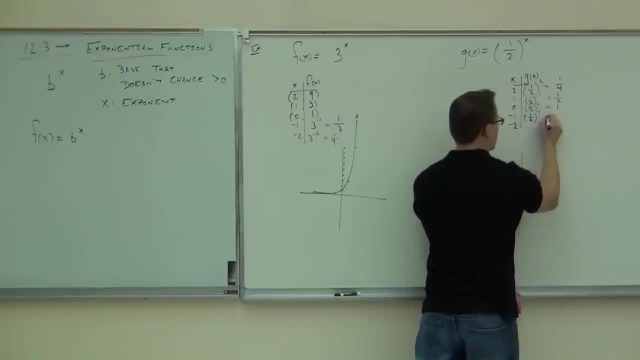 get out one right, So zero. one should be on every one of our graphs, unless we shift it around. We'll talk about shifting later Now. negative one, that's one half to the negative one: power. Here's what this does. Watch carefully. 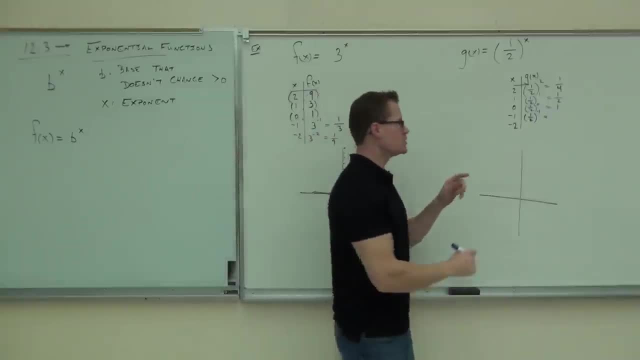 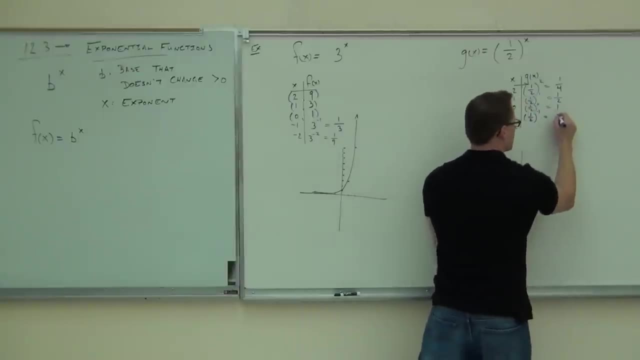 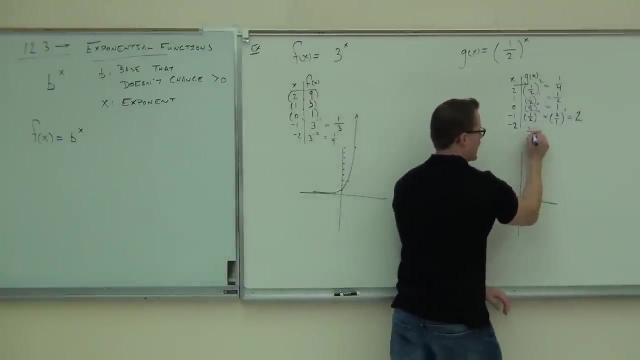 If you have a fraction to a negative power, what you do is you can flip that fraction reciprocated and it changes the sign of that power. So we would have two over one to the first or the number two. Same thing would happen here: One half to the negative. 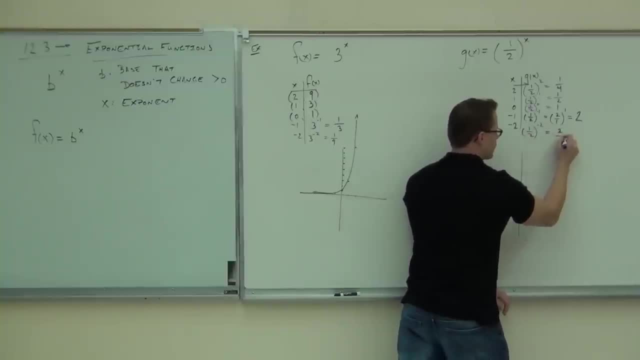 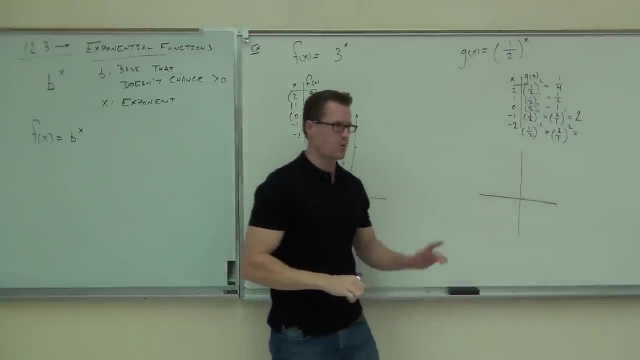 two: you're going to get two over one squared. You flip your fraction, it changes the sign of the exponent. That's the exponent rule that we covered a while back. How much is that going to be? Four? You see the same relationship right. One, fourth, four. 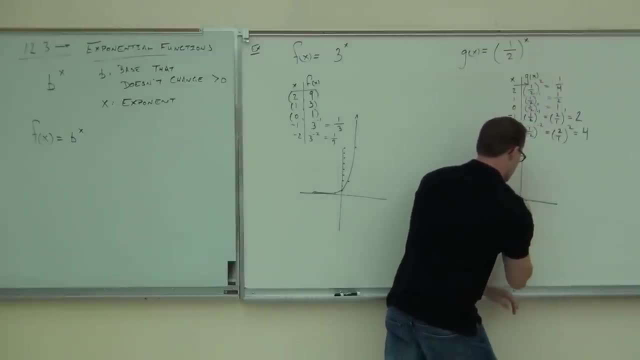 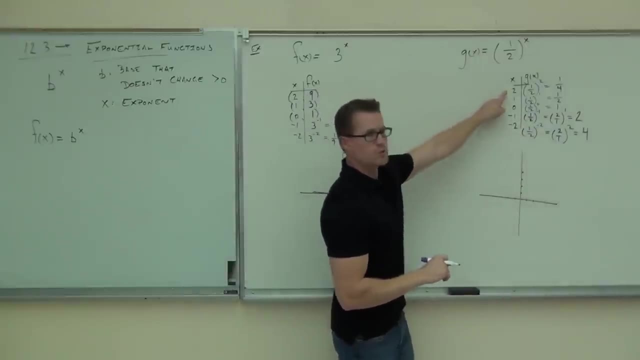 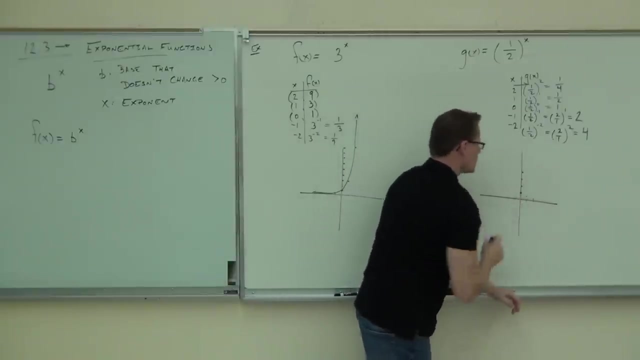 We'll graph it real quick. If I go over to two, two gives me one fourth. That's right there. If I go to one, it's giving me one half. That's slightly higher. If I go to zero, it's giving me one. That's here. If I go to negative, one. check this out on the board. 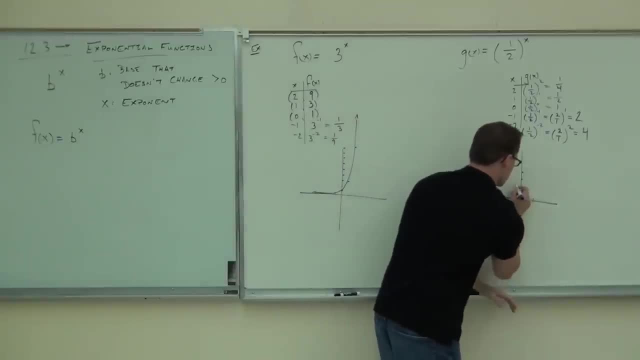 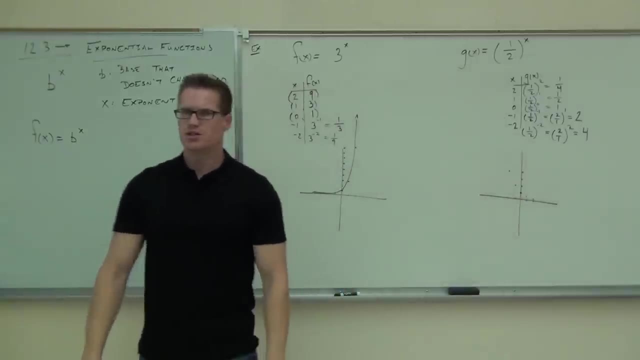 if I go to negative one, I'm getting two, And if I go to negative two, I'm getting four. Are you all okay with those points? Do you see what this is doing? Do you see what it's doing? Is it going in the same direction? 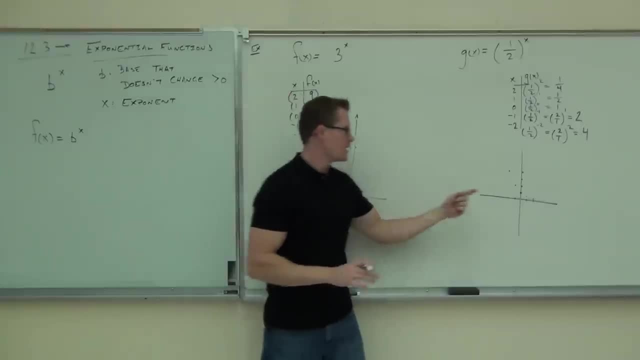 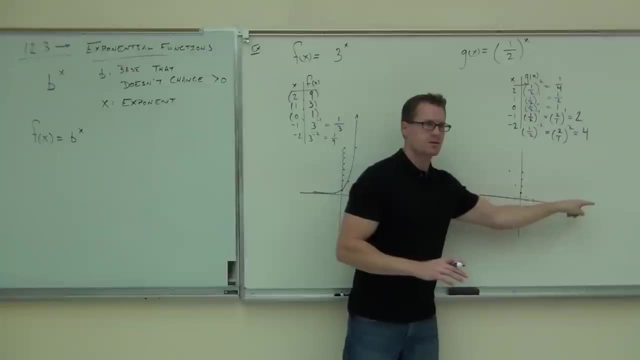 as this. Yeah, that's true. So a couple questions, two more questions. Is it ever going to be below here? No, No, No. Is it ever going to touch the x-axis? No, This looks almost the opposite of this. It's almost like a reflection. 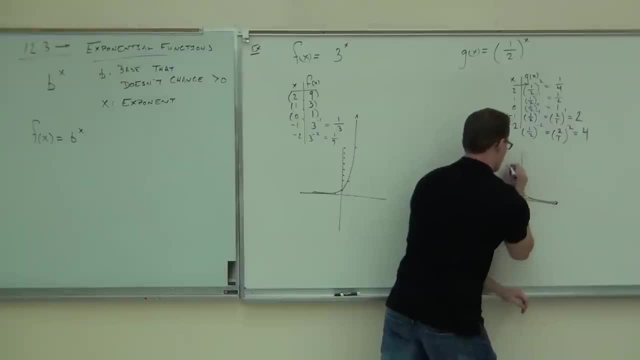 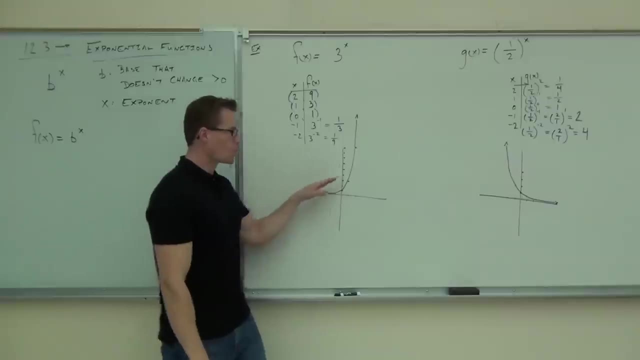 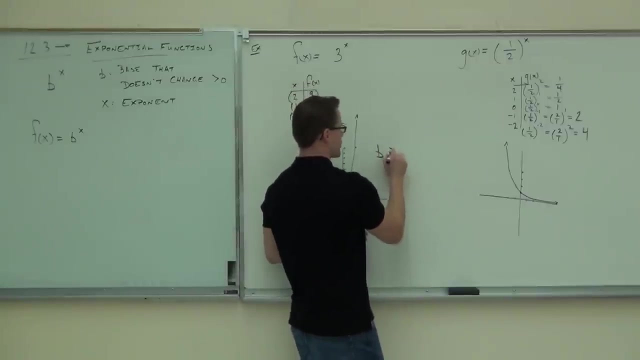 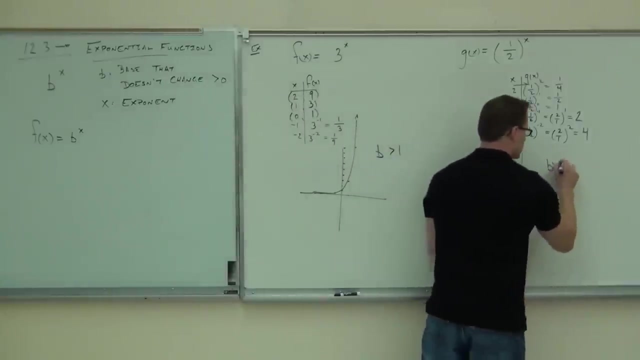 Different number, Different number, Different number. That's it, That's our exponentials. This one goes. That's the idea of these exponentials: If B, if our base is greater than one, if our base is greater than one, we'll have this: It will climb If our base is less than one. 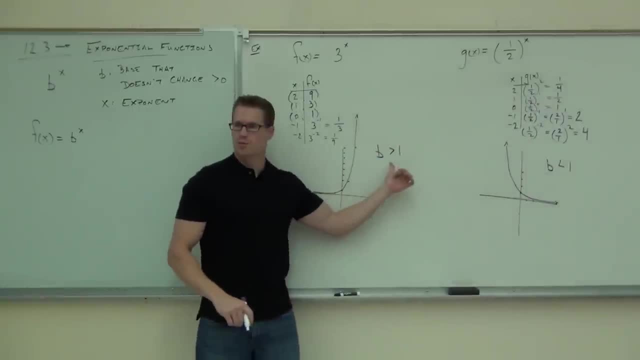 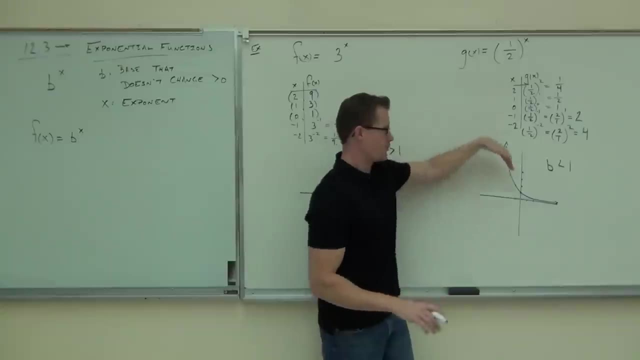 it will fall So whole numbers or fractions greater than one. it's going to look like this every time: Fractions less than 1. They'll never be less than 0. It's never negative. It'll fall like that. How many of you want to set these ideas of our graphs here? 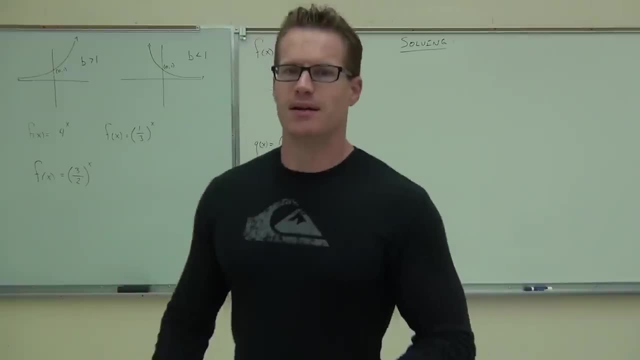 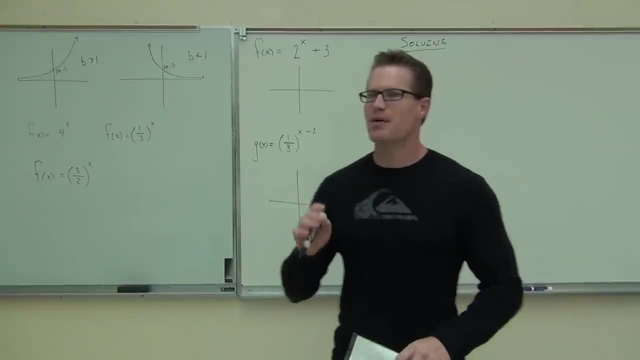 Good, okay, So last time is that let's get this over with, All right, I'm just kidding. Last time we were talking about functions, Specifically, we talked about inverse functions. That's what you did your homework on. 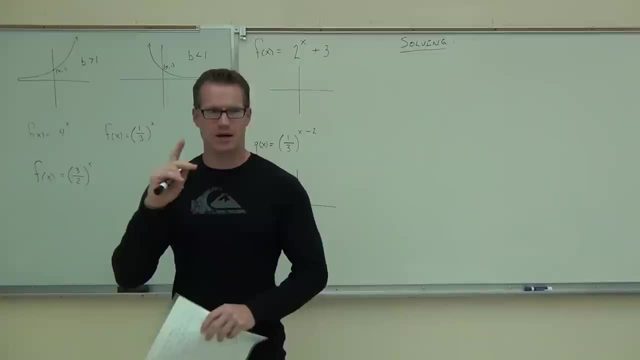 Did you guys do okay on your homework? Yeah, Switching the x and y right. Remember how to do that, Because we're going to look at that in just a little bit. So now we talked about one specific function towards the end of our day. 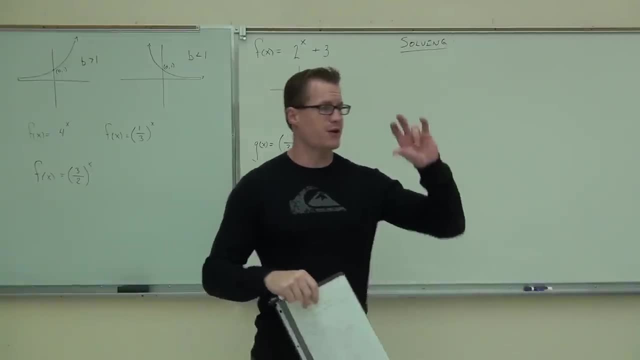 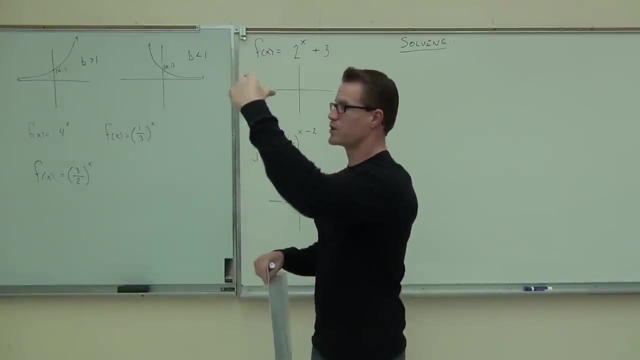 and that was exponential functions And the idea was, instead of having a variable to a number exponent, like x to the second, x to the third, we now have a number which is a base raised to a variable which is our exponent, in this case. 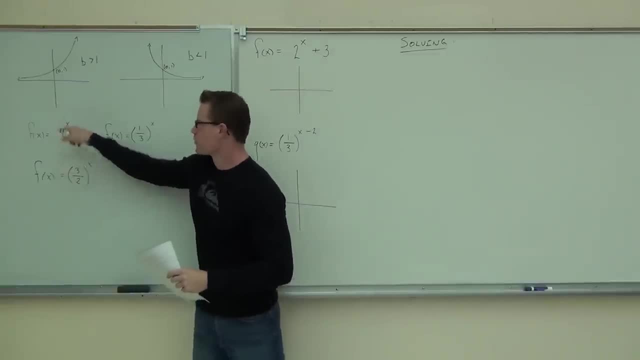 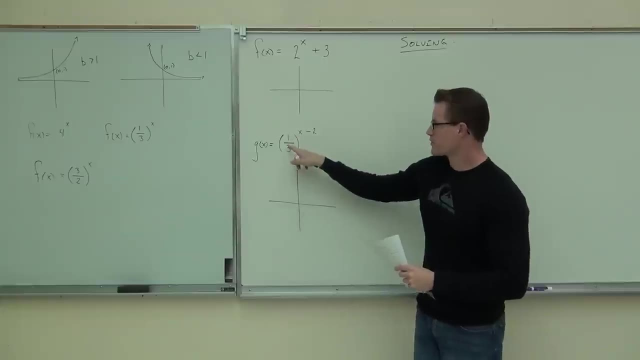 So we have these things as our exponential functions, Like 4 to the x, or 1 third to the x, or 3 halves to the x, or 2 to the x plus 3, or 1 third to the x minus 2.. 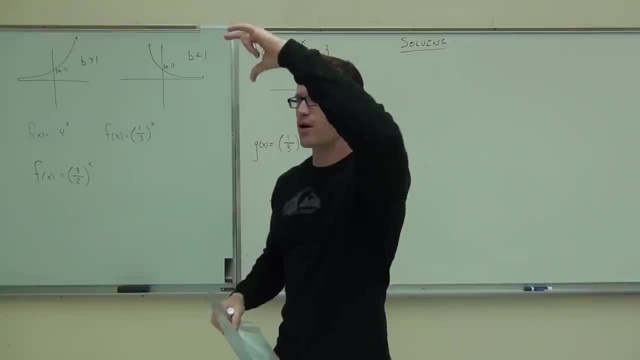 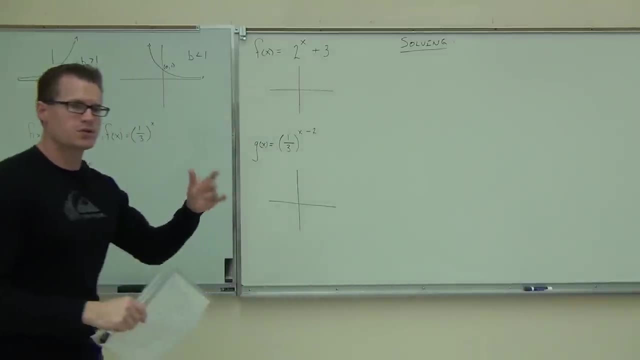 The whole thing. The whole thing. Those are all exponentials, because we have a number base and then our exponent actually has a variable in it, And that's interesting. Now we did talk about two things. We either have one of two shapes of graphs for our exponentials. 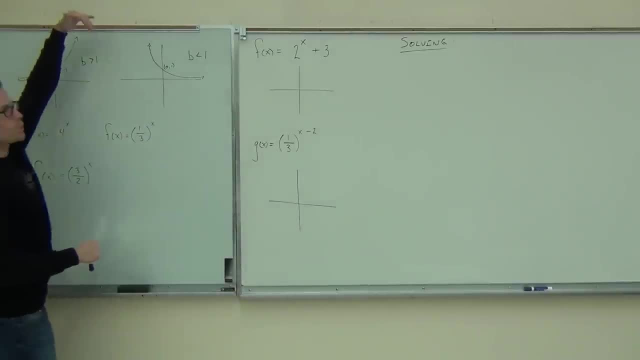 It either goes or. do you remember talking about that last time? It's one of these sweeping curves that grows really quickly or declines really quickly and then flattens out. That's our two types of exponentials. I need you to be able to tell me which one of these 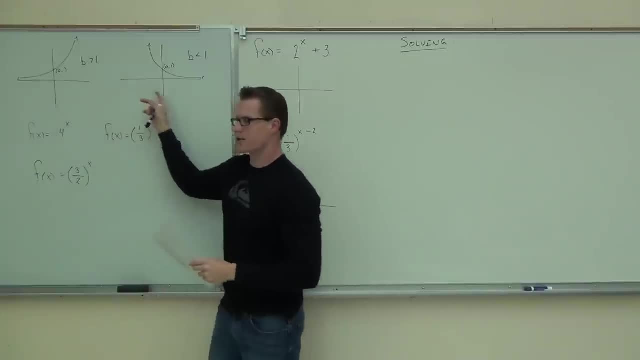 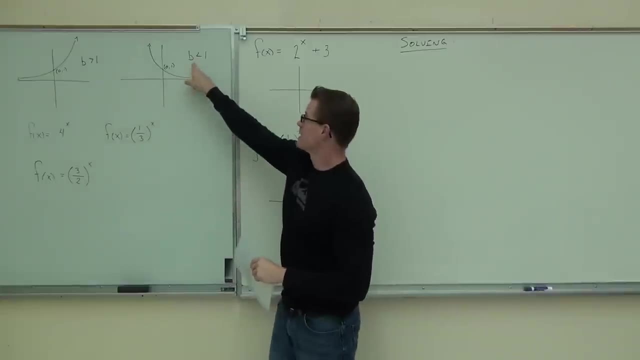 each of these would look most like. Now, of course, this is just kind of a generic thing saying: if our base, which is our b, is greater than 1, we've got this basic shape. If our base is less than 1, we have this basic shape. 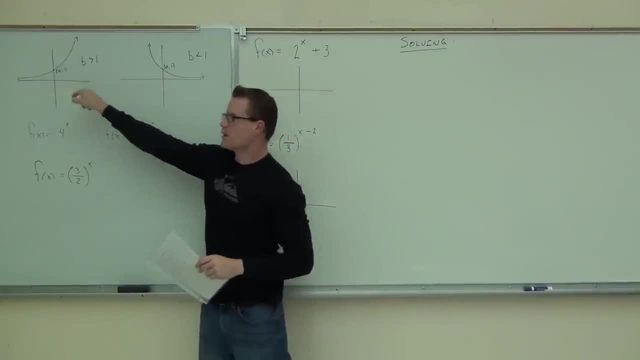 Notice how, in each case, we go to the point 0, 1, and we go to the point 0, 1.. Do you remember why that is? Do you remember why that is? Or, in other words, let me remind you of this. 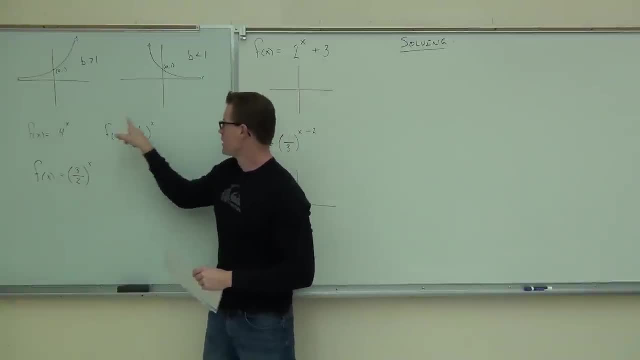 What would happen if I plugged in, if I plugged in 0 here and here and here? In every case, what am I going to get? 1.. What's anything to the 0 power, folks, 1.. That's why we're always going to get the point 0,, 1, unless we shift these around. 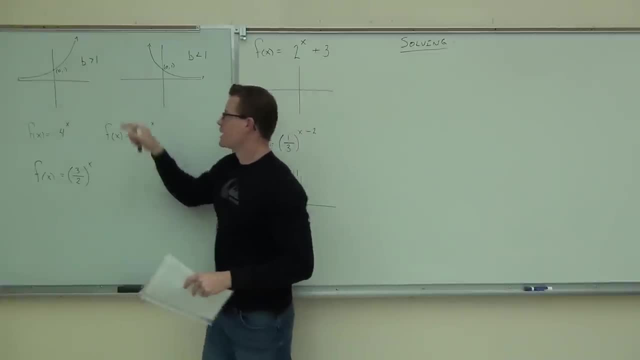 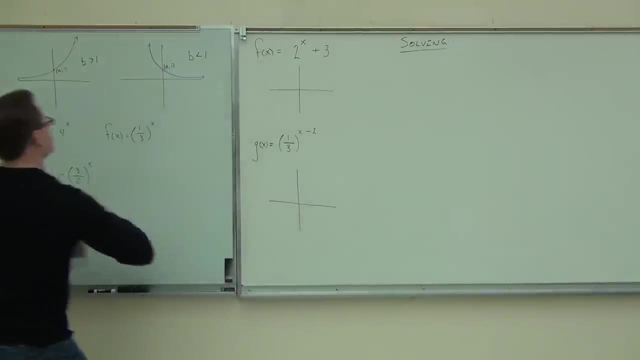 Are you with me on that? It's always going to go through 0, 1.. That's why we have that point and that point. Now let's go ahead and refresh your memory on this. Let's call this graph number 1 and graph number 2.. 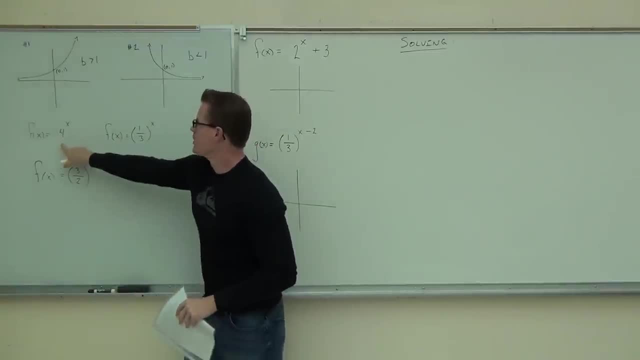 Can you tell me, ladies and gentlemen, what graph does this one look most like? 1 or 2? 1. Why 1? Great, Why is it bigger than 1?? So this 4, that's saying: oh yeah, that's our base, right. 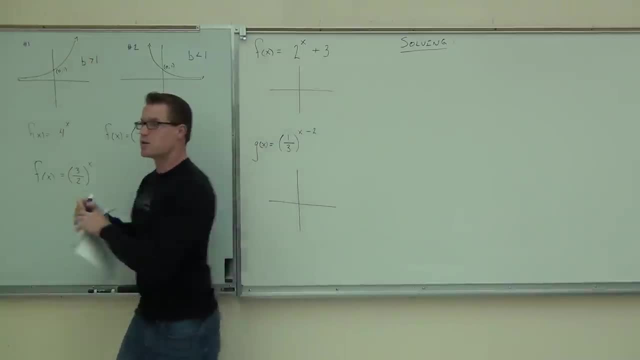 B is bigger than 1.. It's going to be climbing like that. This is most like graph number 1.. Now, if somebody else hasn't spoken yet today, how about this one? one-third to the x, One-third to the x. 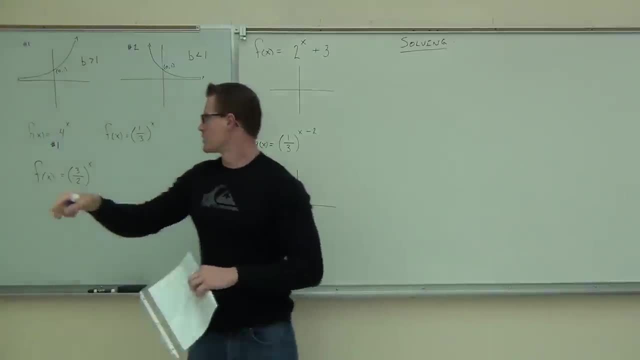 Is that most like graph number 1 or graph number 2 and y Number 2.. Number 2, y, It's less than 1.. Good, That's a fraction. It is a fraction, sure, but it's a fraction less than 1.. 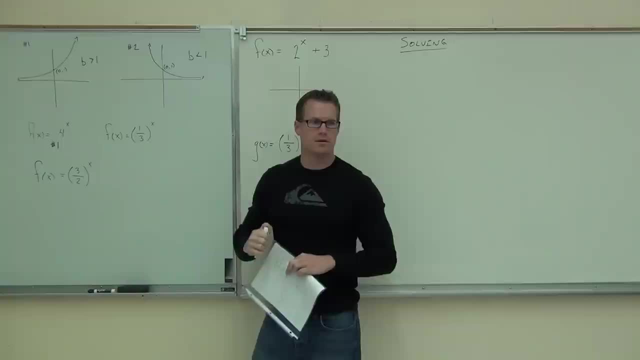 So this would most look like number 2.. It's going to go just like that. We need to make sure that it's less than 1.. It's going to go just like that. We need to make sure that it's less than 1.. 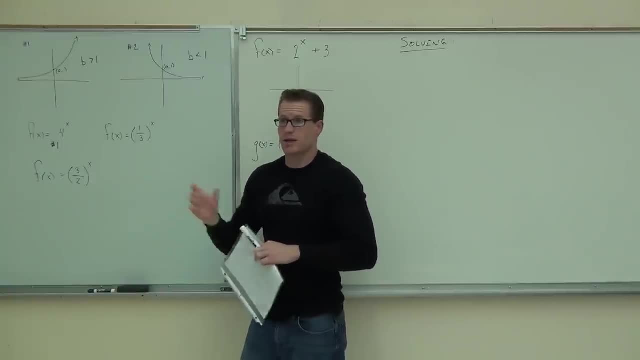 We need to make sure that it's less than 1.. Good, That's a fraction. It is a fraction, sure, but it's a fraction less than 1.. So this would most look like number 2.. It's going to go just like that. 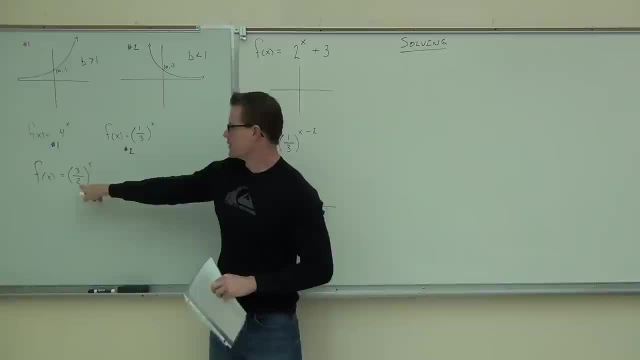 We studied y last time. How about this one? This one can be kind of tricky if you don't really understand why these work. Is this more like graph number 1 or number 2? Number 1.. Why not number 2?? 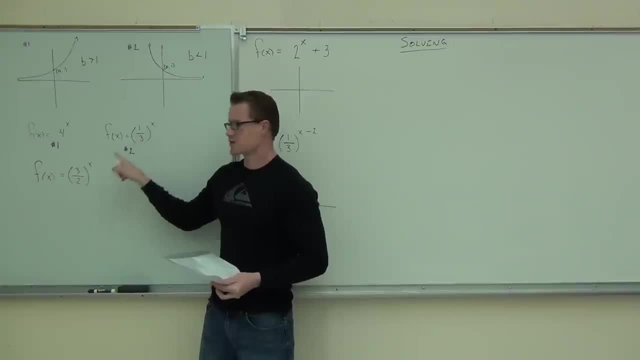 It's a fraction like number 2.. It's greater than 1.. Uh-huh, So this is like 1 and a half. This is 1 and a half raised to the x power, Not 1. Subfraction. 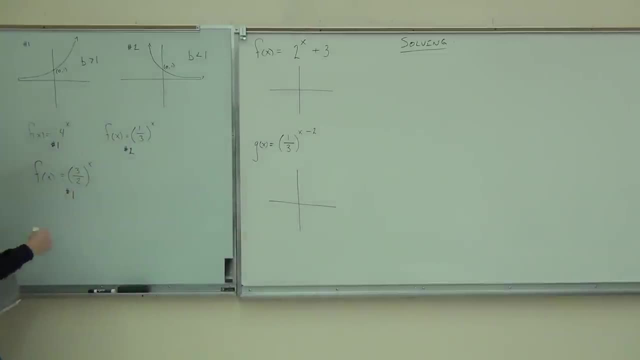 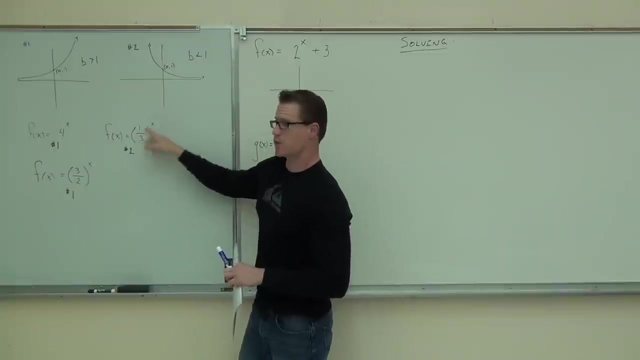 Less than 1.. This is mostly graph number 1. The larger the number, the more dramatically that will climb. The smaller the number, the bigger the denominator, in other words, the more dramatically this will fall. How many people feel okay with this so far? 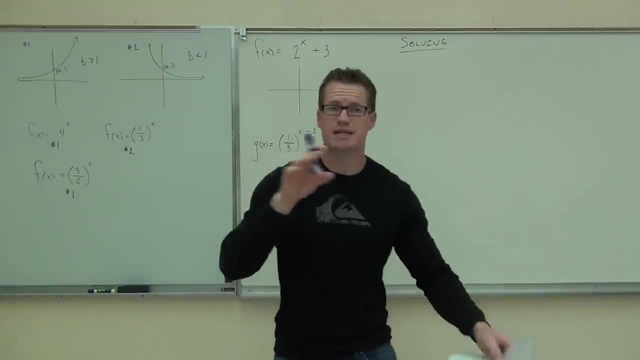 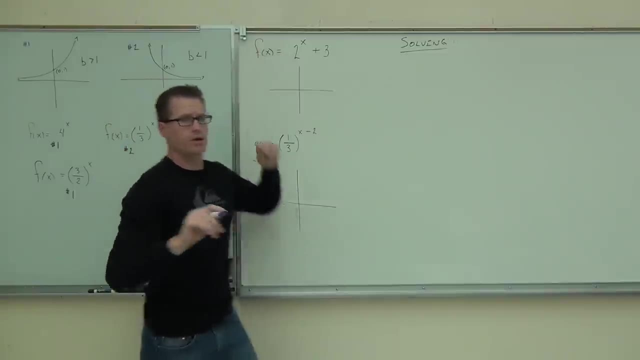 Okay, Now our last two. I want to show you that, just like we did in the last chapter and in chapter 8, we can shift these things around. Let's look at this one Again. is this more like graph number 1 or 2 from over here? 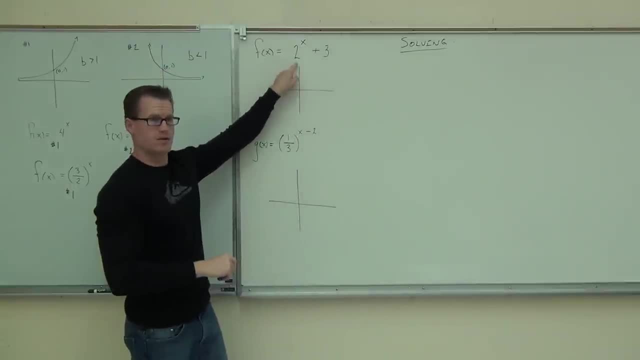 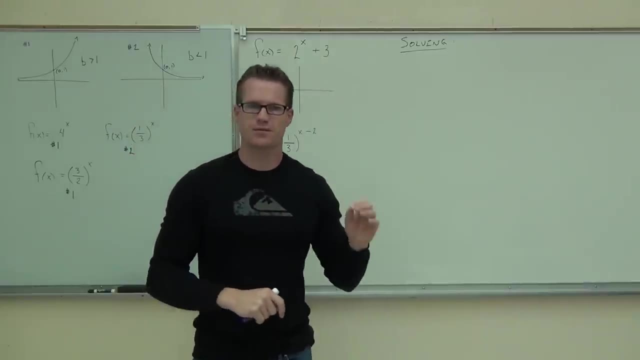 What do you think? Yeah, Definitely 1. Because that's greater than 1.. Are you following me Now? that plus 3 at the end of your graph, that plus 3 at the end of your function there, that should equate to some sort of shift. 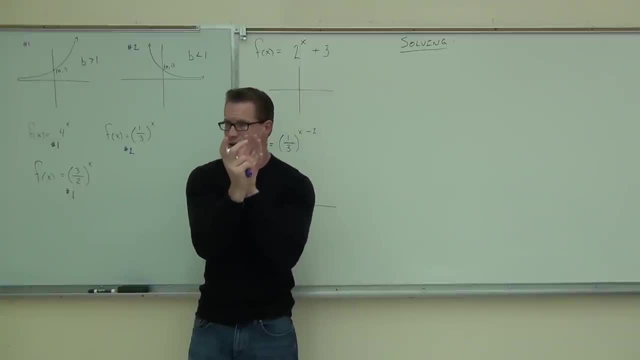 Do you notice how? it's not within the function, It's not connected to the x, It's not in the exponent, It's 2 to the x and then at the very end, you have that plus 3.. You guys see what I'm talking about. 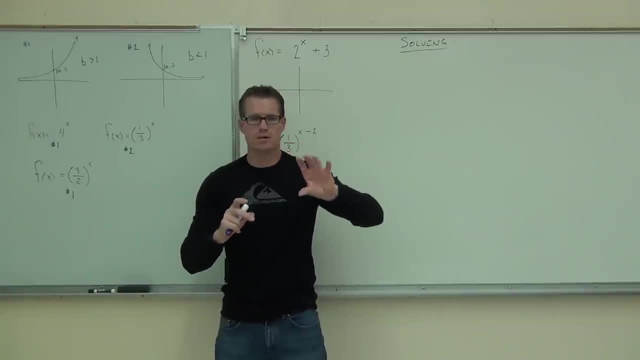 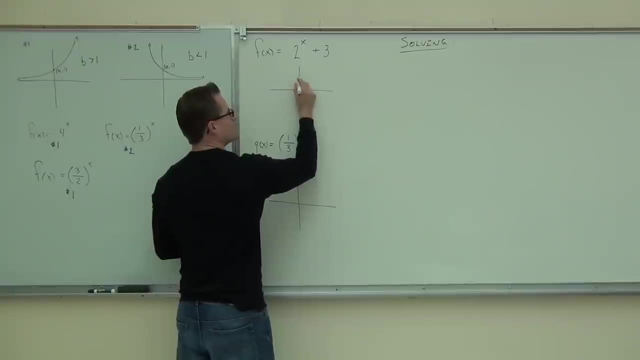 That plus 3, do you suppose that shifts it up, down, left or right? What do you think? Up, That's up, Just like you did with shift. Now here's how you do that. If you normally would cross here at this 0, 1, remember how they all cross at 0, 1?. 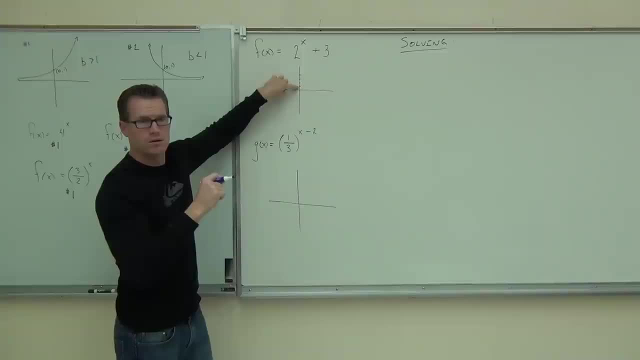 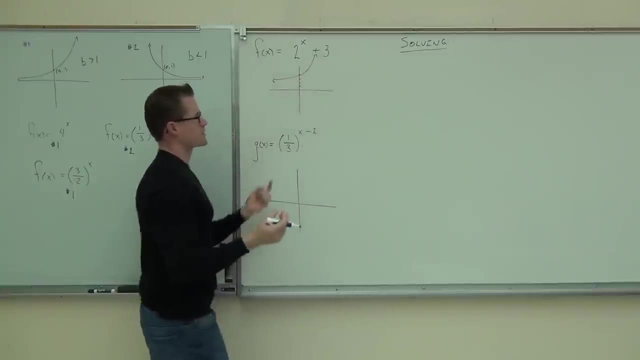 This is going to shift it up 3 spots. Where is it going to cross now? 0, 4.. 0, 4.. Yeah, It's going to cross right there. So we would shift our function up 3 spots because that would be a shift up. 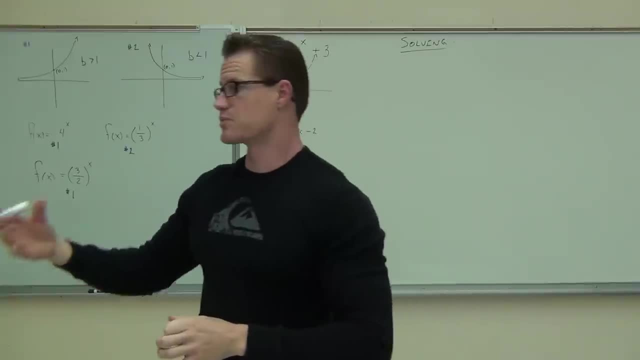 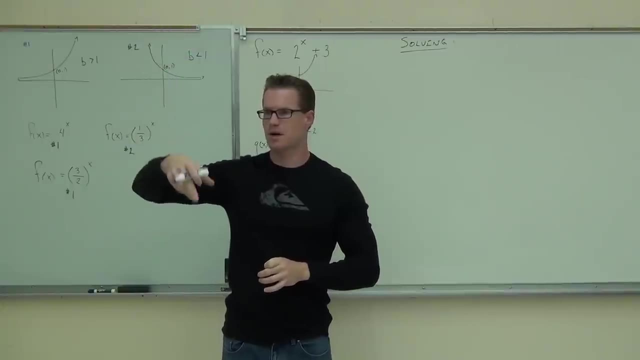 It's at the end of your function. That's a shift up or down, depending on whether it's plus or minus. How many people feel okay with that one? Yes, no. Do you remember the shifting, How we shift those parabolas up and down, left and right? 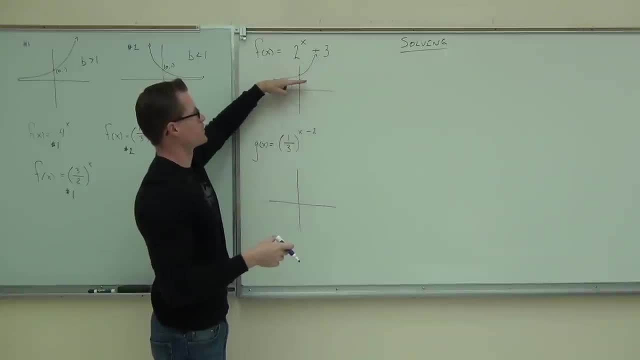 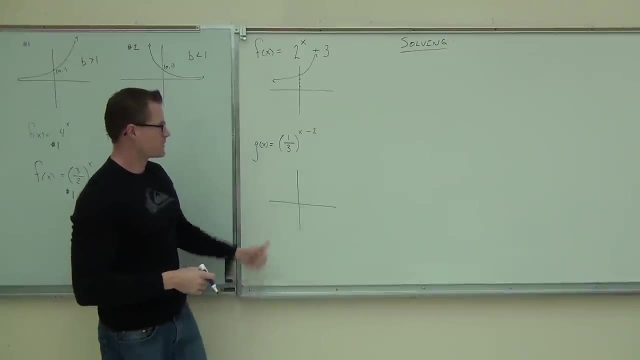 At the very end, that plus 3, that was the end of your function. We're shifting this up 3 spots. We're basically taking this one, shifting it up 3 units. Now the last one: this g of x equals one-third to the x minus 2.. 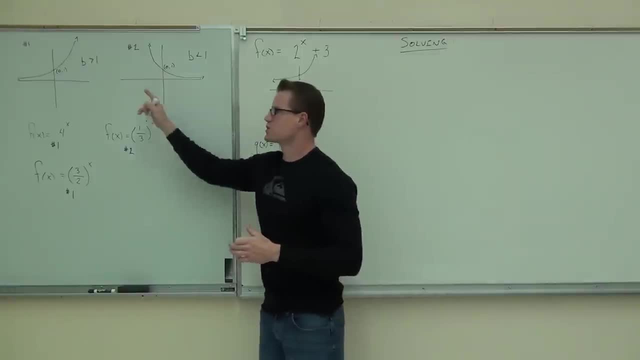 The first thing I need you to understand is which graph it's most like. Would you say this is most like graph number 1 or graph number 2?? Yeah, definitely 2.. Why is it most like graph number 2? Less than 1.. 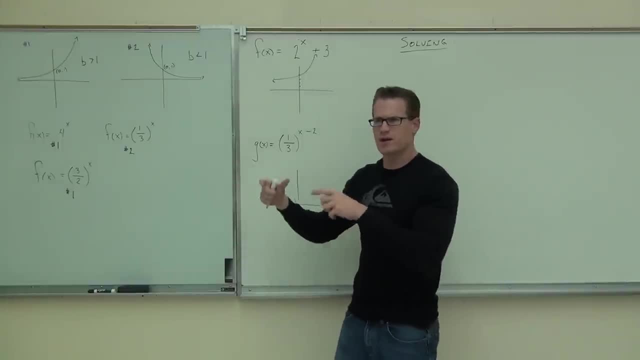 Okay, great, So you're identifying it. sounds like you're identifying the shapes pretty well. yes, So this is definitely like graph number 1, b is greater than 1.. Definitely like graph number 2, b is less than 1.. 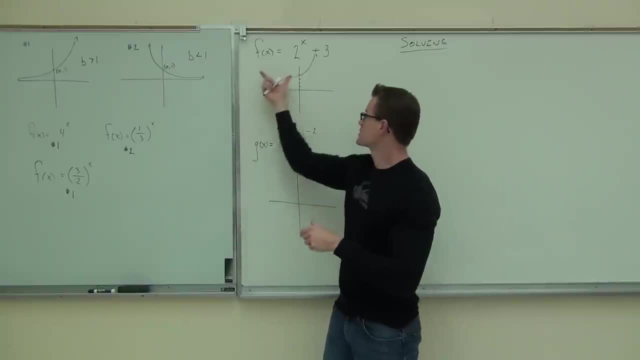 It's a fraction less than 1.. Now, this minus 2, does it look different than this plus 3?? Yes, This plus 3 wasn't attached to the exponent, was it? No, It wasn't within the function. 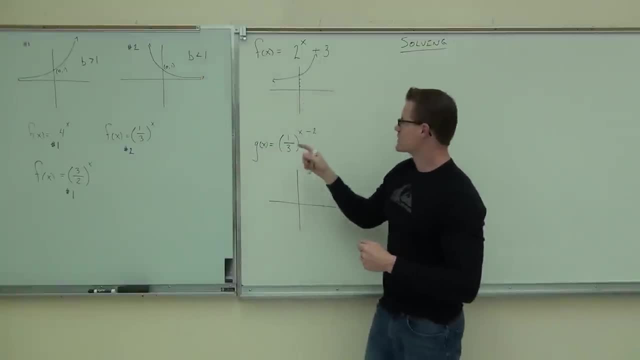 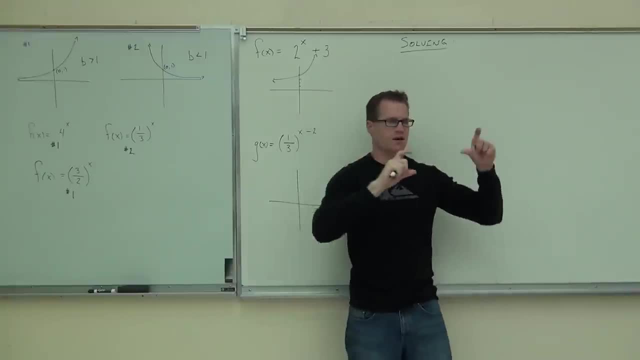 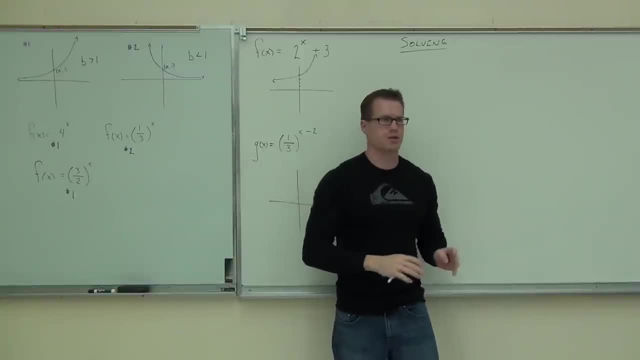 of it. That's shifting it up 3 spots. This one, on the other hand, says: okay, you're going to subtract 2 from your x before you even take that to the exponent. You with me on that. That's not a vertical shift. 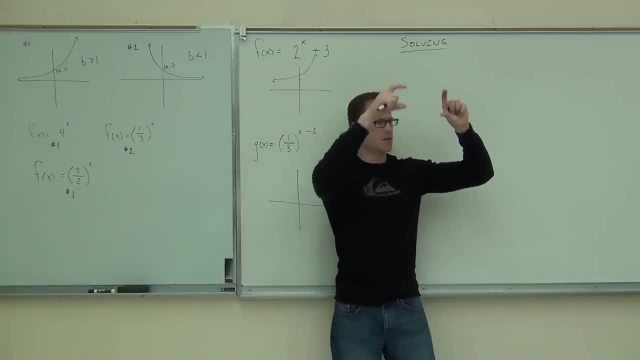 That's a horizontal shift, like we've studied before in chapter 8 and chapter 11. again. Now it's just to be clear that we're not going to be doing on the x, You're going to do on the y, You're not going to do on the y. 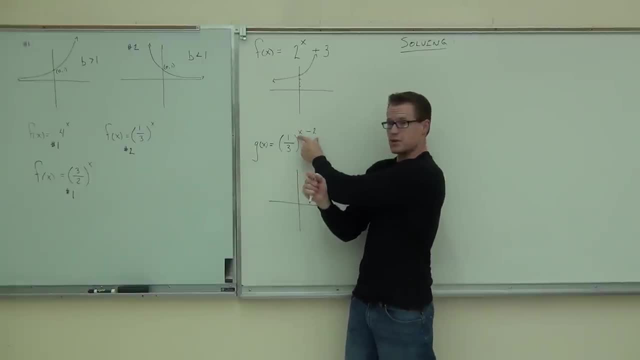 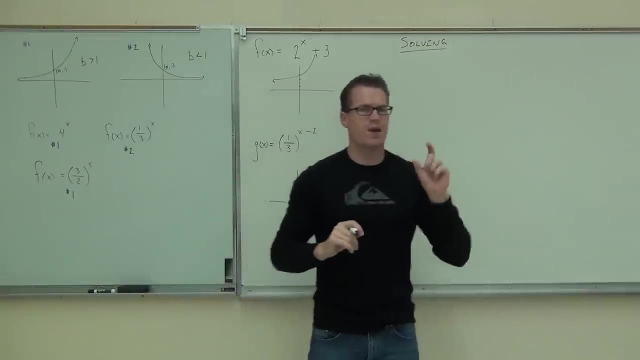 You're not going to do on the y, Do you remember? do you guys see that that is within the function? That is like you have this exponent right here with some parenthesis around. That's what that's saying. Do you remember what minus did? if it's within the function, 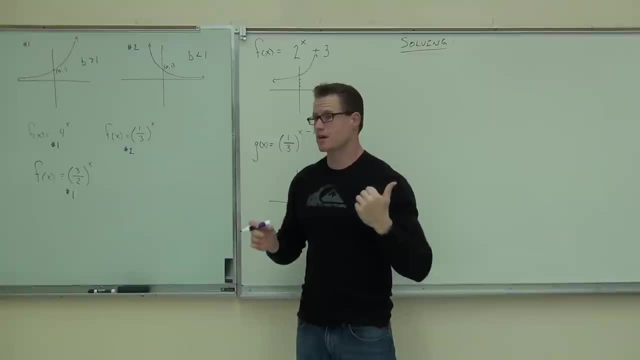 Was it left or was it right? It was to the right, It was to the right. It is like it was the opposite. It's actually slowing down the function. So if it normally started here, remember that we're on this graph. 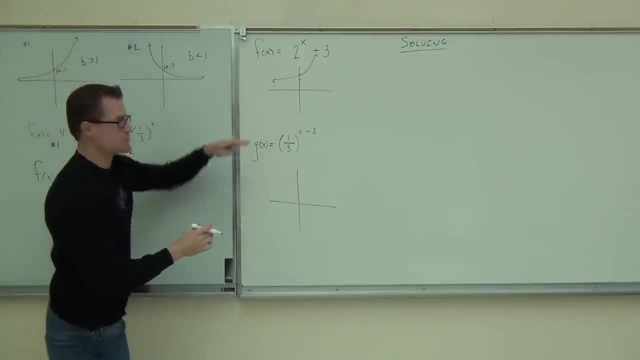 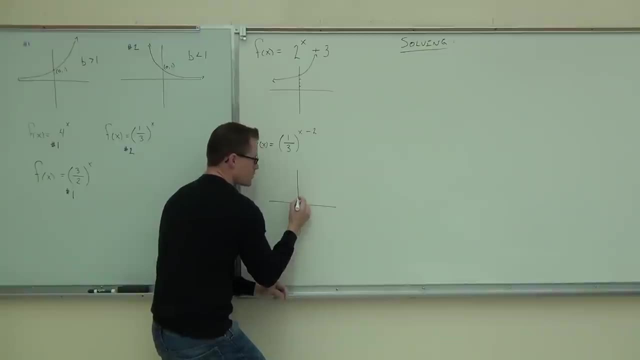 If it normally started here, it's going to start later. It's going to start later, So this would shift it two spots to the what was it again? left or right? Right, Two spots right. So if we normally cross at zero one, check this out. 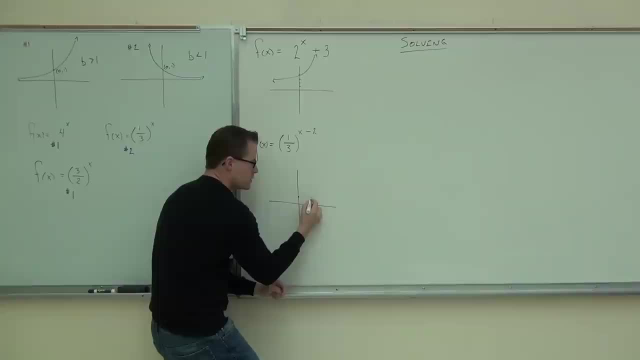 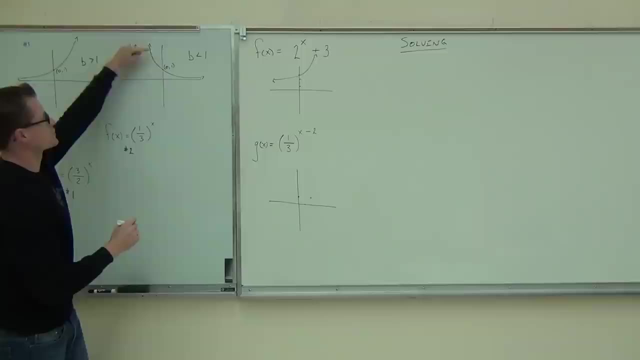 If we normally cross at zero one, we're now crossing at two one. Do you see why we're crossing at two one? It's shifting this spot. look at this spot, this whole graph. but we're going to look at that one value, two spots to the right. 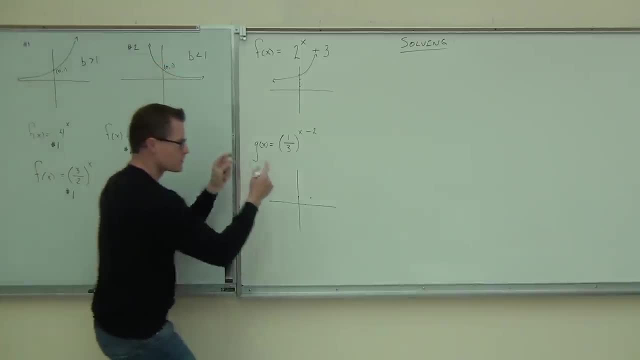 Two spots to the right. Are you guys okay with that one? So we'll read through our graph and just see what we're going to get. Now we don't know exactly where it crosses the y-axis. We'd have to do some work on that. plug in zero. 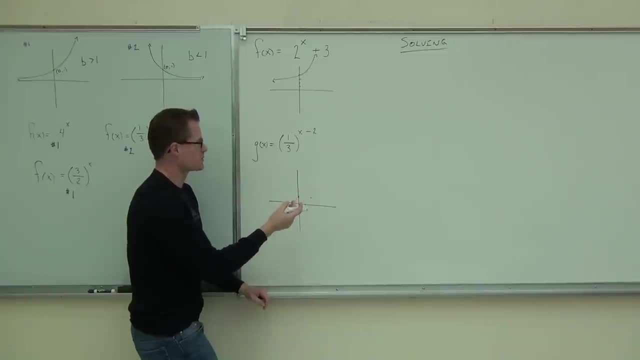 You're actually going to get- let's see- zero negative two. you're going to get nine. You get nine out of that, so we'd cross up here at nine. but basically I just want you to understand that we can still shift our graphs. 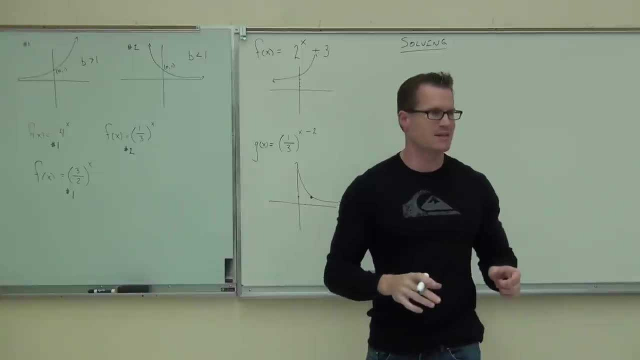 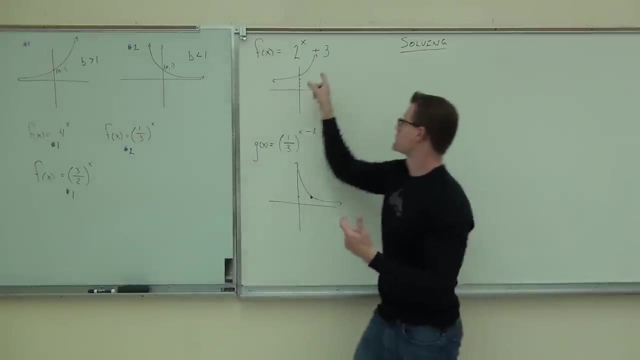 around is what I want you to get across from this. Okay, not exactness. I want you to be able to identify what type of graph you should be looking at and how to shift these things. If it's after the function, again we're vertical. 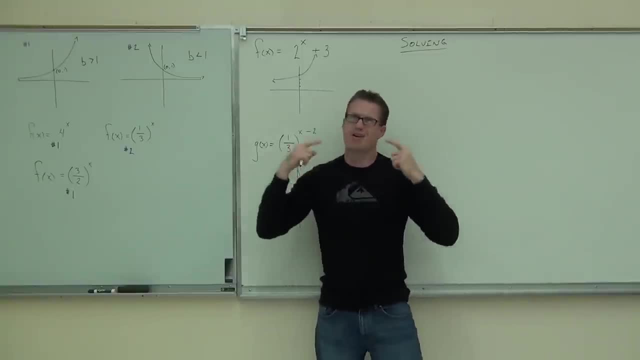 If we're within the function, of course we're going to be horizontal and it's kind of opposite of what you want to think. it is How many people understand our shifting? Do you see the similarity between chapter eight and 11 and now what we're doing here? 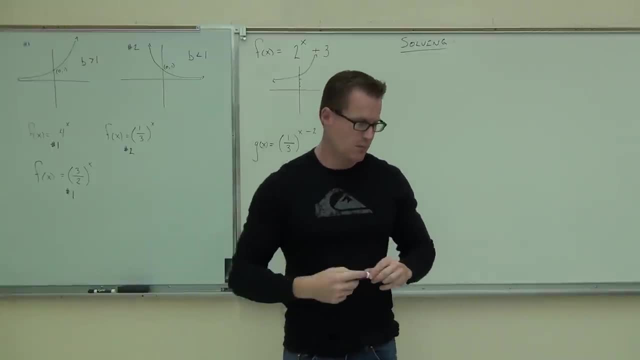 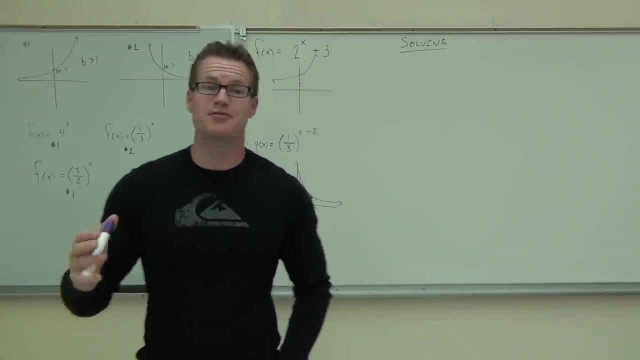 It's the same stuff's getting repeated folks, the same stuff. Now, the last thing we have to talk about in this section is how to solve these exponentials. This is going to be kind of interesting. It's kind of fun. 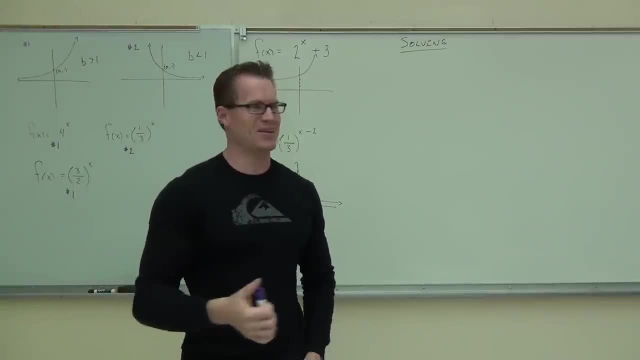 It's like a: do you guys like puzzles? Then you're going to love this Ready for it. You know you'll be doing puzzles over Christmas break, right Sitting there doing. now you can do math puzzles before Christmas break. It's even better. 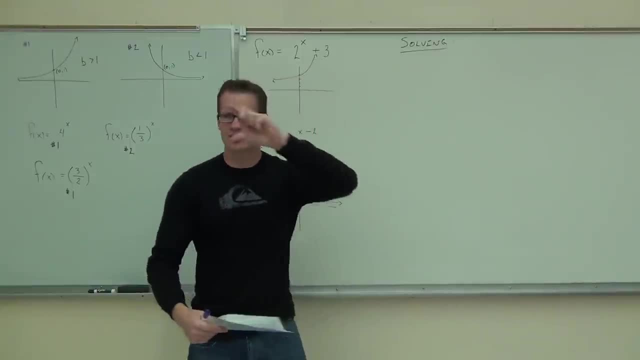 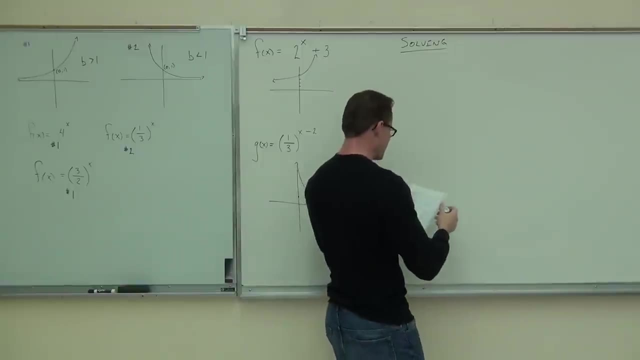 I mean, there's no missing jigsaw pieces. you know, You don't have to bend a corner and bite one off to make it big. This is going to work. perfect, because it's math awesome. Here's the idea of solving these exponentials. 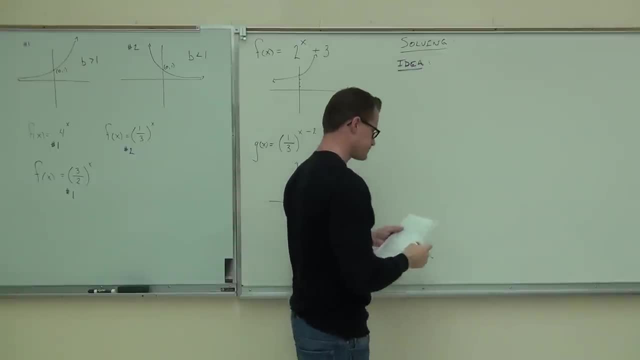 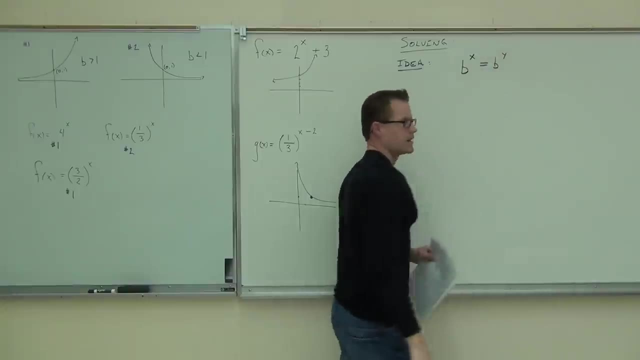 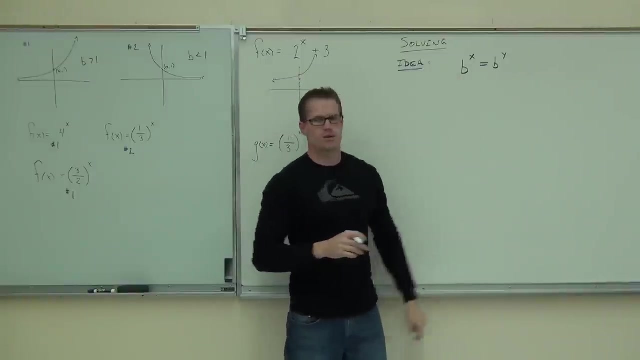 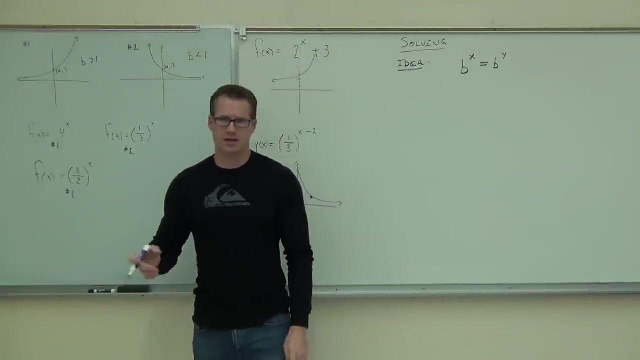 Here's the idea. I want you to assume that we have B to the X equals B to the Y. So basically, our bases are identical. The bases are the same. Are you with me on this? Firstly, can you see it's an equation. 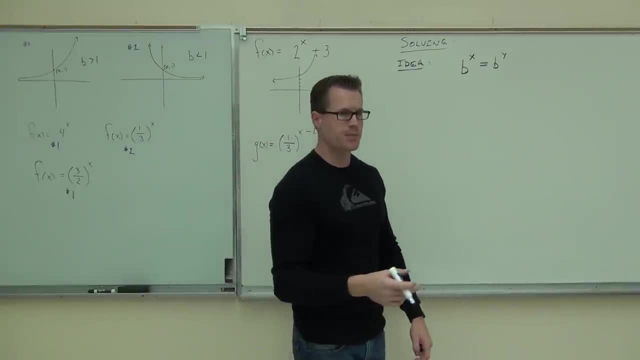 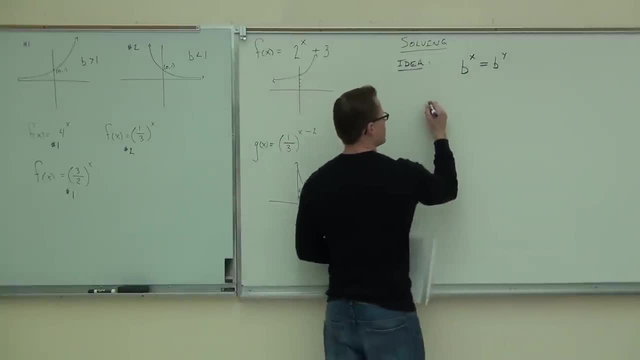 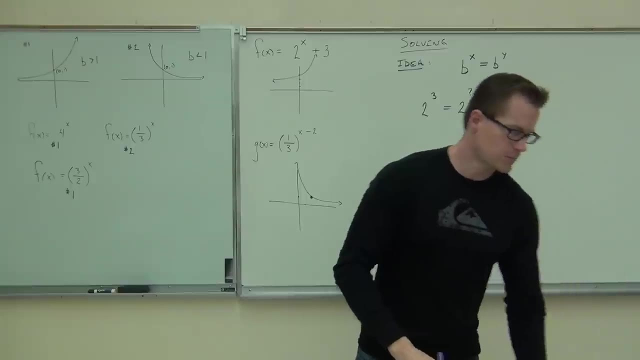 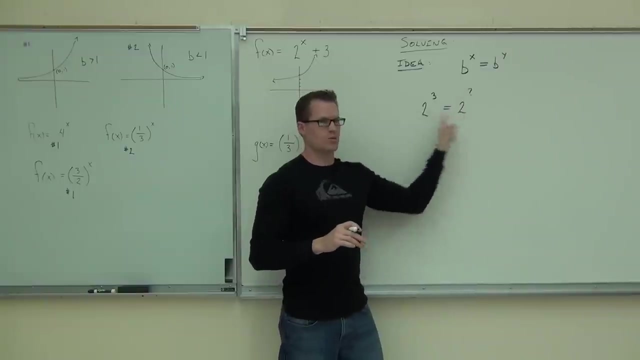 And if you can't answer that right now, let me give you a specific example. Let's say 2 to the third equals 2 to the question mark, And you don't know what that is. What's the only possible number that could be to make this equal? 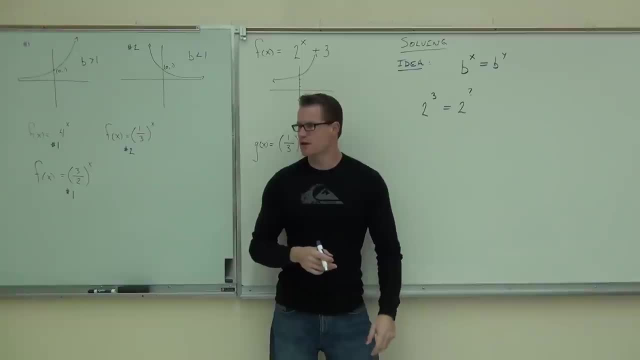 3. 3.. If it's 4,, you're going to have 8 equals 16, right, If it's 2, you're going to have 8 equals 4.. The only thing that this could possibly be. 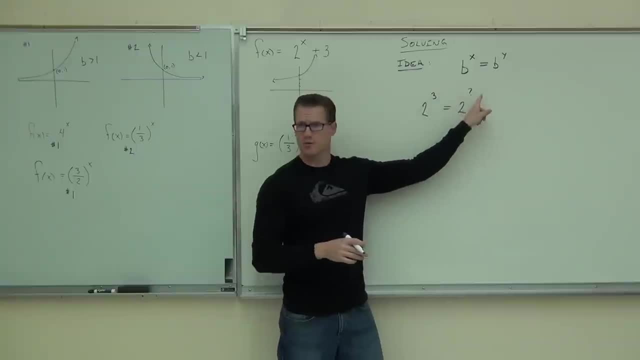 possibly be. to make this equal is also a number 3.. Are you with me on that? That's it. That's the only thing it could be. So here's what this says for us in general: If our bases are equal, if our bases are equal, then our exponents absolutely must be equal, Does that? 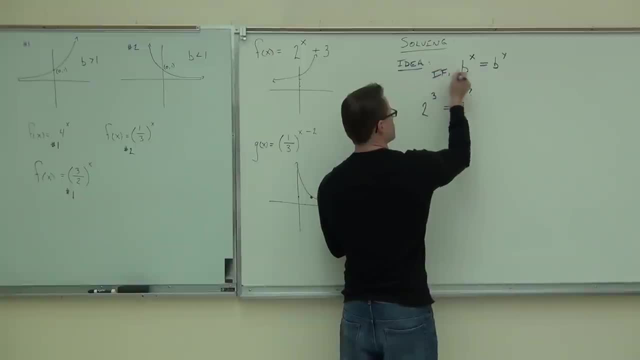 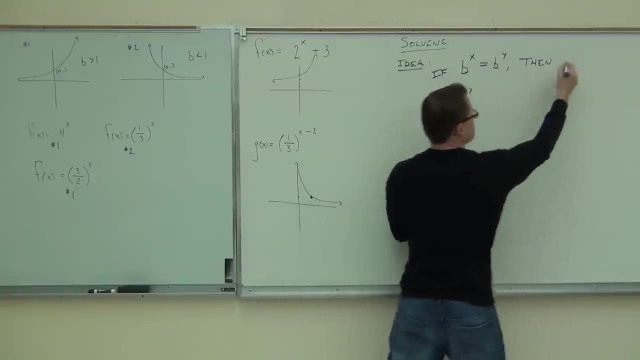 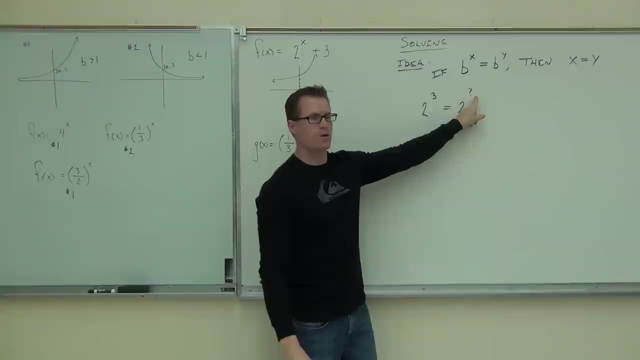 make sense to you. If you have this, if this, then it's very nice. If your bases are the same, then your exponents must be equal. That's the only way that's going to work. If 2 to the 3rd equals 2 to the, I don't know. well, you do know The only way this can possibly. 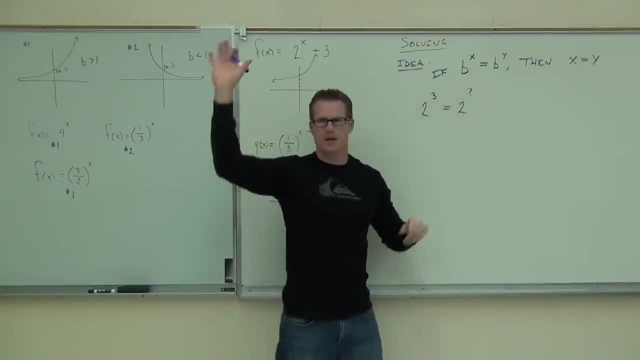 equal is also a 3.. That's the only way. How many of you feel okay with the idea of this? If our bases are the same, our exponents? I didn't get a whole lot of hand raising, so if you have questions right now, it would be a perfect time to ask us. No question? 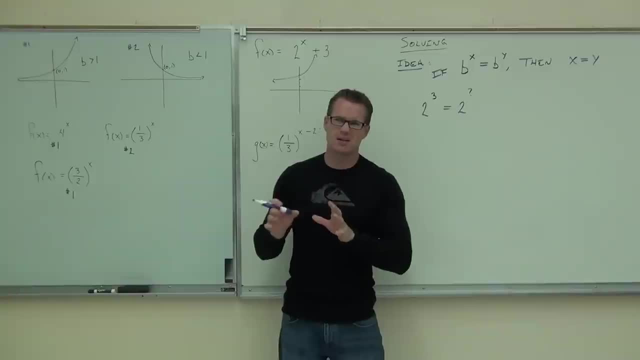 No question. Any questions on that one. Do you get the concept that if the bases are the same, the exponents have to be the same? I mean, try plugging in any number besides 3 there and see if they're equal, Are they? 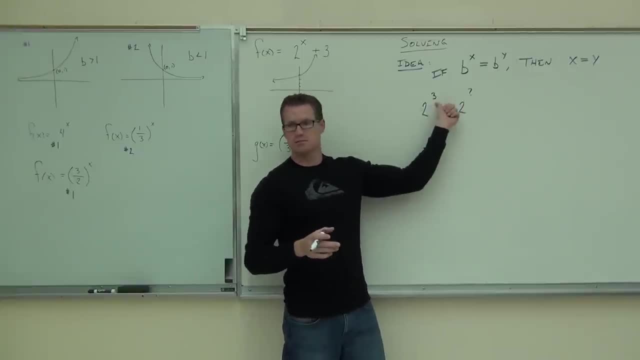 going to be equal. No, The only way that's this is 8, right. The only way this is also going to be 8 is if you have 2 to the 3rd. If you have 2 to anything else, it's not going. 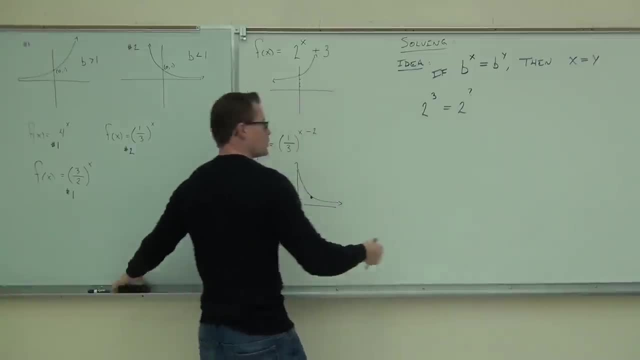 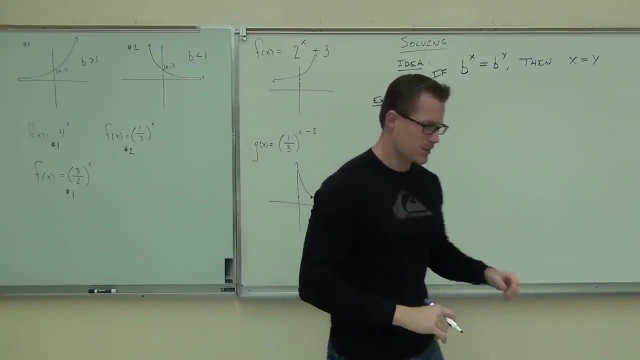 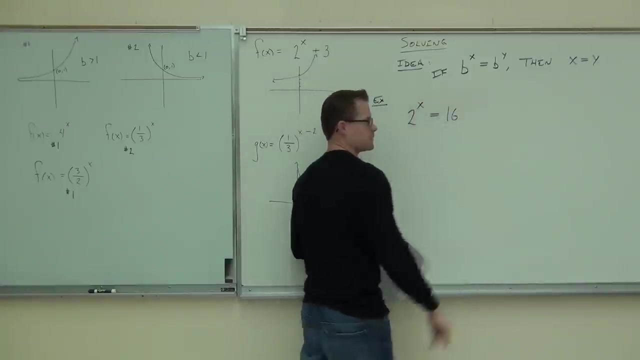 to be 8.. You're going to have something different. That's the whole idea. Now, how we're going to use that. how we're going to use that is with problems like this: 2 to the x equals 16.. Wait a second: 2 to the x equals 16.. I'm trying to solve for x. 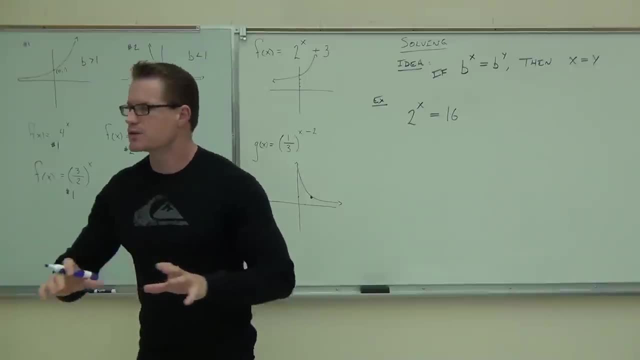 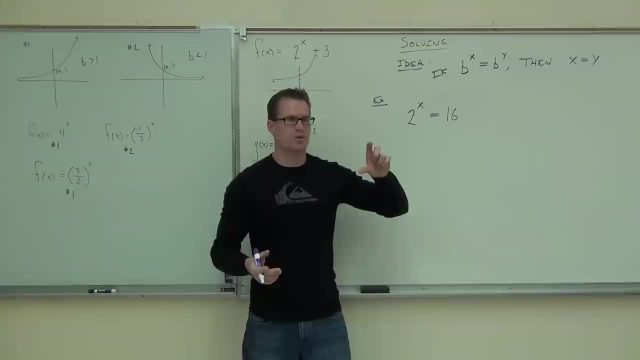 right, But really we have no algebraic way to manipulate this problem. to solve for x, What are you going to do? Are you going to divide by 2? That's not going to work because x is still an exponent, right? Wait a second. How do I solve for x in this case? We're going 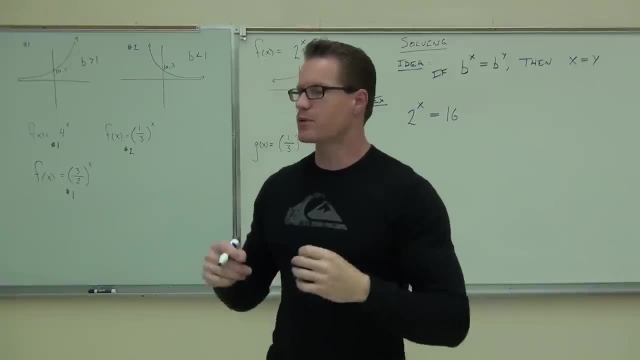 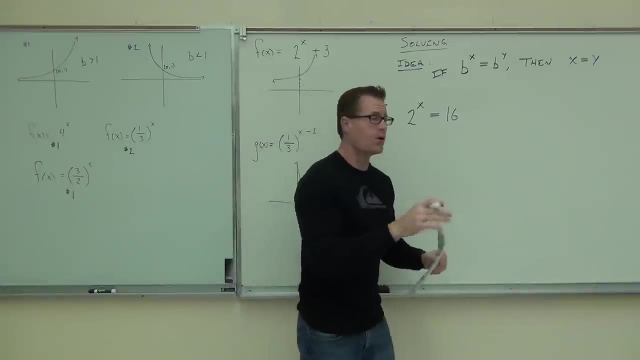 to use this fact. So here's your ultimate goal when you're dealing with exponentials. This is it. This is all we have for now. In just a while we'll have something else, But for now, all we have is the idea that. 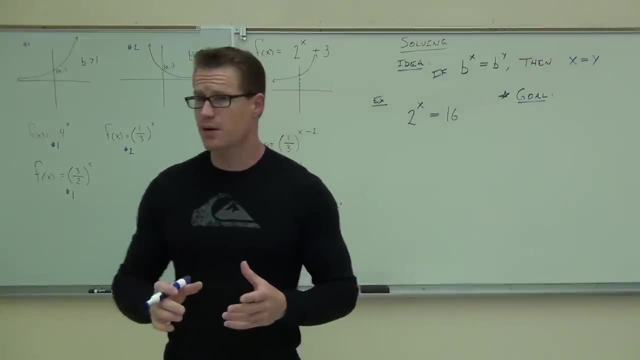 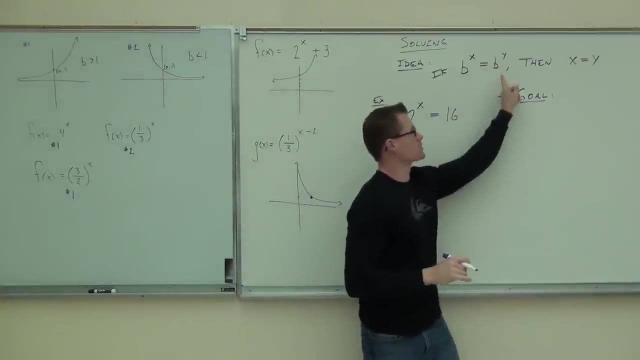 if you can make your bases the same. let's take care of the words. if you can make your bases the same, then you know for a fact that your exponents are going to be equal. You follow me on that, If you can make your bases the same. So our goal is: you're going to try. 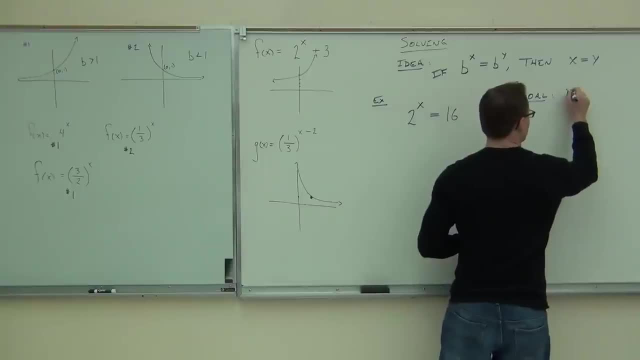 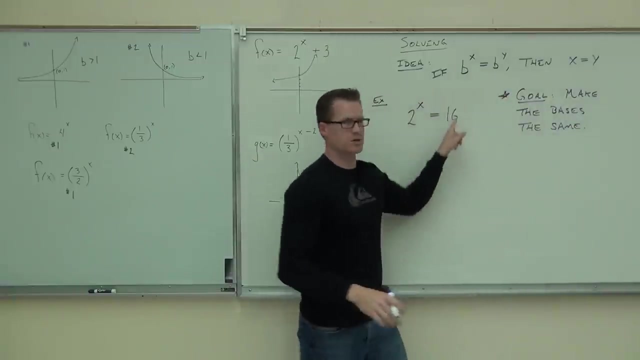 to make the bases equal, Make the bases the same. Now you got to buy into this fact before you can do this problem. So if you don't buy into this fact, this is not going to work. Do you buy into the fact that if the bases are the 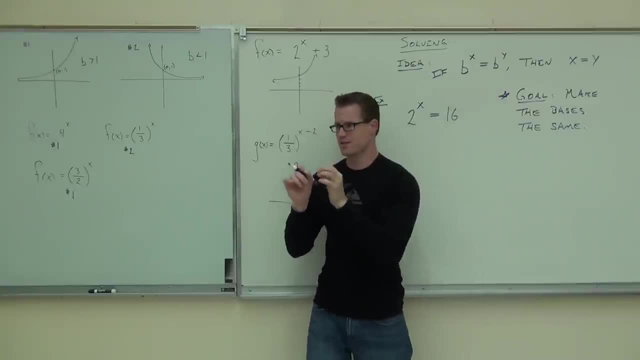 same, then the only way these two things can actually be equal is if the exponents are equal. Do you follow that? If not, this isn't going to work. If you're like, well, I don't understand that, Well then you're not going to get this part. So if you don't, if you're 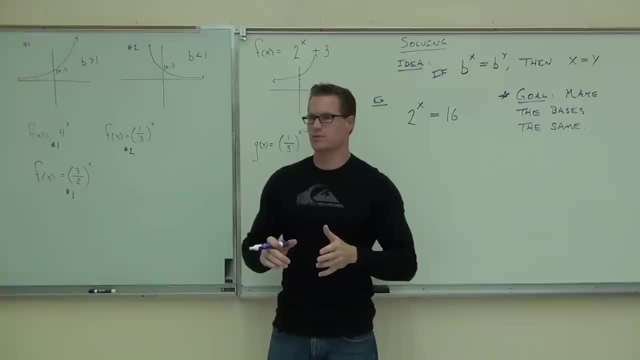 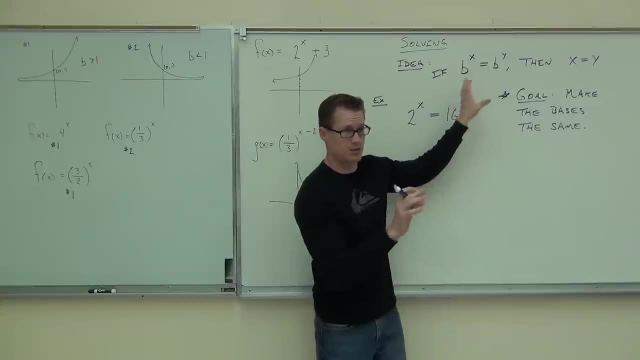 like I really don't get it. do you have any questions for me about that one? Are you guys okay with that? Give me a head nod if you are, That the only way these two things are actually going to be equal and the bases are the same is if those exponents are also the 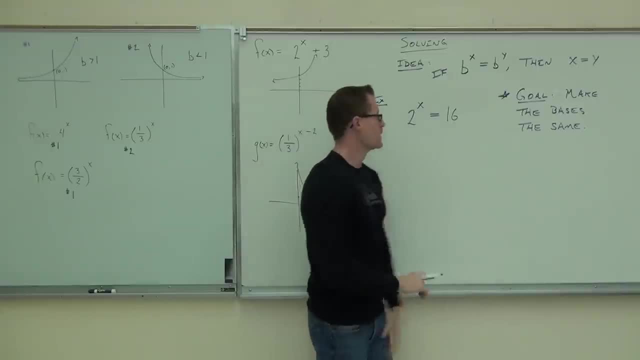 same. It has to look identical. You follow me. It's got to be the same thing Now. so if we're, our goal is to try to make the bases the same, Do I have the same bases here right now the way it is? 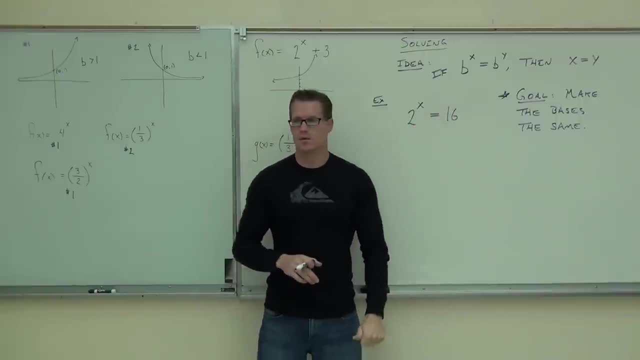 No, That says two. to the x, That says 16.. No, That says 16.. Well, what I need to do is somehow make that into a two, a two to some power. Do you follow me? Because our base over here that's given. We can't change that one right. 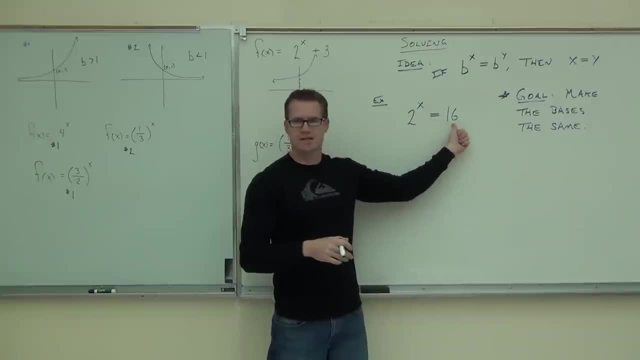 now That's two. two to the x, This one though that's 16.. Can you write that as a base of two to some power? Two to the fourth, Two to the fourth. So, if we can translate this thing a little bit, we got two to the. 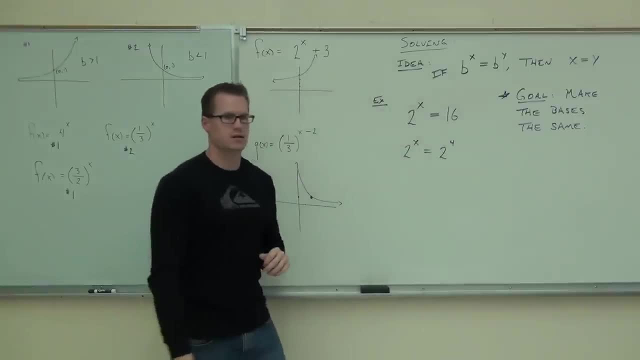 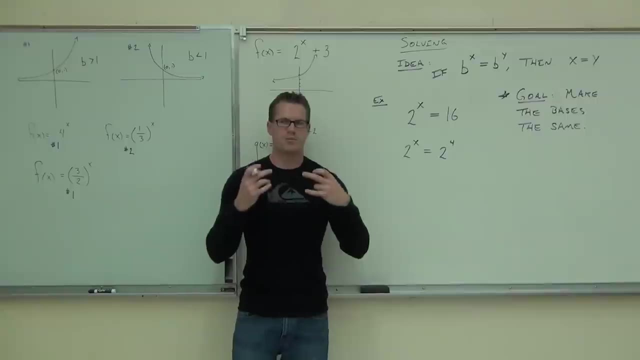 x equals two to the fourth. Is that still the same thing as 16?? No, Well, that's awesome. You know why that's awesome? Yeah, Well, look at the problem. Do you have the same base? Yes, Right now we know that if the bases are the same, the exponents must be equal, Do you? 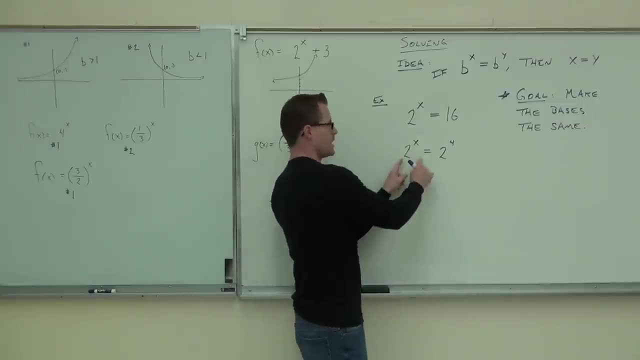 follow me on that one. So why does it work for us? Well, shoot, I mean, if you have, if you have this. look at this statement. It looks identical to that, except in this case, b is two and your y is four, right? Well, look at the next thing we could do Essentially. 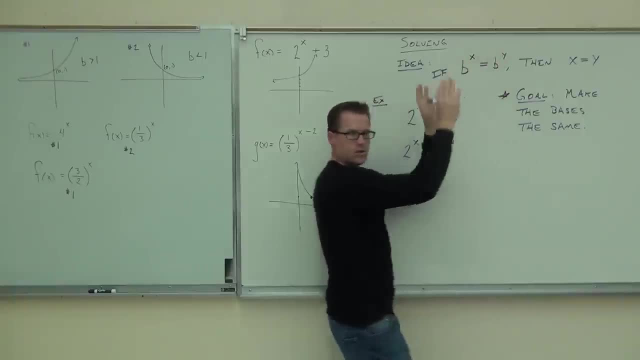 we can drop our bases. Do you see that If the bases are the same, you can drop your bases. You go: oh well, that's the same thing. You can drop your bases. If the bases are equal? b to the x equals b to the y. that means x equals y, Two to the x equals two. 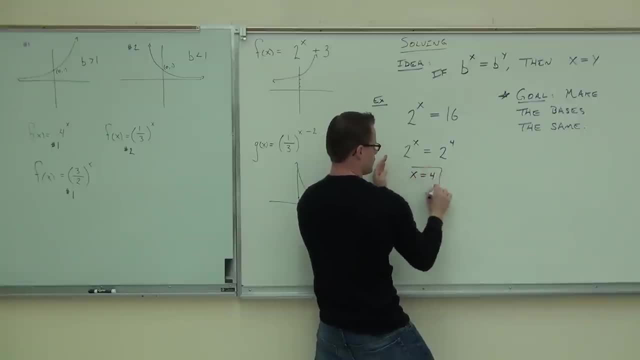 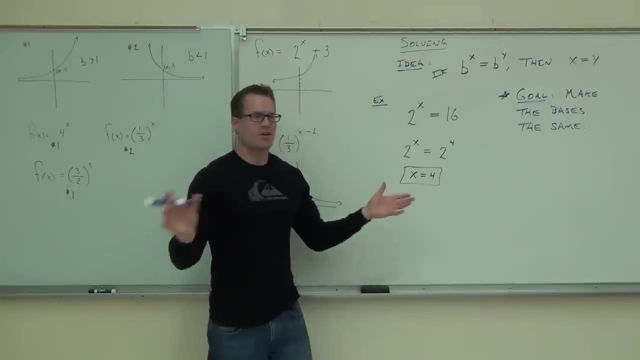 to the fourth. that means x equals four. Are you doing that? Isn't that kind of neat. Yeah, Yeah, that's cool, right? Well, that's nice. Nothing, nothing, That's it. It's just manipulating those bases. 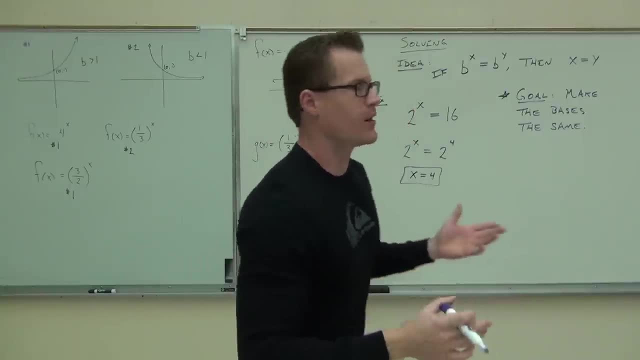 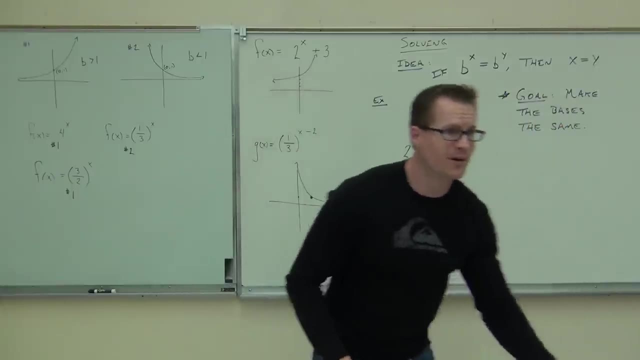 to get them to be the same in this section. That's your whole idea here. Now can I get a little bit more complicated than 16?? Sure, Sure, 16 is pretty easy, right? I hope, I hope, Well, I hope you're able to understand that idea. Good, Notice how you had to get that. 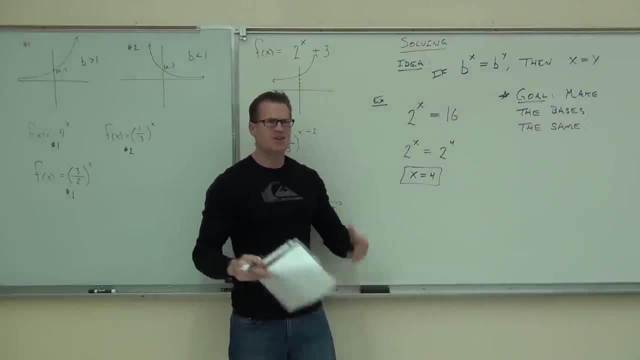 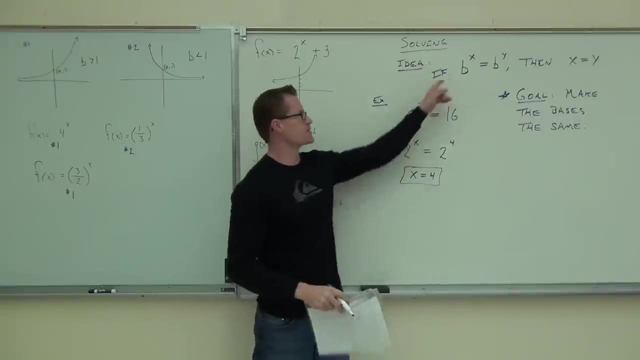 before you get this right, You have to understand that concept, otherwise you're like what's going on with the two? It's magic, Harry Potter. You have your math bond out and you're just: no, this is magic, right? This is using this fact right here that if the bases are the 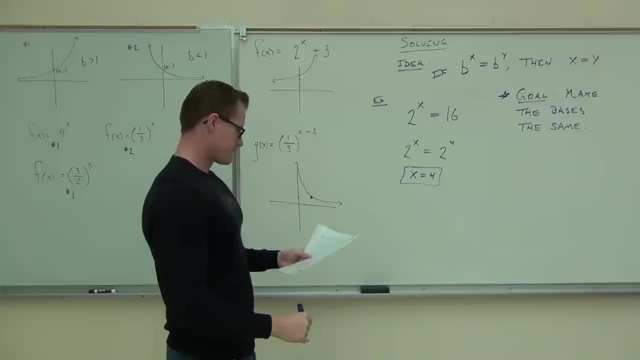 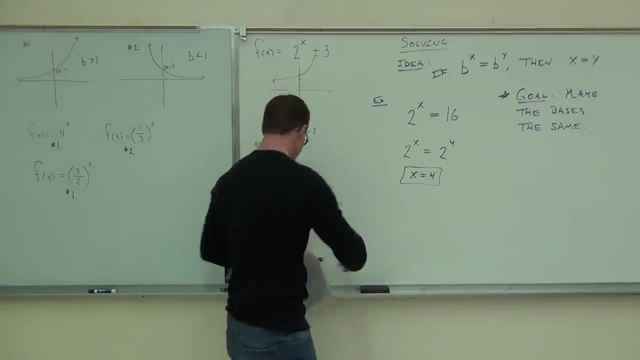 same. all right, the stones have to be equal. That's the whole idea. I'm not Harry Potter, I'm more like Voldemort. I've already told you this. Except they don't have that nasty looking, weird snake face thing. 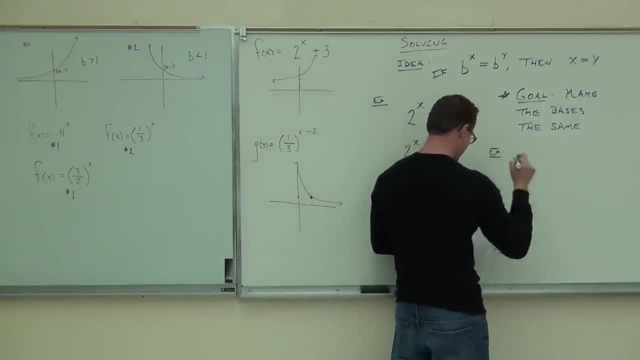 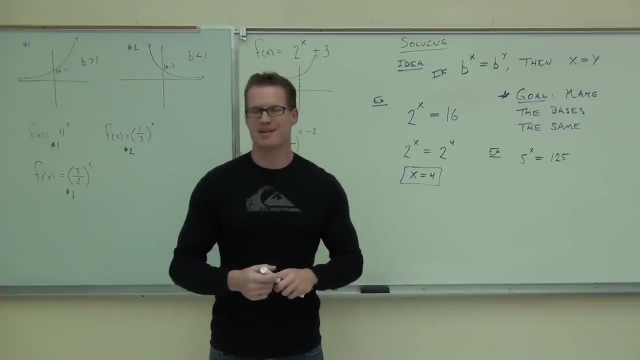 I hope. I hope Let's try another one. Do a couple more together. I'll give you a few to do on your own. We'll talk about an interest problem. It'll be very interesting, And then we'll continue. Five to the x equals 125.. 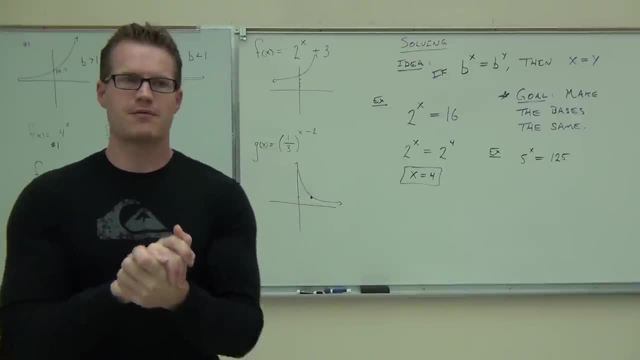 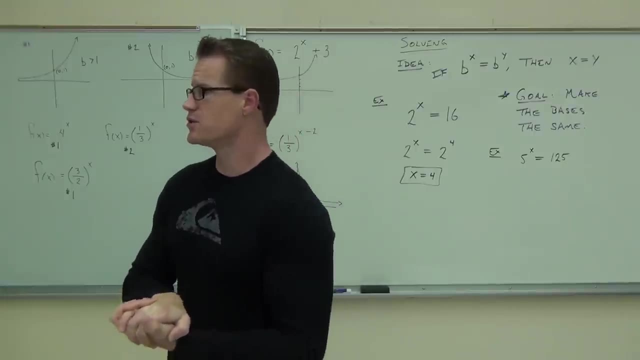 Are our bases the same right now? No, We have five to the x equals 125 to the first. That's not going to work for us. We want five equals five. as far as the bases go, Can you change 125 into a power of five? 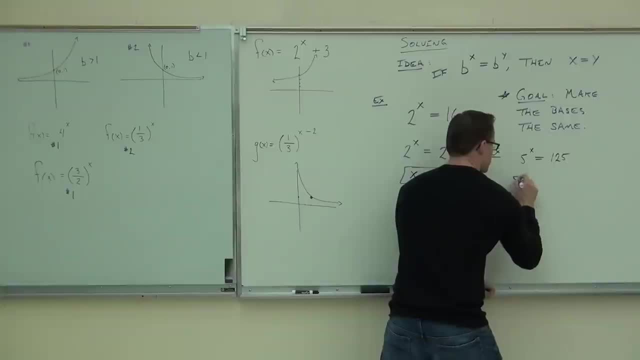 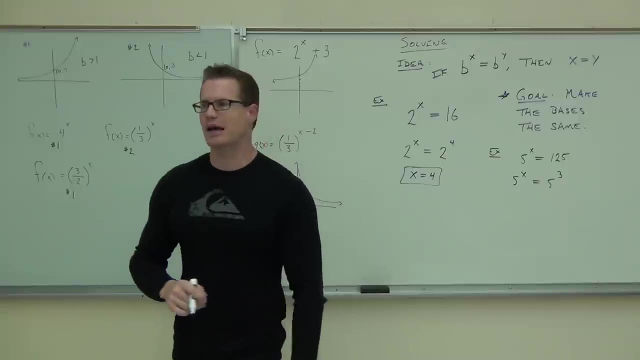 Five to the third, Great. So our whole goal here is to try to make this equal. this, our two bases: Five to the third, That's the same thing as 125.. How much is x? And you're done As soon as you make those bases the same. 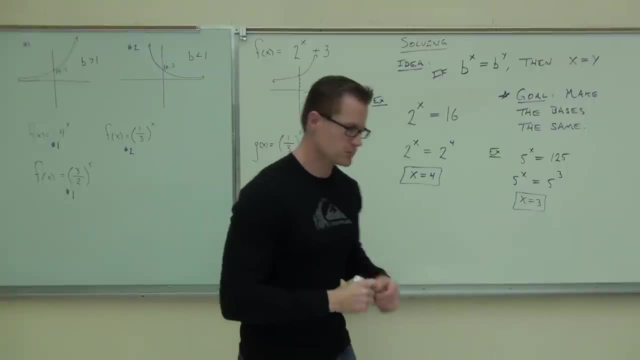 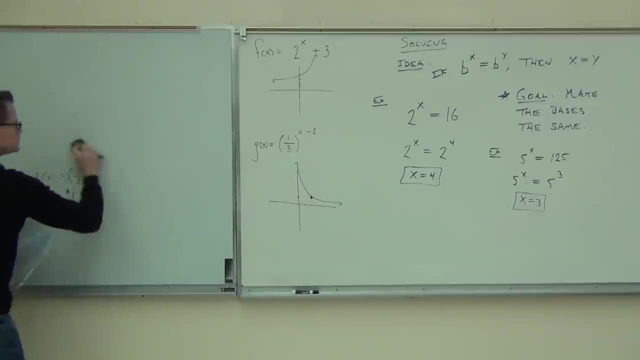 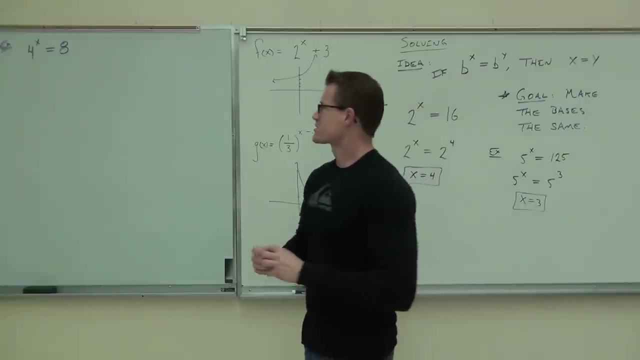 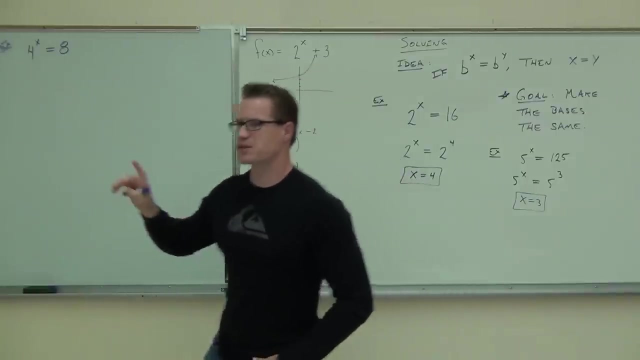 you set your exponents equal to each other. Four to the x equals eight. Okay, Well, it's definitely an exponential, because our variables in the What's our base over here? Okay, Your goal is to try to make your bases the same right. 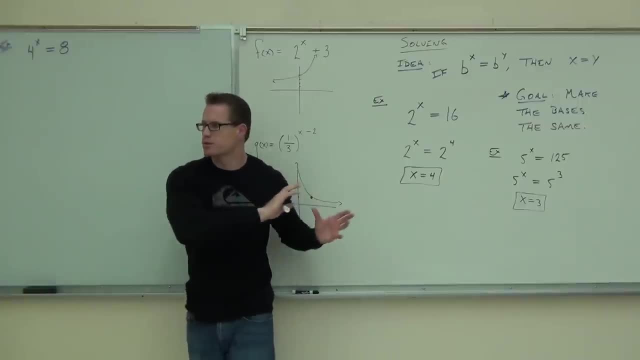 Now watch carefully If you get that, great. but that's not the only thing we're doing today, So you've still got to be focused on this next step. here. There's some other manipulation we can do. Can you write this as four to some power? 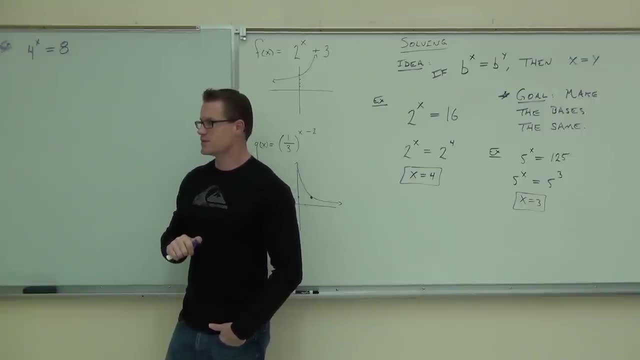 Don't you give me four squared, because four squared is 16, right, You can't do that, You can't go. oh, four to the x equals four squared. I'm done, Okay, That's just two. No, No, it's not two. 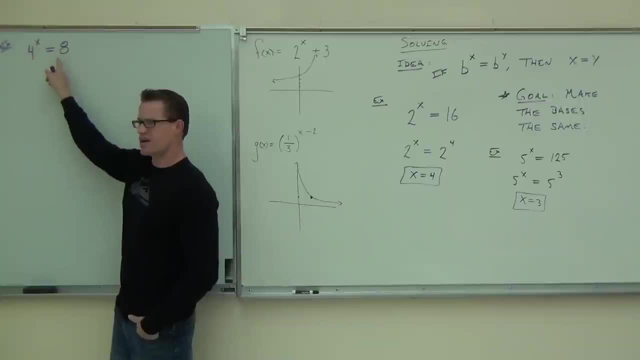 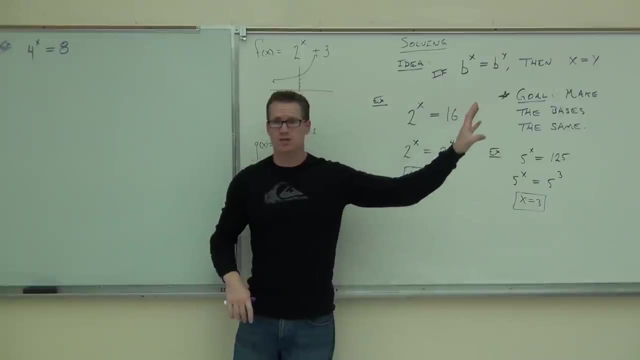 Why Have you plugged in two? You get four squared equals eight. Does that make sense? No, You can check your work here. right, You should be able to plug in those numbers and they actually work out in your original equation. It does here. 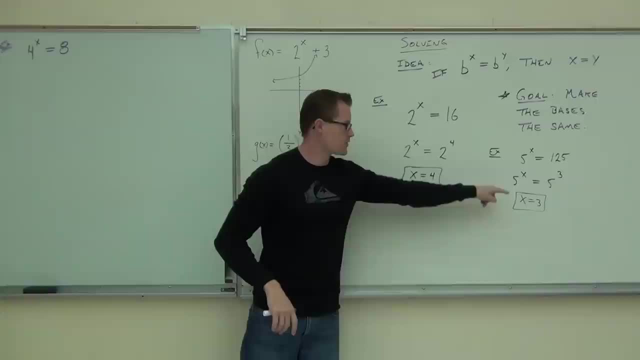 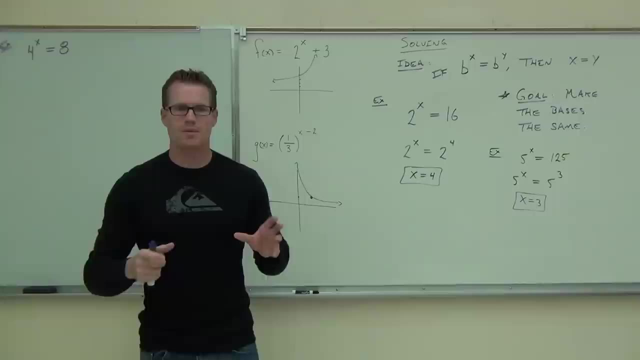 It does here, It does there. Two to the fourth is 16.. Five to the third is well, 125.. Here we've got to change both bases, So occasionally you'll come across a problem where it doesn't look. 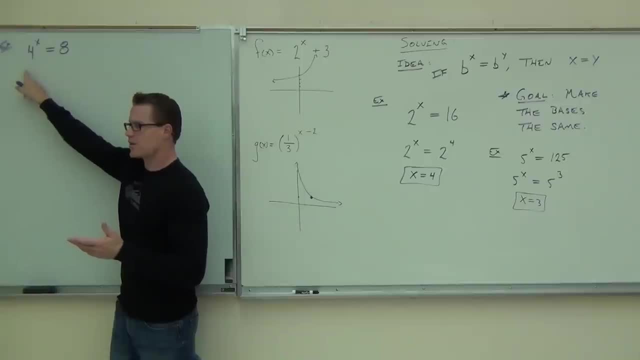 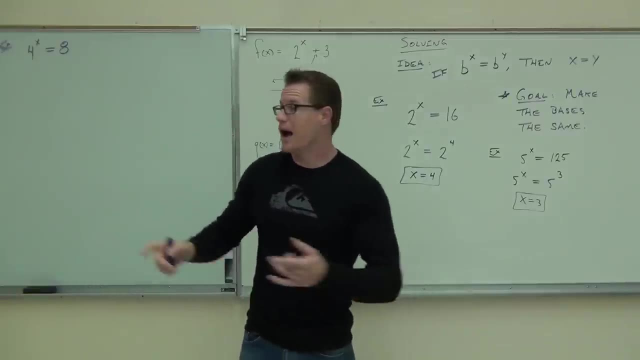 like you can make common bases out of it. Well, this one. you can't write this as four to any power. However, do they both have? Do they both have a base that you could write in common? Yeah, How could you write this one? 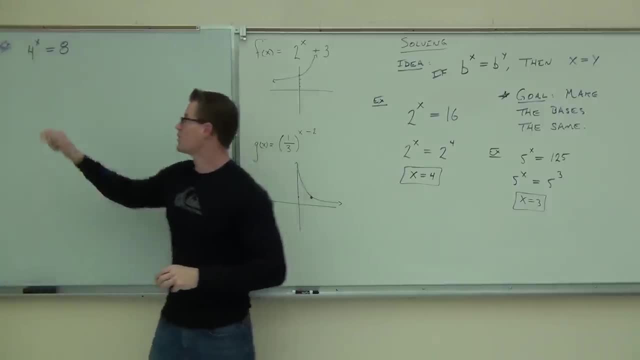 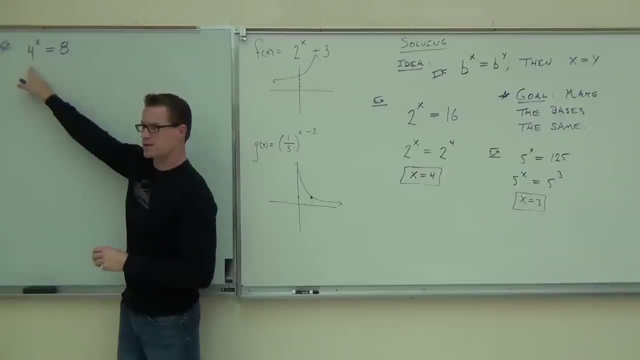 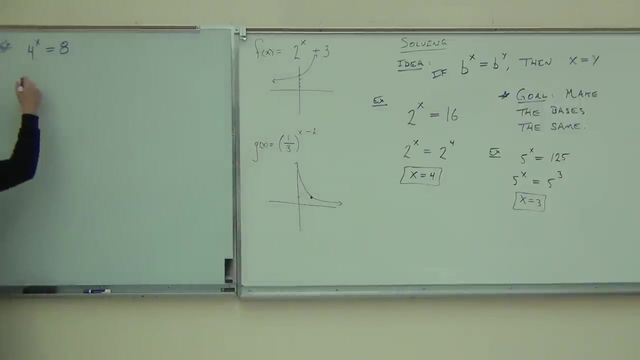 Think about a smaller base. How could you write four as a power that this one could share as well as a base that one could share as well? You could write this four as what? Two to the what power. Okay, So instead of thinking of this as four to the x, I can think of it as two squared. 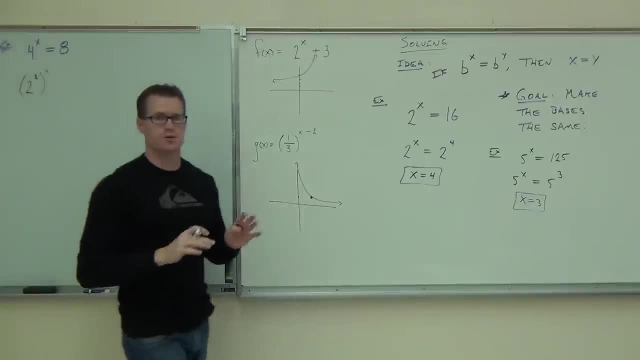 To the x. Two to the x. Okay, All right, All right, All right. Is that still the same thing as 4 to the x? Yep, So you're still looking for a common base. only this time you've got to look for it within those numbers. 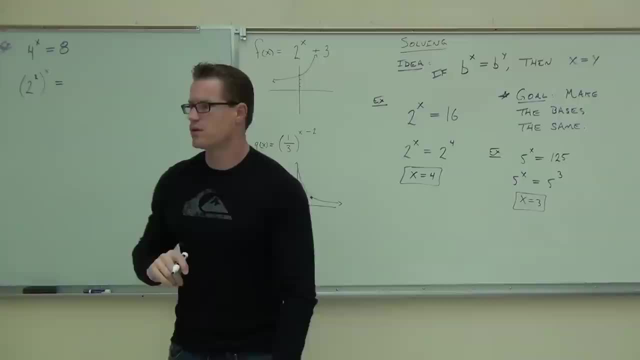 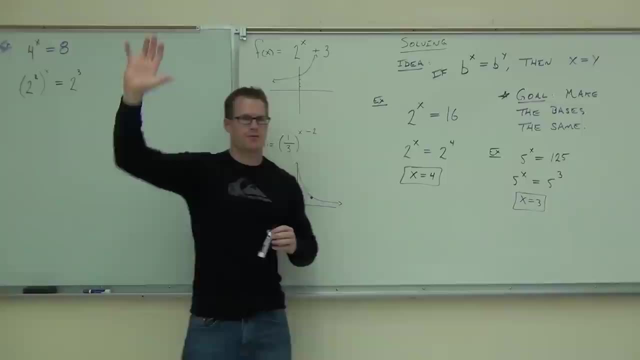 How about 8?? Can you write that as 2 to some number? 2 to the third, 2 to the third? Okay, I need to show of hands how many of you were able to follow that one Good. Okay, so you can't go directly for the 4 here. 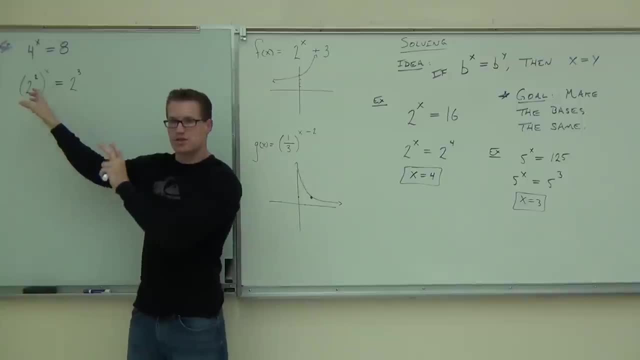 You can't write that as 4 to any power. Here, though, you can write this as 2 squared and 2 to the third That does have the common base of 2.. Are you with me on that? Now, this is going to take just a little bit more work on this side. 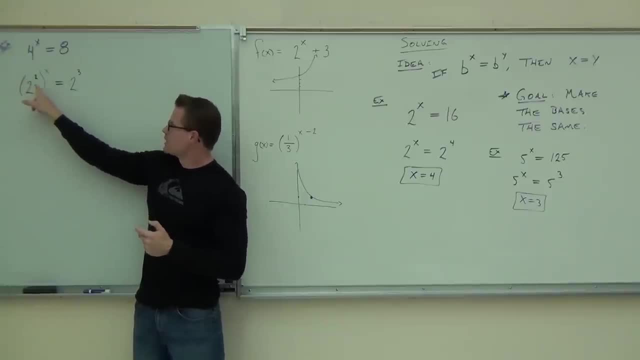 a little bit more work over here. What do you do when you have a power raised to a power? Do you add, Do you subtract, Do you multiply, Do you divide? Which one Multiply? I only have a couple people saying that. 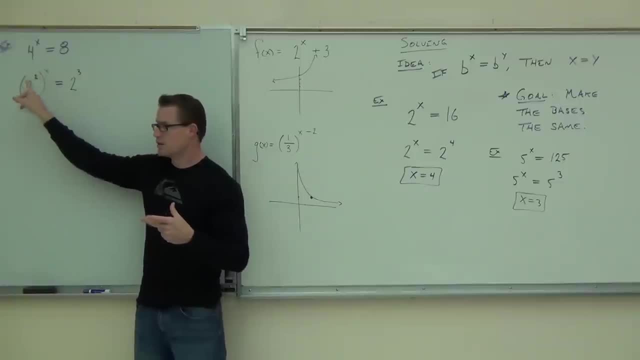 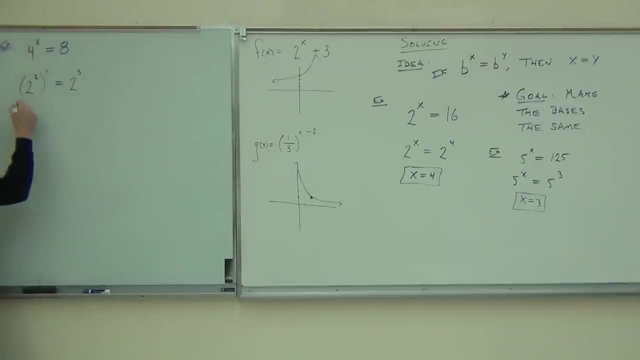 Are you all familiar with the multiplication there. So, instead of 2 to the second, to the x, could you do this? Could you do 2 to the 2x? Yep, What's 2 times that You're multiplying those right? 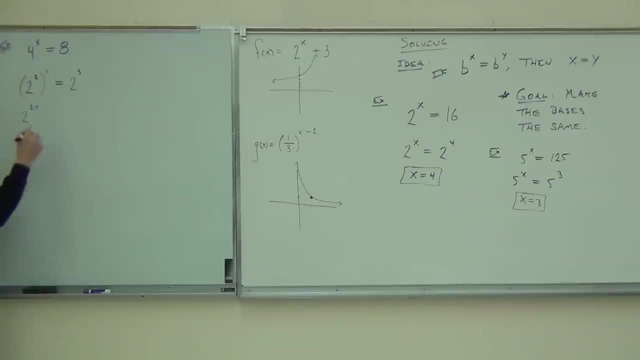 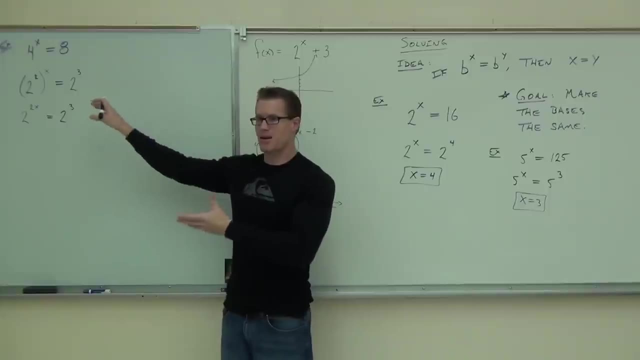 2 times x is 2x equals 2 to the that side. we didn't have to do anything on. Hey, look at the board. Do you have common bases now? That's awesome. What do you know about our exponents? 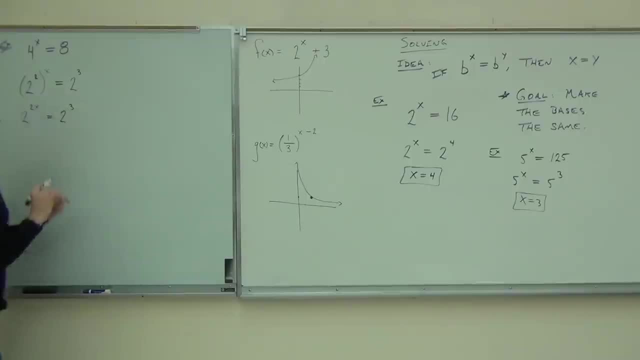 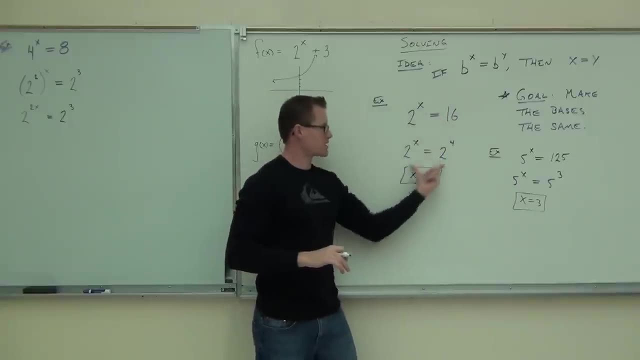 If our bases are the same, what do you know for a fact about your exponents? They're equal. They are equal. Look what we did over here. We had common bases- exponents were equal. We made common bases- Exponents were equal. 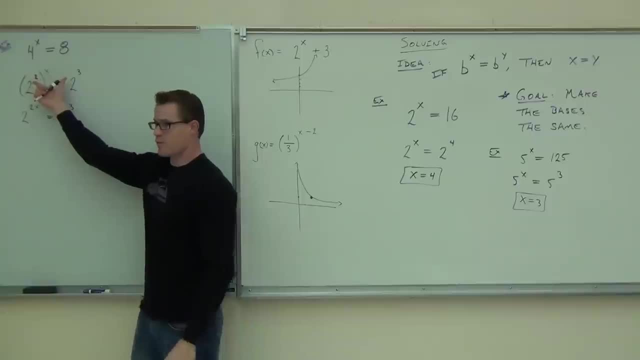 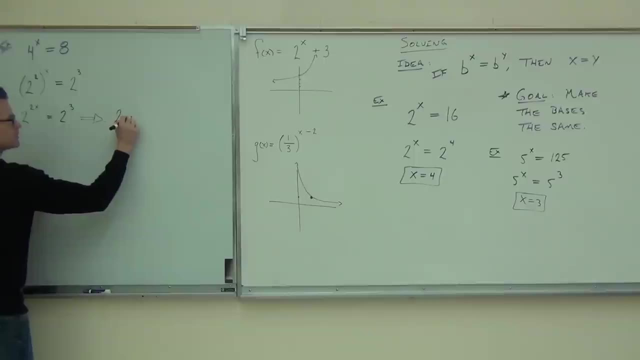 We made common bases, Exponents were equal. We now, with a little bit more work, we made common bases, But what this means is that your exponents have to be equal. You can essentially drop your bases if they are the same in your equation. 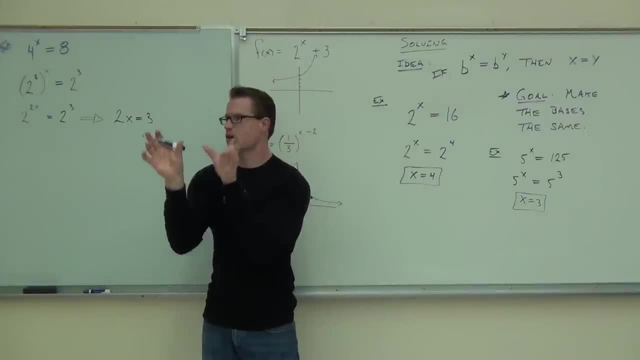 That's what we've done. We said: oh, bases, those are the same thing. That means our exponents must be equal. That lets us go from here to here. Would you raise your hand if you're okay on that problem so far. 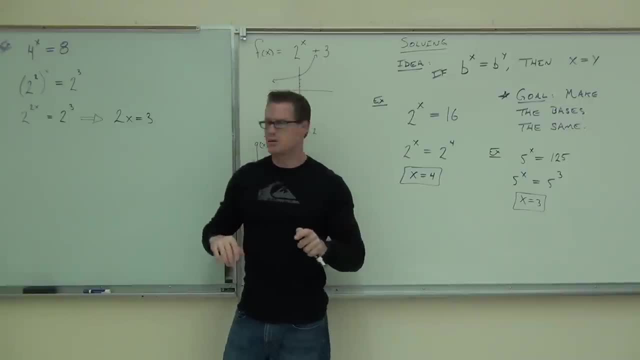 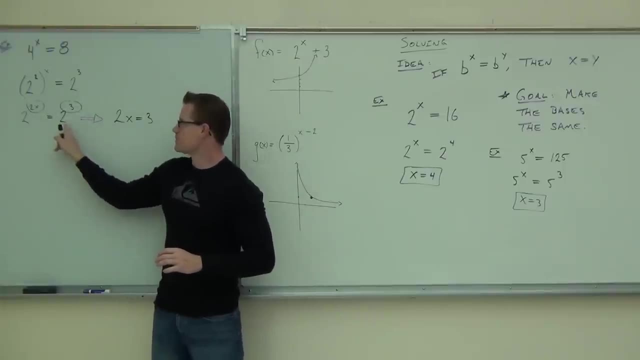 Okay, How do? x is equal to 3?? Well, this is my exponent, right, And that's my exponent. You know, if your bases are the same, your exponents must also be the same. It's got to be there. 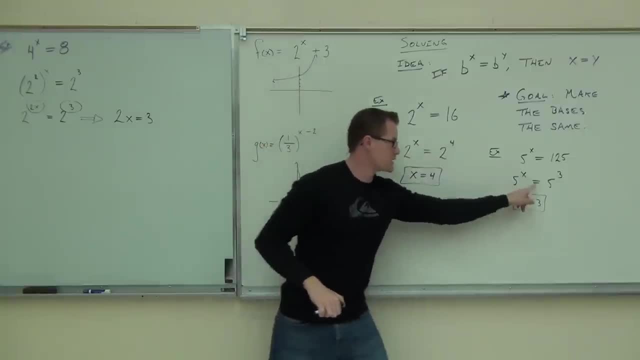 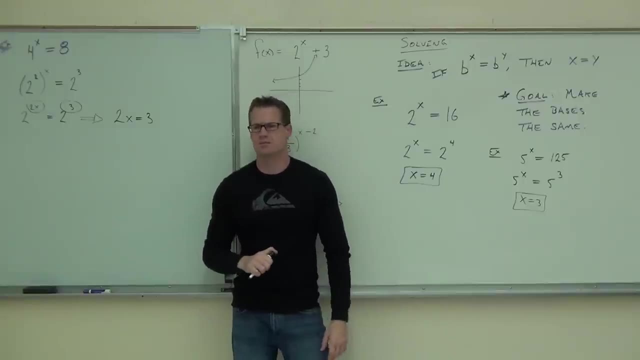 Just like over here, x was equal to 4,, x was equal to 3,. 2x is equal to 3 in this case. Now are you done? What do you got to do now? I have to divide the 2 from the x. 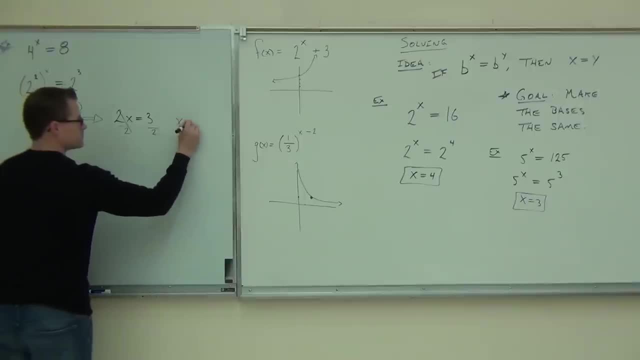 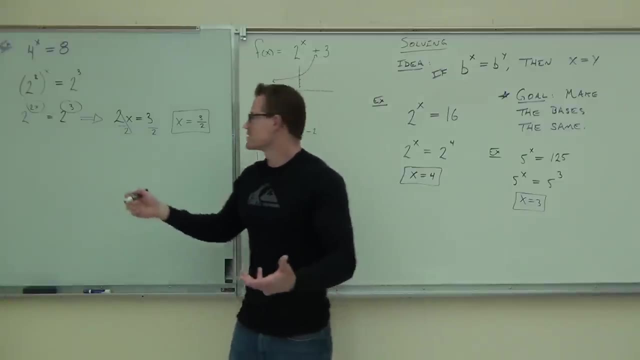 If you do that, Is it okay to get a fractional exponent? Yeah, In this case that means a square root of whatever, that is, a square root of 4 cubed. That's what that means. It's a 3 half power. 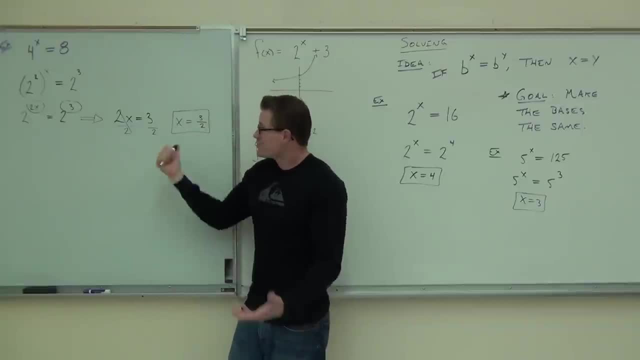 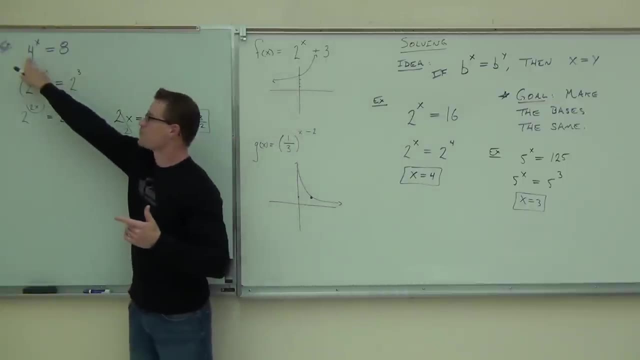 Remember talking about roots and exponential powers like that. That's what we've done. If you take on a calculator and you do 4 to the 3 halves, you're going to get 8.. If you do it in your head and you go: okay, the square root of 4, remember the square root. 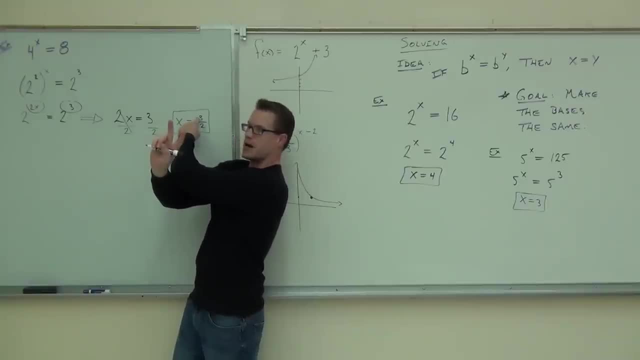 What's the square root of 4? 2.. Now raise 2 to the 3rd power. What do you get? 8.. You get 8.. That means that works out. That is the equation there. That's a solution for our problem. 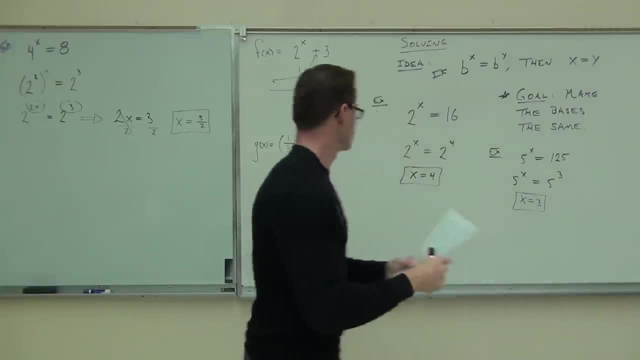 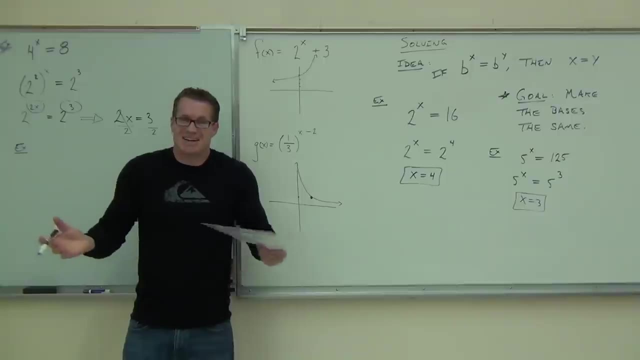 You still with me on this? Yeah, Okay, Let's try one more together. I'll give you a few to do on your own. Can you see how, when you get the hang of this, this is kind of fun. It's kind of neat. 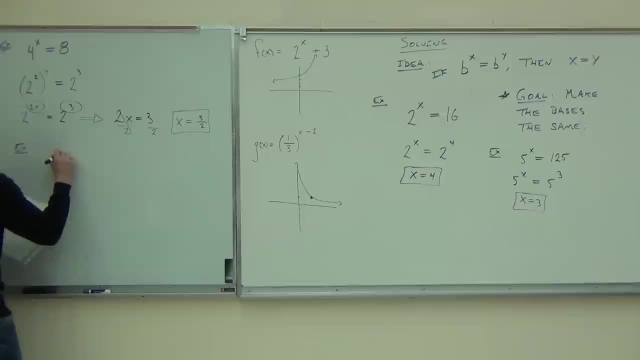 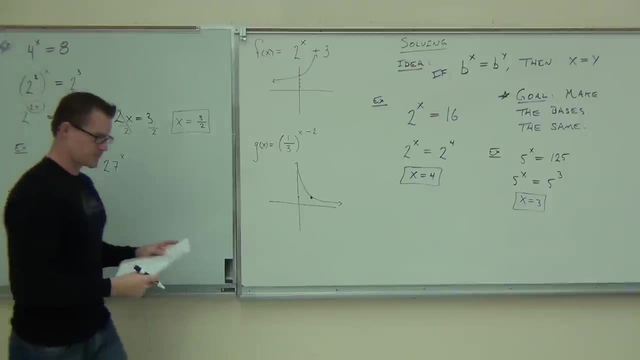 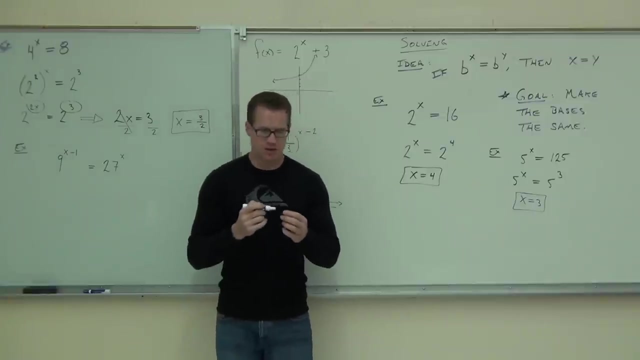 Well, I like it. Okay, Just always remember your goal. Your goal is to try to make those bases identical. That's what you want to do. So the first thing you look for is: do you already have some number that you can make the other base into? 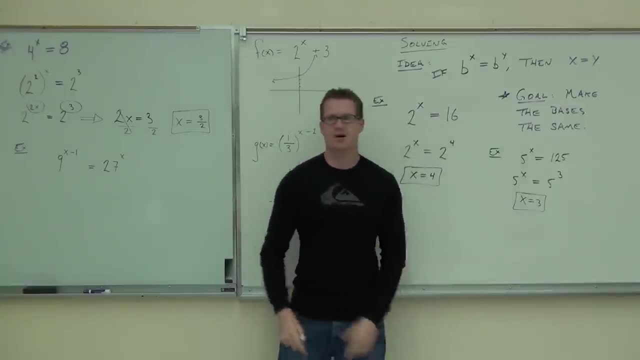 Well, for instance, here we had 2 and 16.. That was great. We had 5 and 125.. That was great. 4 and 8, we could not do that with. You can't write 8 as any power of 4.. 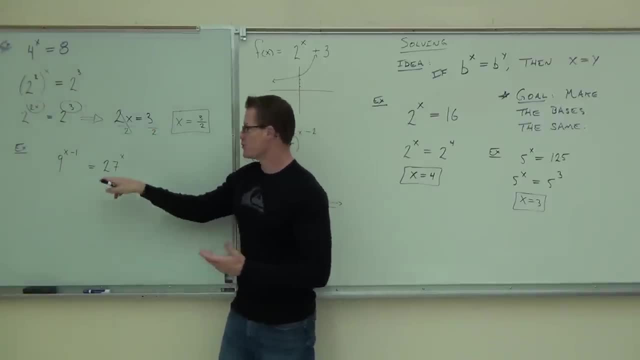 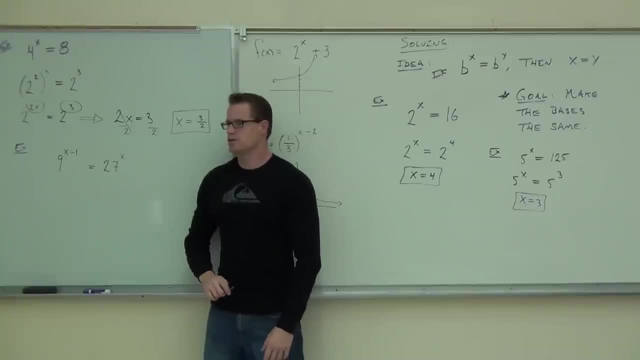 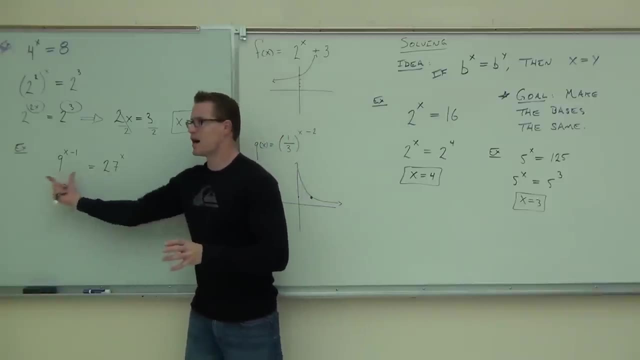 No, I mean, if you try 9 squared, you're getting 81, right? So I mean you can't do that. However, can you look for a number within 9 and 27 that you could write both of them as some power of? 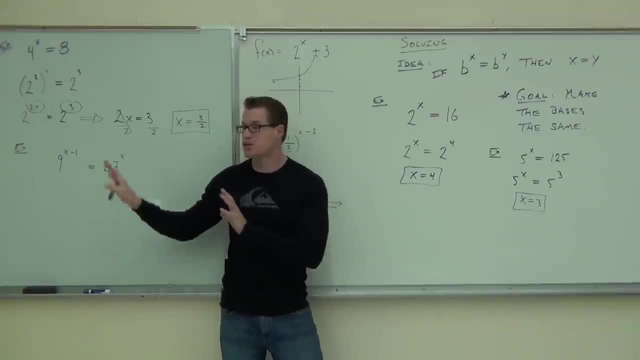 So you go 9, 27.. Those should have a common base somewhere in there, Otherwise you can't do this problem, So you're always looking for that. What number do they share as a base? 3. 3. 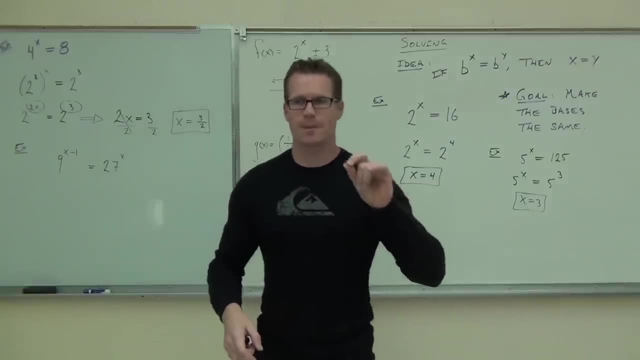 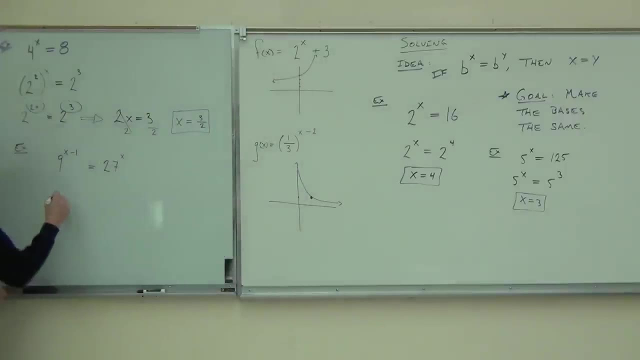 3. Okay, 3.. So now I want you, on your paper, to translate 9 into a power of 3 and 27 into a power of 3.. Do that for me. What's 9?? 9 to 9 is 3 to what power? 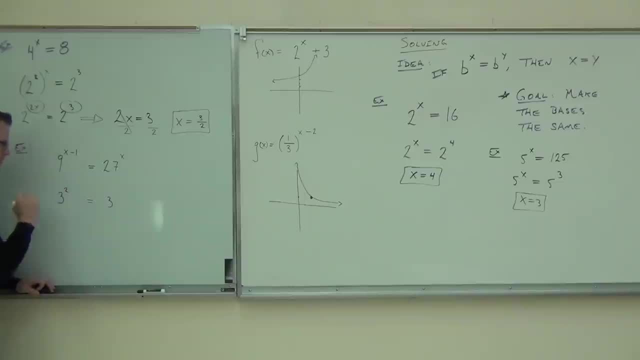 3. 3 to the what 3 times And 27 is 3 to the 3.. Did you make it that far? Yes, Okay, Now, of course, we still have this stuff going on, So watch carefully on this. 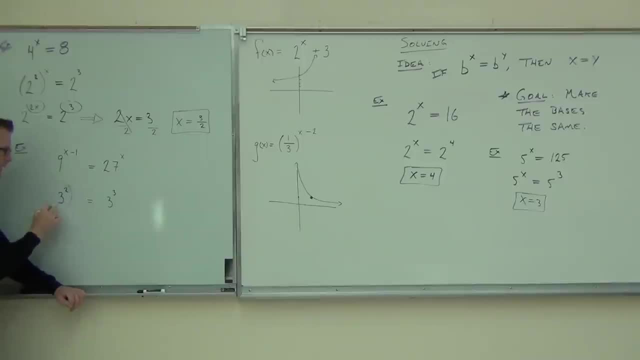 This was just our 9, right? This is still our 9.. So we still have this x minus 1 up there, You with me, And this was 27,. but we still have our x up there. Little head nod if you're still okay. 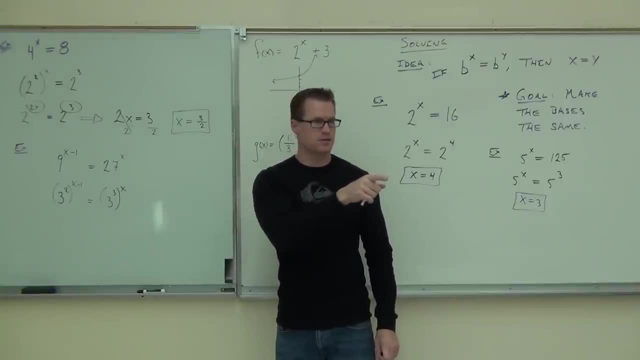 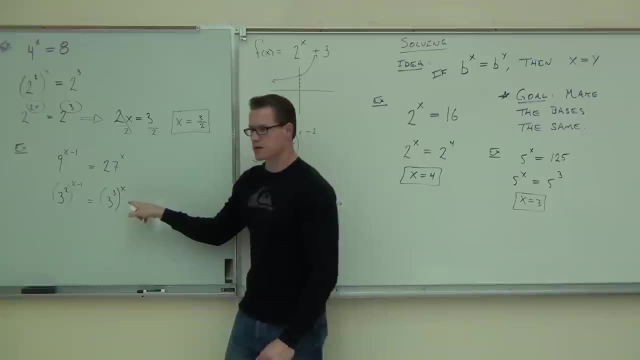 Yes, Yes, I'm here, Yes, Yes, Okay, What do you get? So we're okay getting 3 squared. We're getting 3 to the 3rd. We didn't change this at all yet What do you get when you have a power raised to a power again? 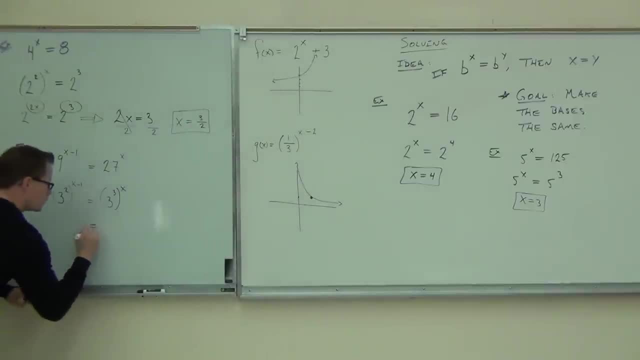 5., 5., 5. 5.. So tell me, on my right-hand side, what I need to have: 3.. 3 to the 3 of x, 3 to the 3 times x. Yes, Not 3 plus x. 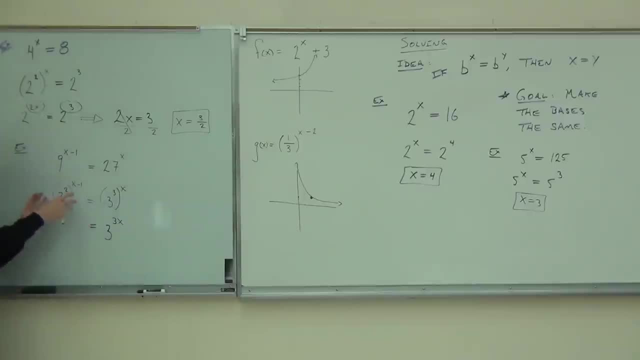 3 times x, We're multiplying those x's Now on the right-hand side. this one's interesting. Take a little bit of time to think about this for a second. We've got 3 squared to the x minus 1.. 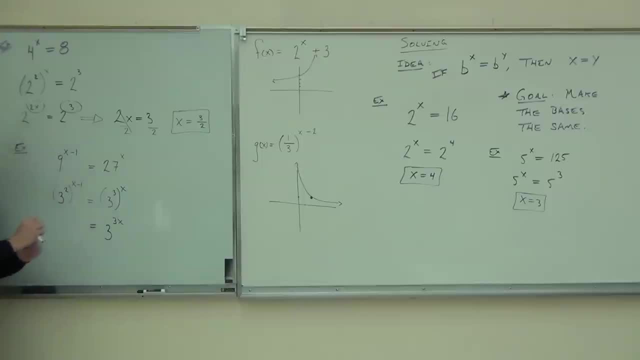 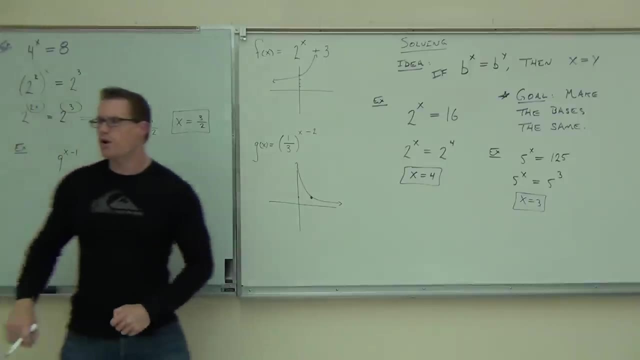 Again, just like this side. what do you do when you have an exponent raised to an exponent? Multiply it, So we're going to have 3.. Do I write it like this? No, No, Write this, Oh no. 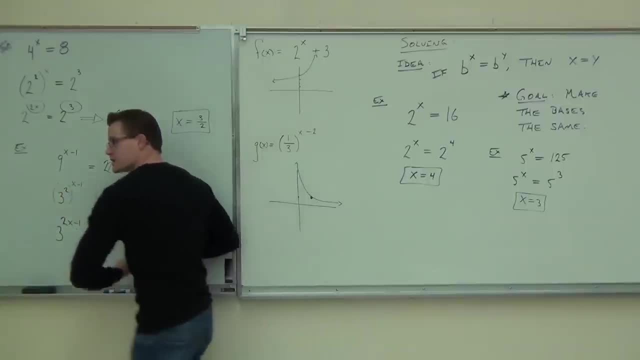 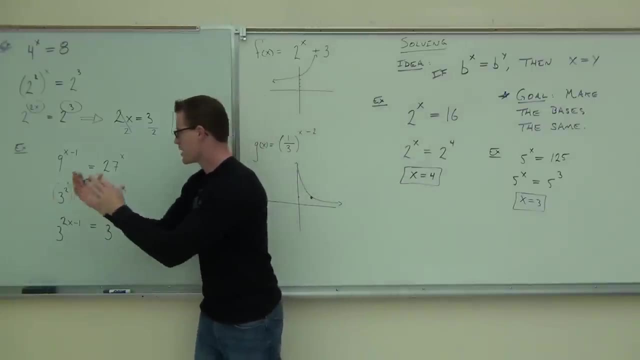 Because this is my entire exponent. right, It really should have some parentheses around the thing. It really should, because that's my exponent. So when I take my 2 and I multiply it by x minus 1, well, wow, you better have some parentheses there. 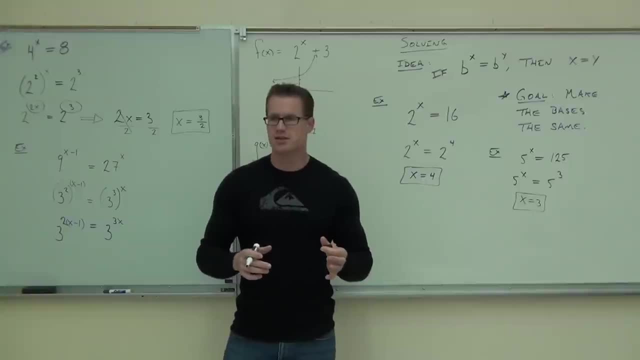 Do you see why the parentheses are important? I think I just said: do you see why them parentheses are important? We're in Alabama. We're in Alabama. We're in Alabama. See why the parentheses are important. You know, when I was 13,. I went around the country with my parents in a motorhome. We spent a lot of time in Texas And Texas is freaking huge. A lot of time in Texas, Louisiana, Alabama and Florida, And when you're 13, you pick up accents very quickly. And by the time we got home I still had an accent for about five years. I still have it. sometimes when I'm talking, I say y'all all the time I'm not, I'm from Clovis. That's weird, It's weird. 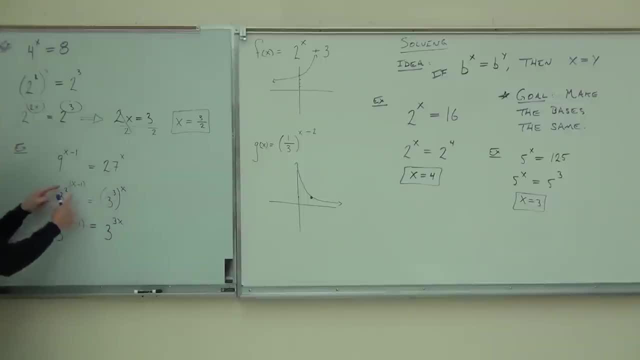 Anyway, we've got 3 to the x, We've got 2 to the x minus 1.. What do you know when your bases are there? They're the same. What do you know about those exponents? Well, look what happens. 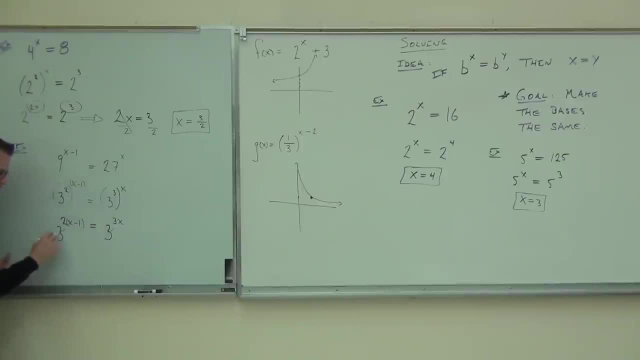 As soon as we get those 3's right here and right here. If you want to cross them out, you can do that. I don't care, But what this comes down to is that now we have an expression: 2 to the x minus 1 equals 3x. 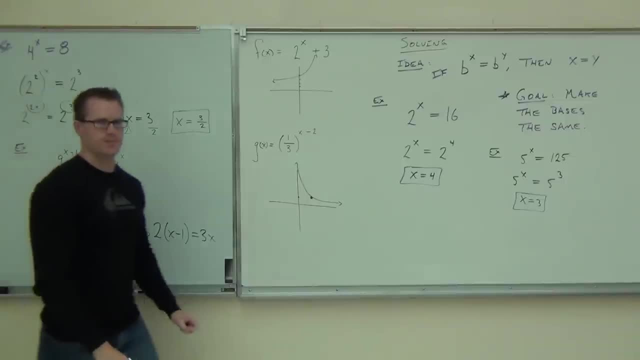 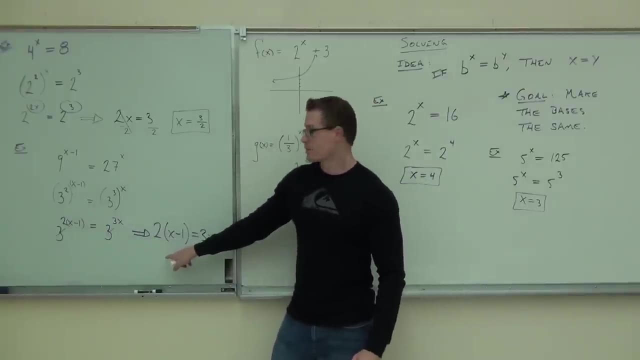 We have this exponent. That's an exponent Equals that exponent. Do you see how we're getting from here to here? Do you see how we're getting from here to here? That's kind of an important one. You know what people always do. 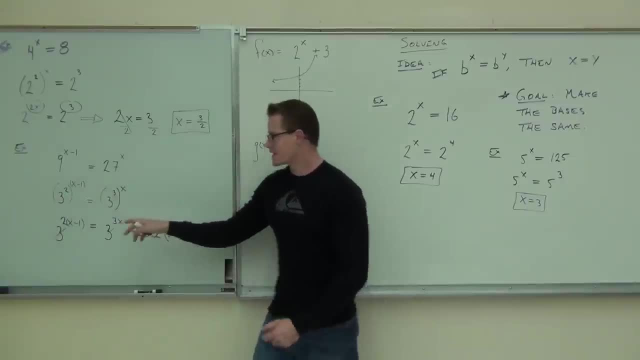 They always give me 2x minus 1.. They forget to distribute that. That's why I'm having you write the parentheses. write the parentheses and wait until this step to distribute. That way you don't forget to do that, You with me. 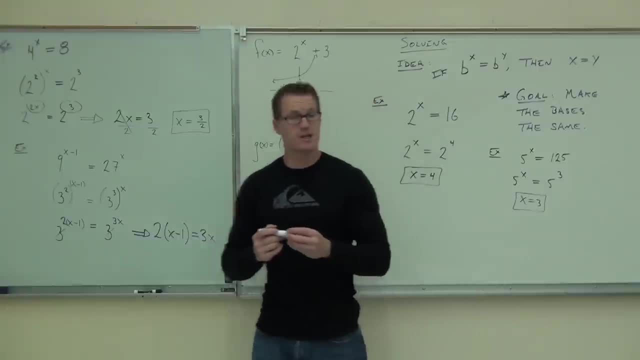 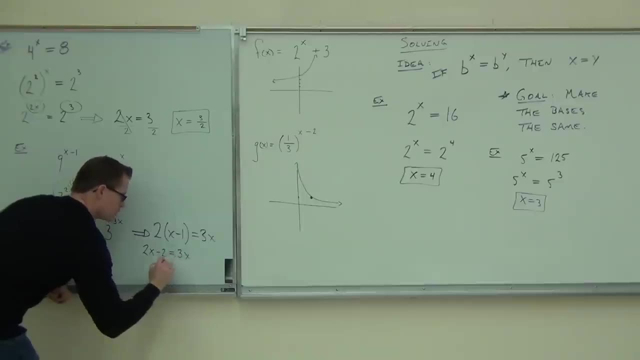 Can you solve that? Sure, That's a basic equation. I mean, that's pretty easy, Of course. you're going to distribute, You're going to get 2x minus 2 equals 3x. We'll distribute that 2.. 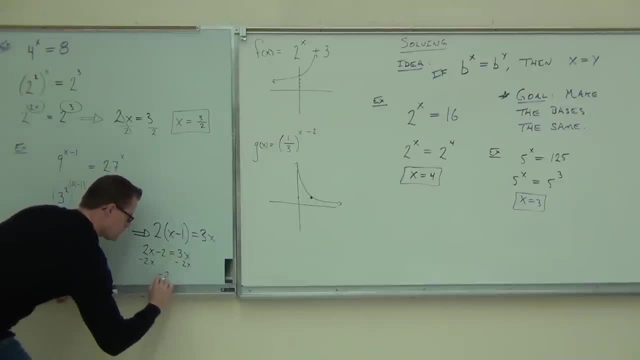 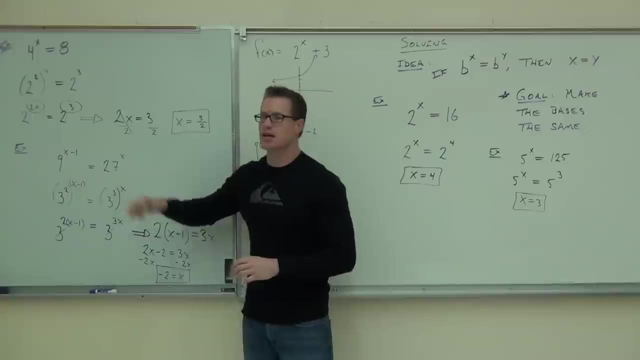 You'll subtract 2x, That's equal to 2.. Negative 2 equals x equals negative 2.. You can plug that in and you can check it. It's going to work out for you. Would you raise your hand if you feel okay with this so far? 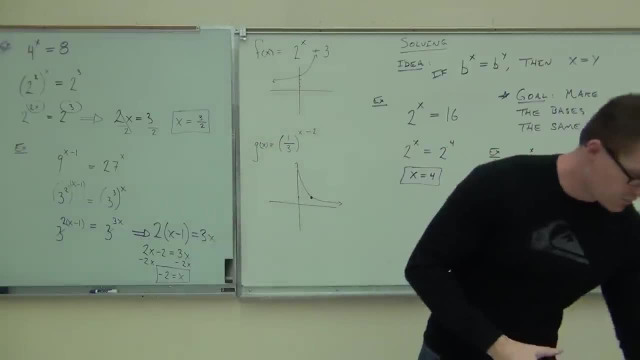 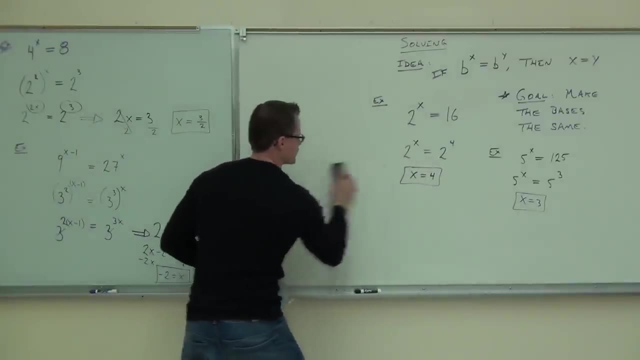 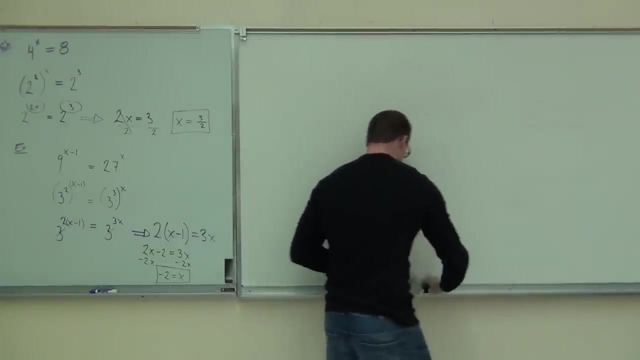 Yes, no, Yeah, You guys over here, Try three of them on your own. We'll move on. Are the two bases always going to be the same? The two bases are not going to be given to you here. They weren't, but you had to bring them. 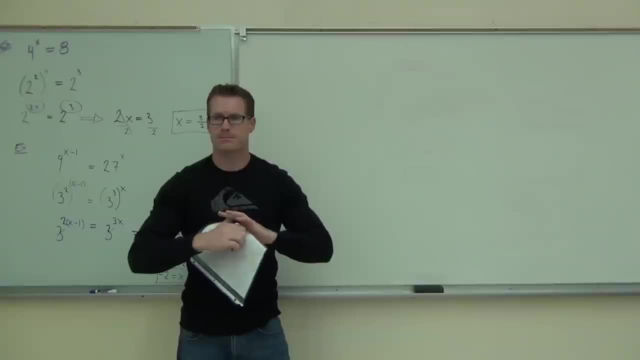 Are you going to have, like the bulk numbers? I mean it's not going to be the same all the time. You have to. Yeah, you have exponentially. you have to have those numbers there, So you're going to be given numbers. 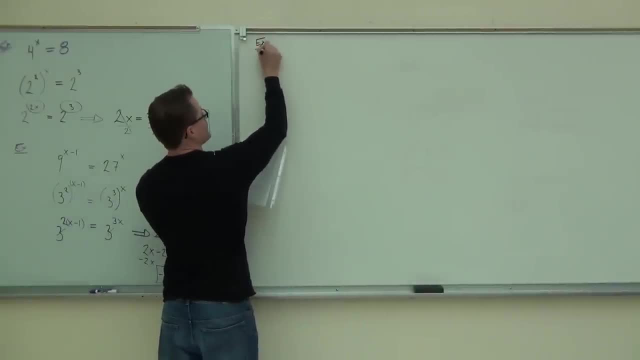 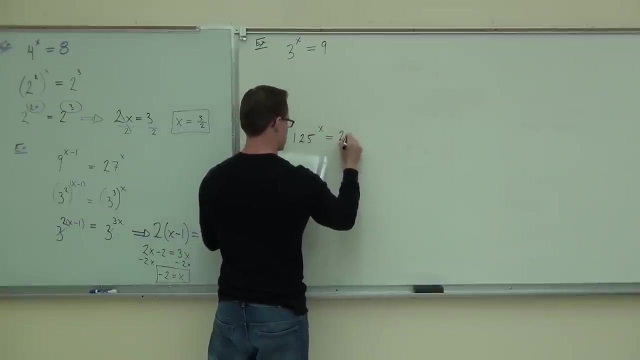 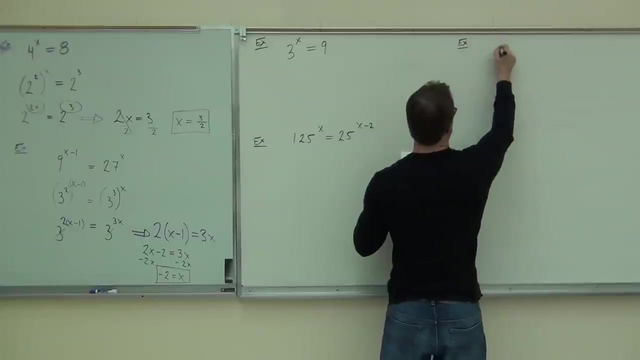 And in this section, your only job is really to find out what number you can find to make them equal bases. That's your only job here. Okay, this last one is a tricky one. You really got to think about that. I'll give you a hint. 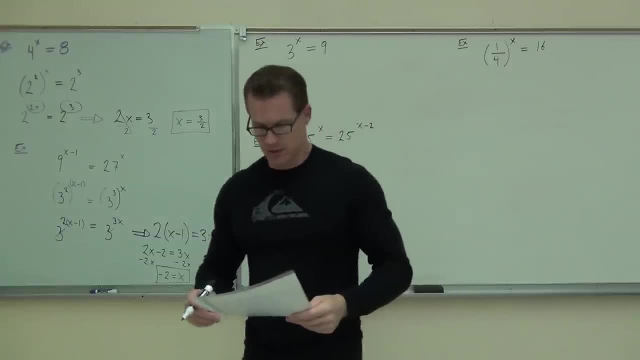 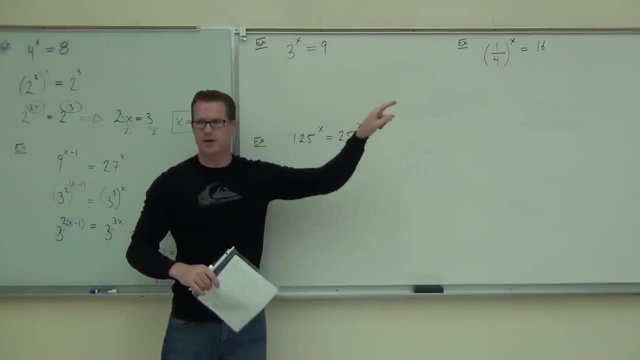 Think about negative exponent. I'll give you a hint for that. So that's a tricky one. So try those ones. I expect you're rock solid on the first two of them. The last one is going to be some. you're going to have to really think on that one. 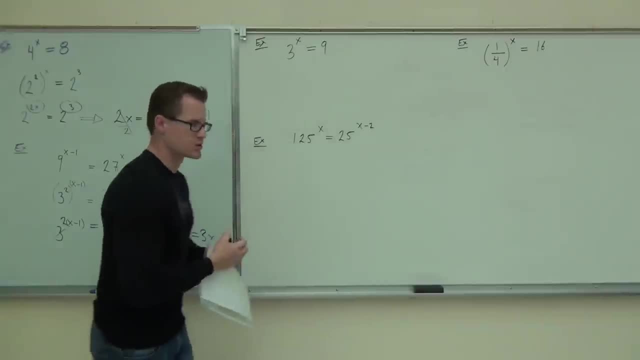 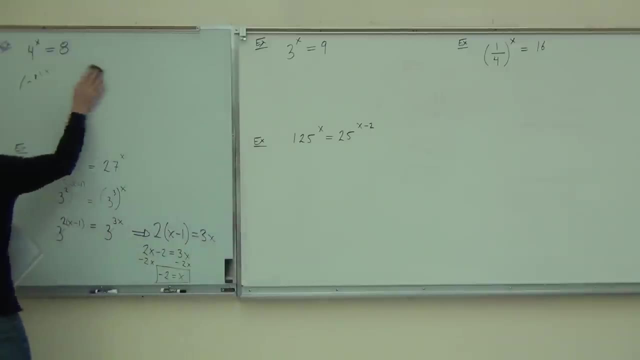 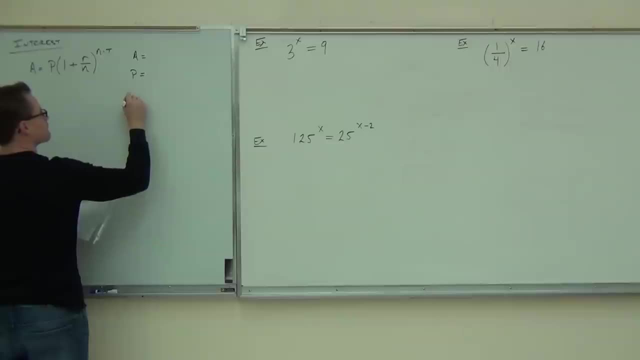 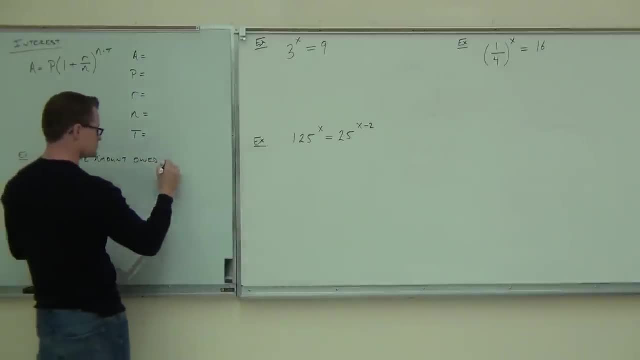 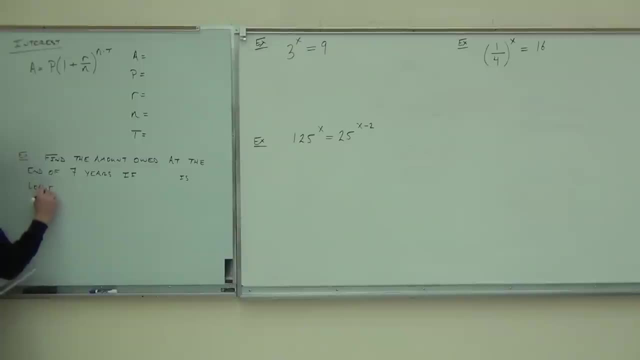 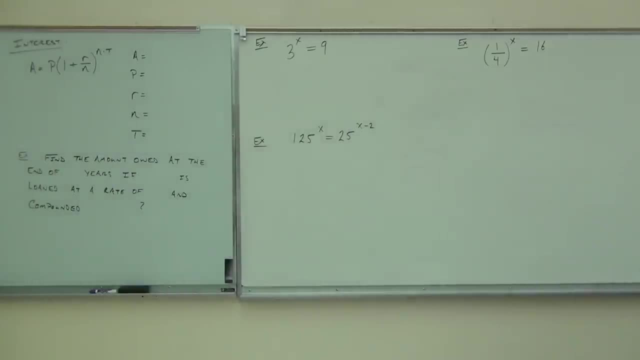 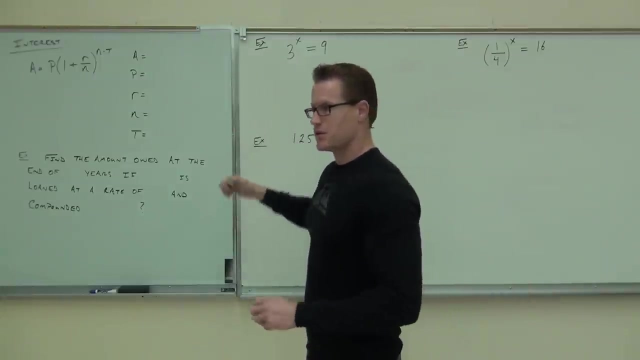 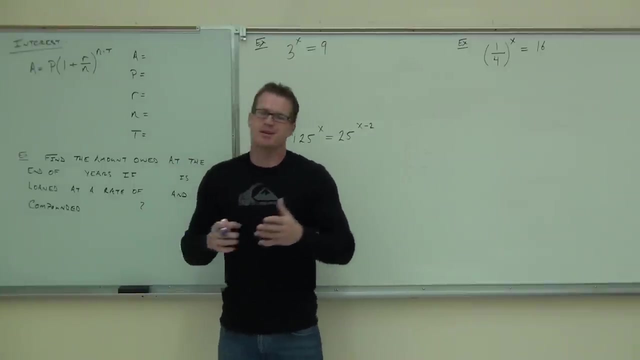 Are you guys done with the first two? Okay, let's go ahead and start the next one. So, first one, some of these you can do in your head. I still want you to show the work, because I mean three of the X equals nine. you're thinking well. 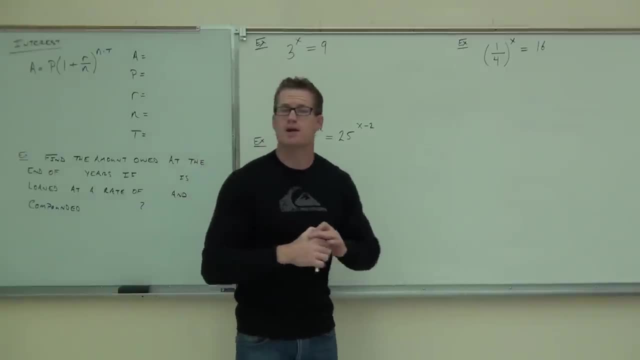 that's obviously a two. right, That's obviously a two. But the idea is get your bases the same, because you probably can't do that one in your head. If you can, well good for you, but that's pretty hard. 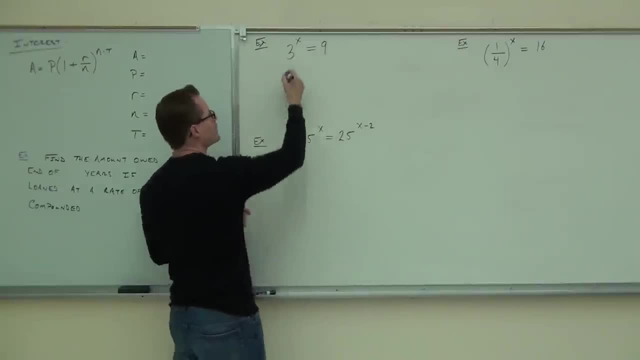 You've got to think about it. It's probably going to take you longer to do it in your head than actually work it out. So here we go. okay, I know I can do three to the X equals three squared, because I'm going to try. 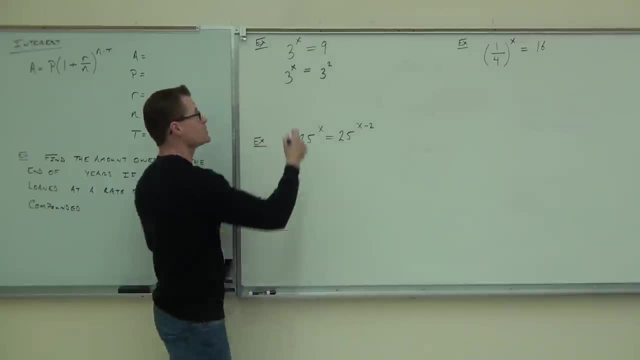 to write nine as a base of three. I need my bases equal. But as soon as you have those bases equal, you also know your X ones are equal. Set them equal. If you don't have to do any more work, you're done. 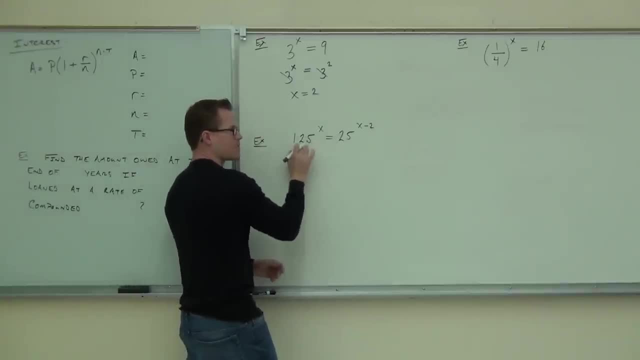 If you do like the next example here. well, I know that I can't write this as 25 to any power, but I can write them both as five to some power. This one we did earlier in the day, That's five to the third, then to the X. 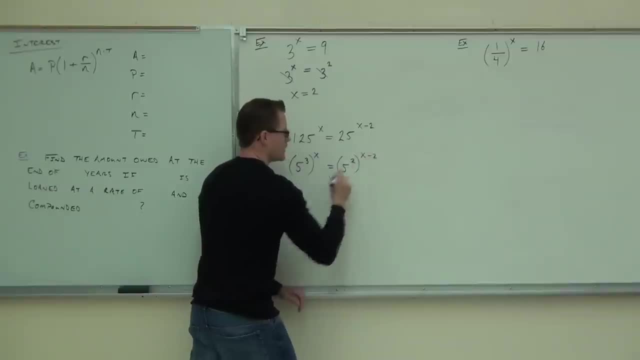 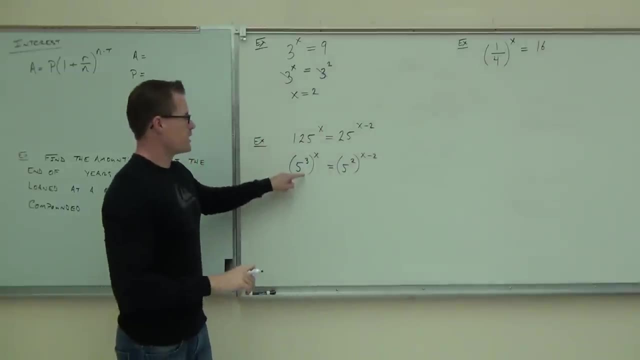 This is five to the second and then to the X minus two. How many people made it that far? Good for you, That's good, okay. So 125 is five to the third. 25 is five squared. We haven't done anything with those exponents yet. 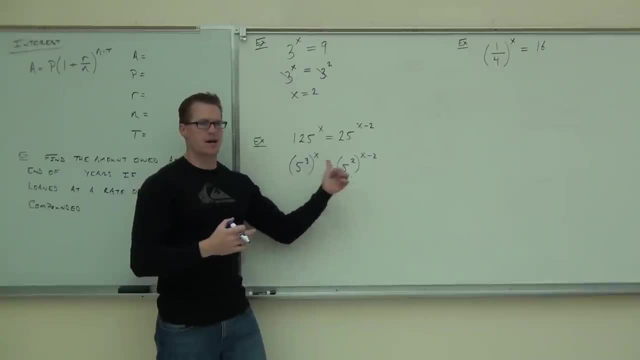 Then your goal is to realize that, well, if I have an exponent raised to an exponent, that means I'm going to multiply it. So instead of five to the third to the X, I've got five to the. is it three plus or three times X? 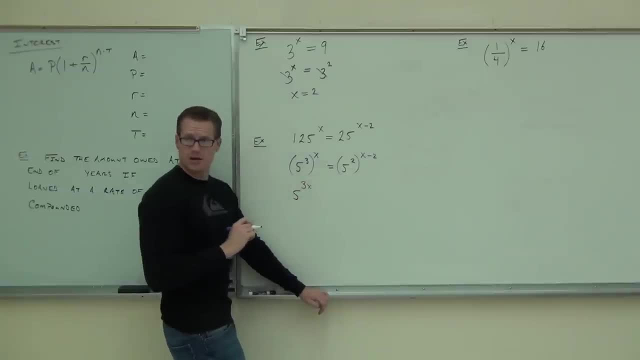 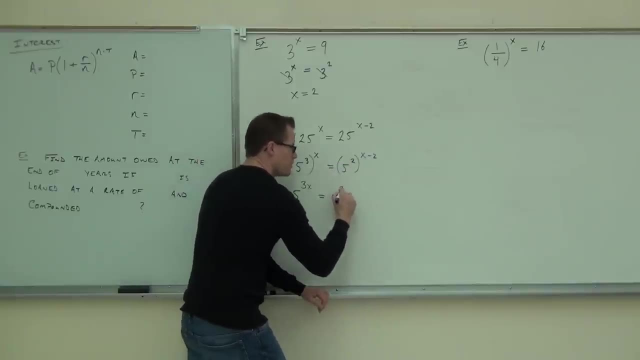 Two plus three times. So that would be three X. Did you get three X? No Equals on the other side. I've got five to the. I have a two being raised to the exponent, but it should be like this: two to the X minus two. 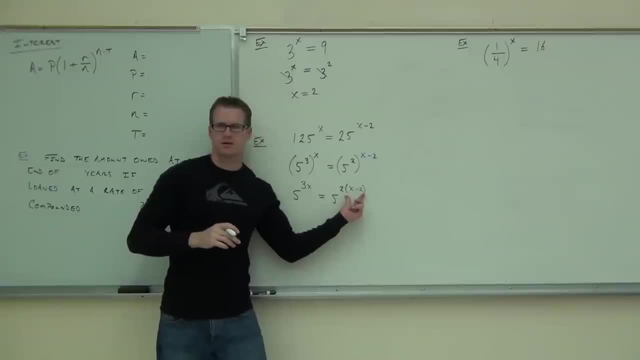 Two to the X minus two. Why do I have parentheses right there? Multiply- We're multiplying by the entire exponent. We have to do that. But as soon as you have those bases, the same, notice how our five and our five are the same exact base. 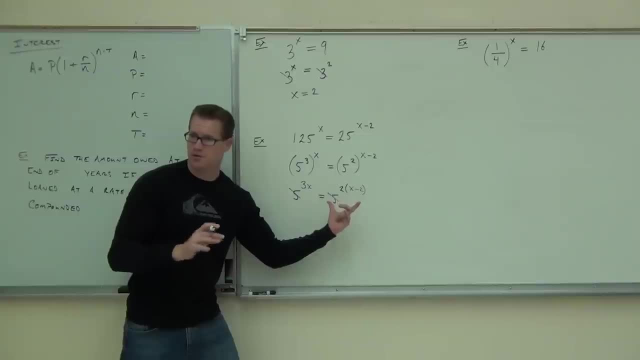 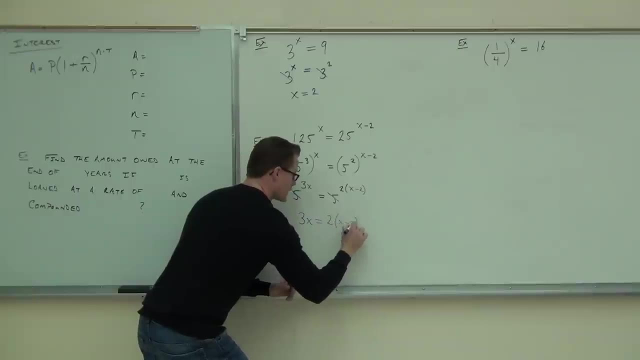 in this case. That's why we did this work, to get down to the five equals five as far as our bases. Then you can set your exponents equal to each other: Three X equals two X minus two. of course, we'll distribute. 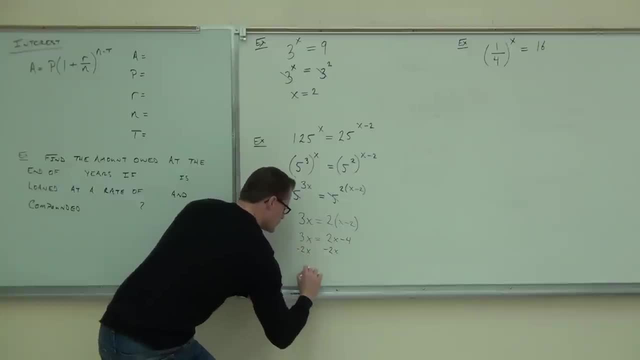 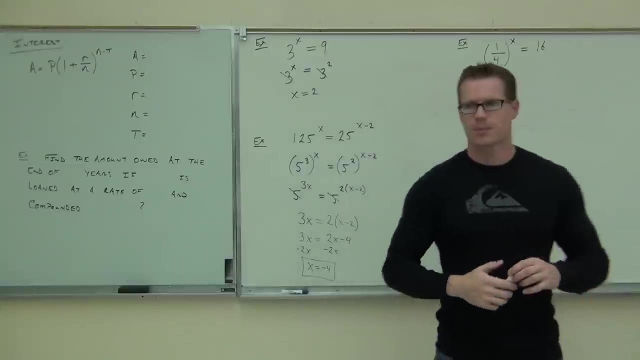 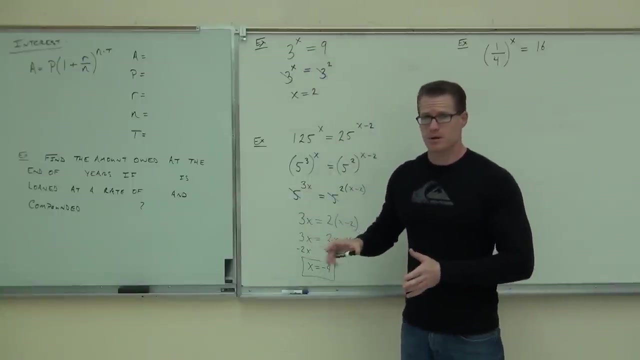 Subtract two X, X equals negative four. So again the whole goal. here the whole goal: try to make your bases the same As soon as you get them the same, take your exponents and multiply them, because you have an exponent raised. 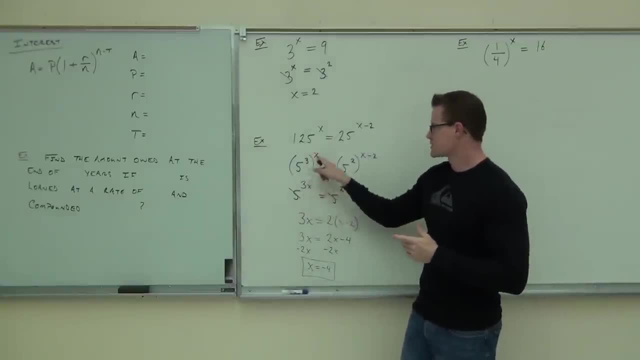 to an exponent. that's what exponents do. So multiply three times X and two times X minus two. You might have to distribute there, then solve it with a basic equation, because now your bases will be the same. You set your exponents equal work all the way down. 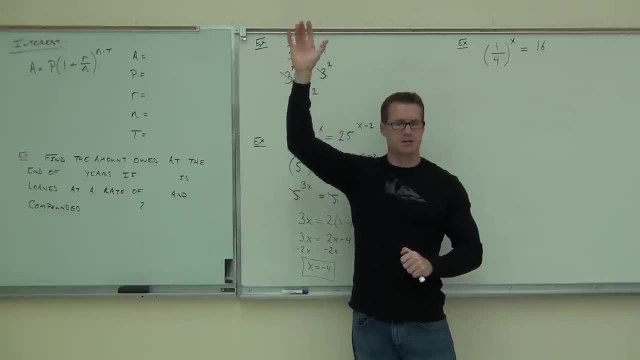 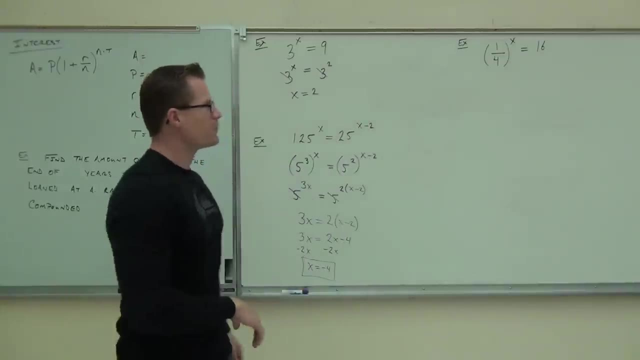 I'm going to feel okay with what we talked about: the idea, at least the idea. Okay. Now the last one, the last one's tricky. Last one's tricky because you look at that, you go: I've got one-fourth to the X, I've got 16.. 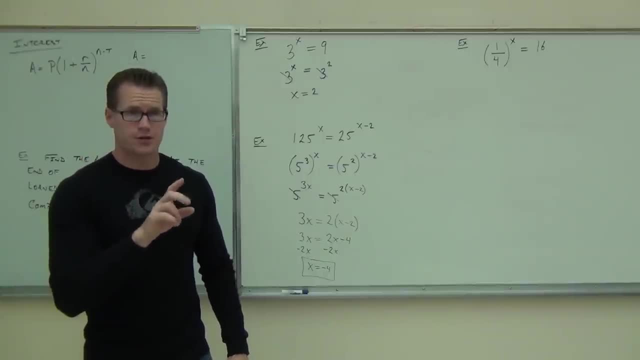 Now you do have a couple options here. The first option: you could use a four. You could use a four as your common base, or you could use a two as your common base. Are you with me on that? You have options here that will both work. 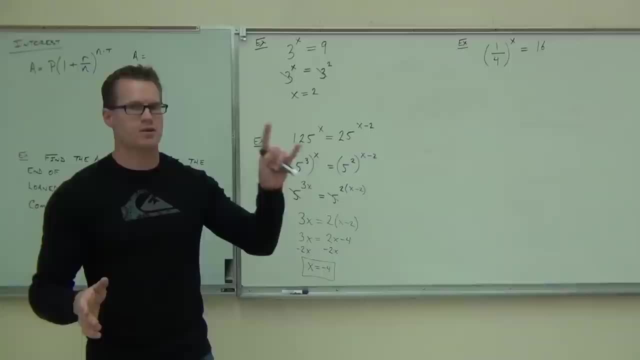 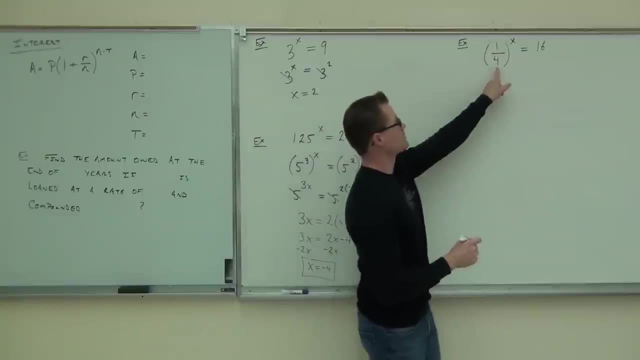 They will both work. I'm going to show you the two version because I want you to be able to do other problems besides just this one type. Okay, Here's the version using two as a common base. First thing, do you see that two is a base? 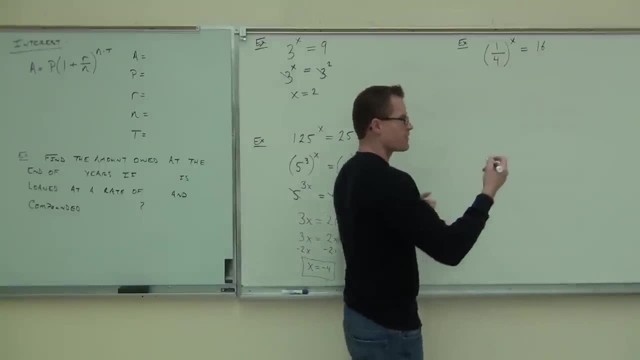 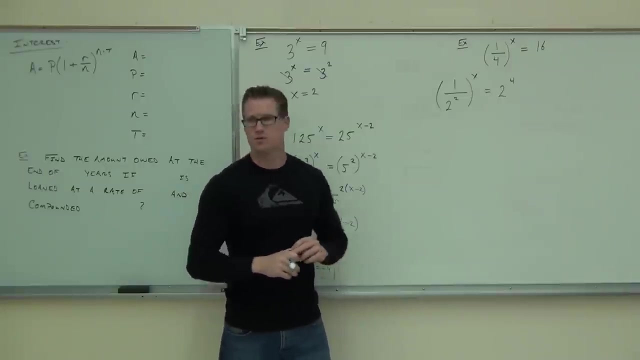 between this and that number. Well, do me a favor. Write it like: one over two, squared to the X, equals two to the fourth. Is that okay with you? Yes, no, That's still one-fourth, That's still two. 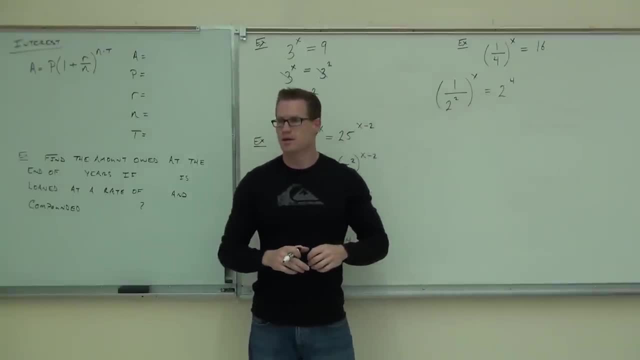 I'm sorry, That's still 16.. Two to the fourth is still 16.. Yes, no, Now I gave you a hint. I said: think about negative X squared. Think about negative X squared. I said, think about negative X squared. 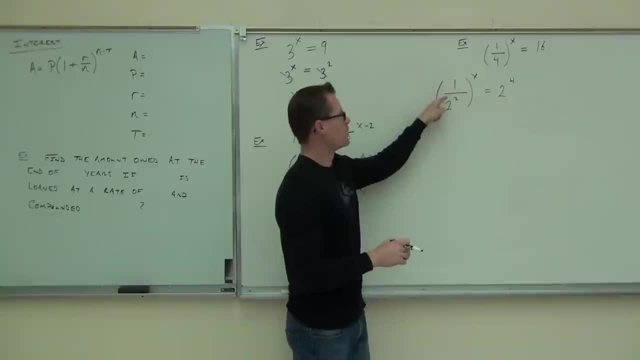 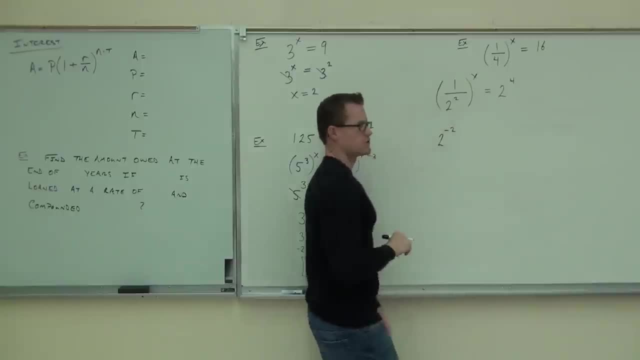 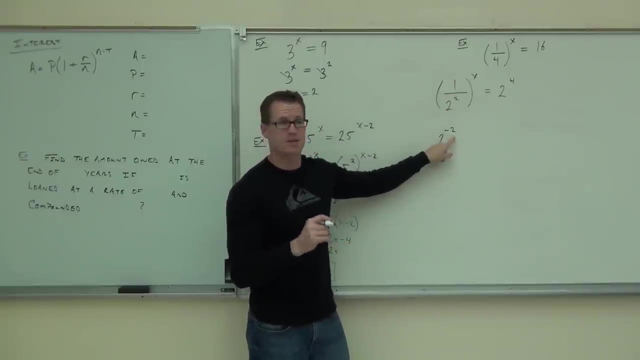 this is the same thing as two to the negative, two power. Do you see that if I move that to the top of my fraction, I can change that variable, that exponent, to negative and it means the same thing. You with me on that. 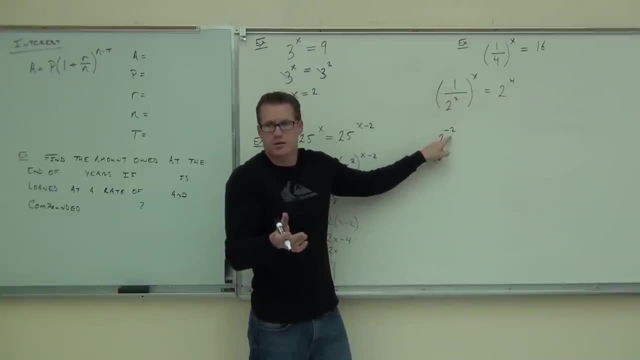 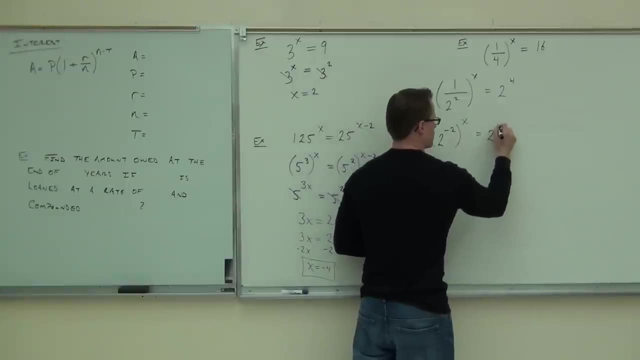 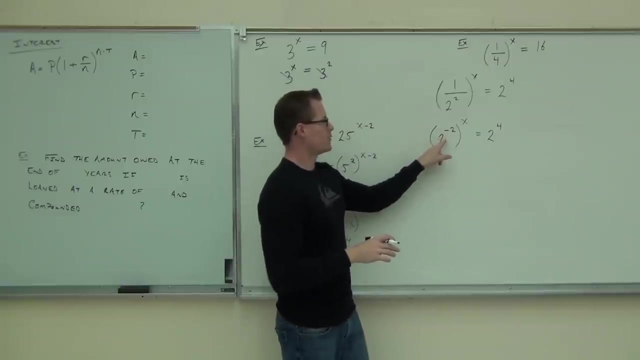 You could go from here to here, couldn't you? That is one over two squared, That's what that is. So go in reverse, Hey. hey, now we have something we might be able to work with. In our case, up here we'll have exponents raised to exponents. 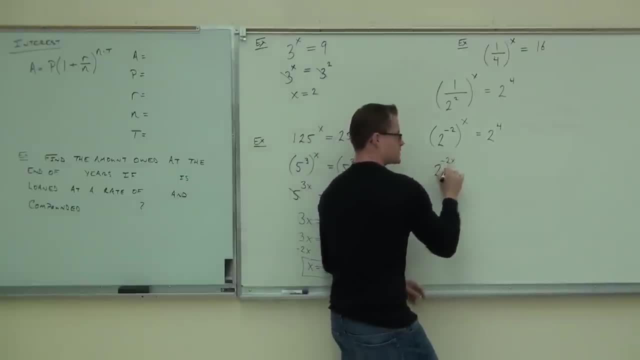 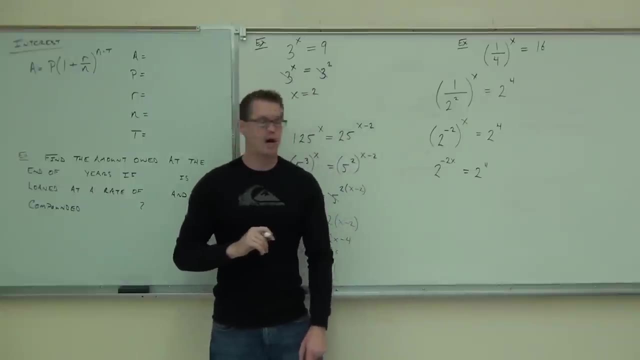 We'll multiply. You're going to get two to the negative two X. See where the negative two X is coming from. You're multiplying there Equals two to the fourth. Do you have common bases now? Yeah, Set your exponents equal to each other. 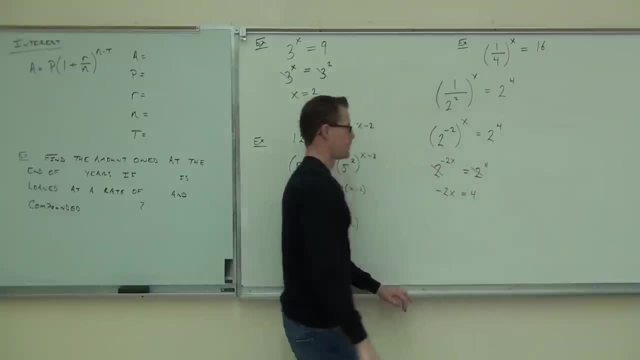 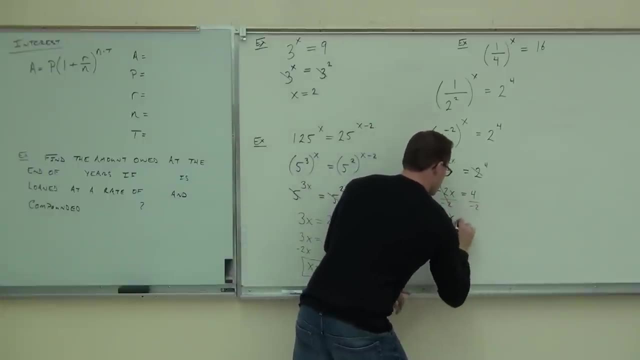 We've got negative two. X equals four. What are you going to do to get rid of that negative two? Divide, All right. If we divide by negative two, You get X equals negative two. So when you're faced with those fractions, don't just give up. 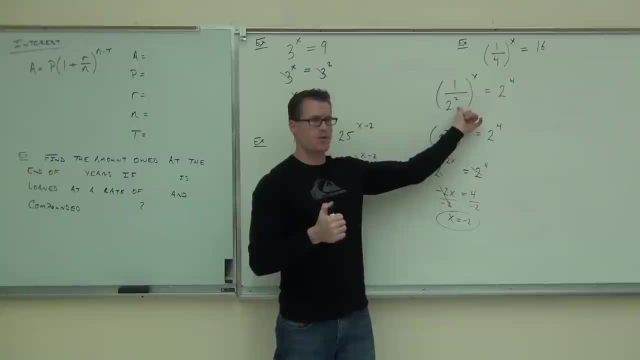 Do the same thing. Only when you have something on the bottom your denominator of a fraction, make it a negative exponent, Move it to the top of your fraction. Could you guys follow that one? That's a little trickier but it's possible for you. 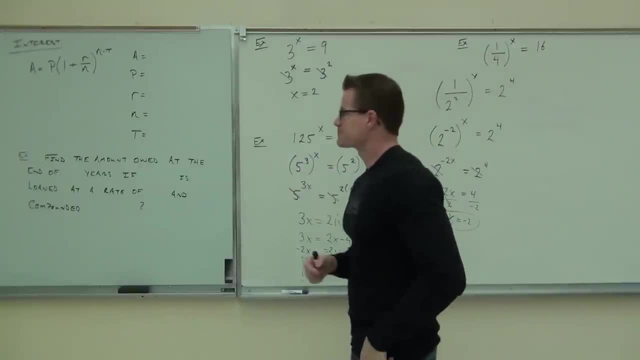 Now, the last thing we'll talk about in this section is something called interest. Have you guys ever bought anything on credit? Yes, No. Do you have a credit card? How many people have one? I don't have a credit card. 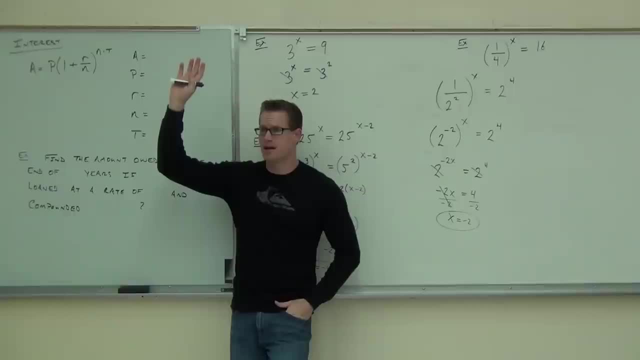 I don't have one, Then you've bought something. You've probably paid a little bit of interest, right? Unless you pay off your statement every month, you pay interest. Now I try to pay off my statement every month because I hate paying interest. 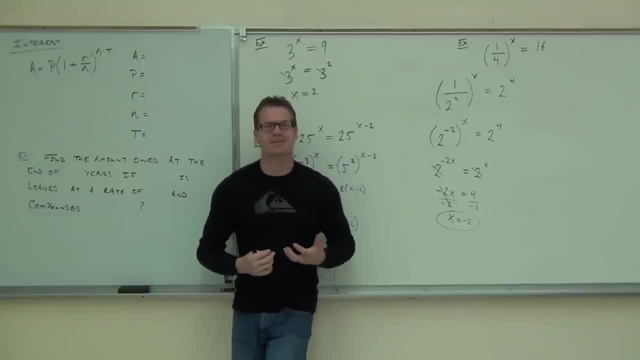 That's giving away your money, right, Just for the sake of getting it sooner, because you want it now, Right? Everyone does this, though People buy cars without all the money because cars are expensive. You ever bought a car before? Oh my gosh. They're ridiculous. All right, You pay $25,000 for a car you drive for a lot and it loses $5,000 just like that, Just from driving it, Driving it off the lot, you lose like I don't know what percentage of the money it is. 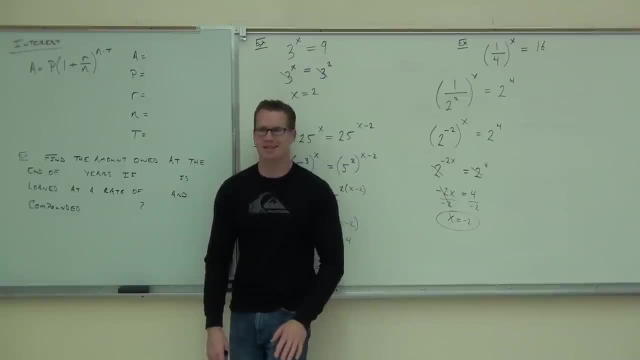 That would be one-fifth 20% of it, but it's not that much right off the bat. Anyway, you're losing some of that value, but if you buy the car without all the money you're going to pay interest. 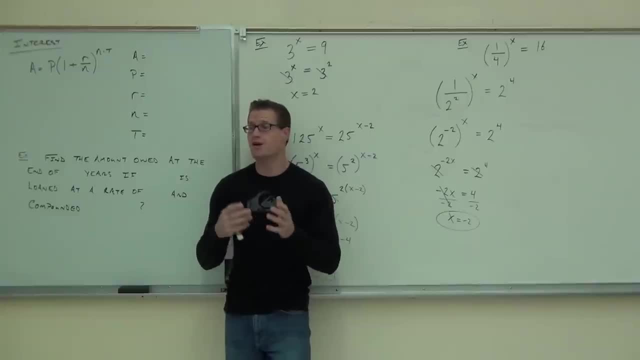 You ever read those ads? 2% financing, 5% financing on your vehicle. If you buy a house, everyone has mortgages right, now, right, And you have interest rate for your house. That means every month you pay a little bit of interest so that you can live in this place. 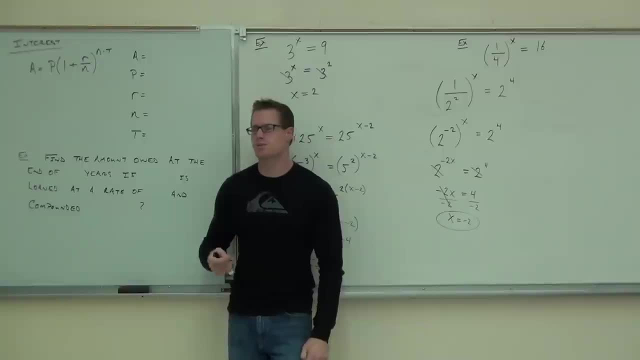 Because you borrowed the money from the bank. We're going to figure out how to do something called compound interest. Here's what compound interest does. Compound interest can work for you or against you. Do you guys have bank accounts? Yes, Yes. 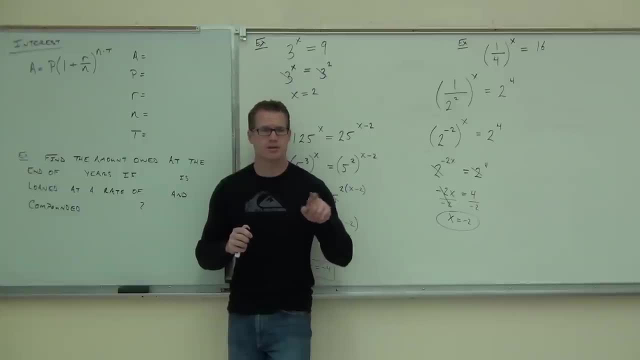 Do you have money in your bank account? Yes, What's your account number? Just kidding. But in your bank account you get a little bit of interest each month, don't you? You ever look at your statement? It says at the very end: oh, you made .01 cents this month. 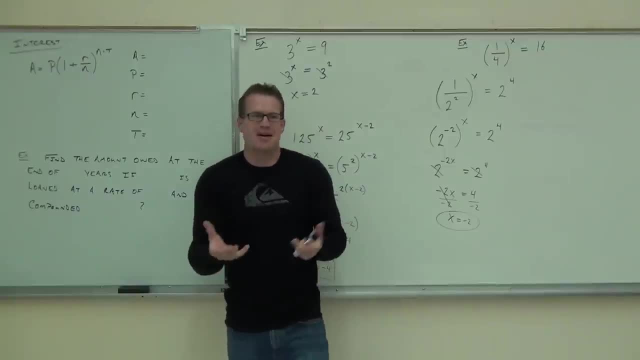 Congratulations. You have no more interest. You have no money, right? So even if you have a lot of money, the interest isn't very great. You get like maybe 10 cents a month because they say: well, here's your reward for saving your money with us. 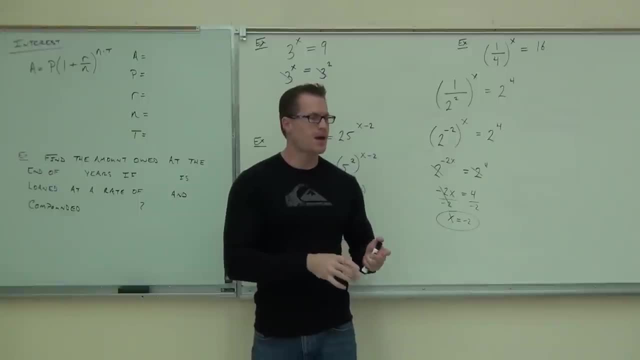 We're going to give you a percentage of your money. That's called interest, And here's how compound interest works. Let's say you start. let's do a very optimistic example. Let's say you start with $1,000 in the bank. 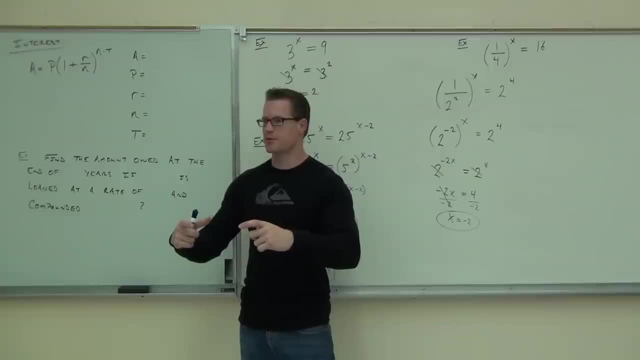 You with me And let's say your interest is compounded monthly. At the very end of the month they're going to say, oh, we're going to give you a percentage of that money. Let's say, we give you a dollar. 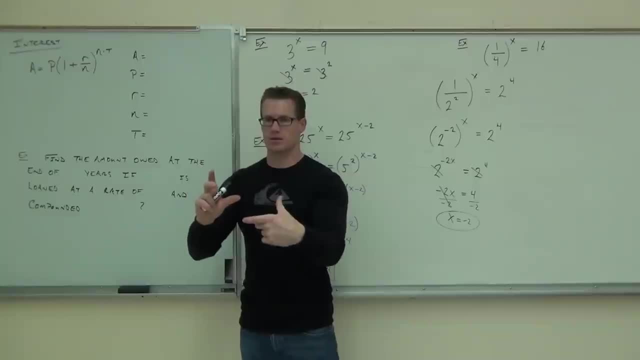 That would be a pretty good interest rate right now. So let's say we'll give you a dollar for having $1,000 in the bank. Well, at the end of the month then you're going to have $1,001. 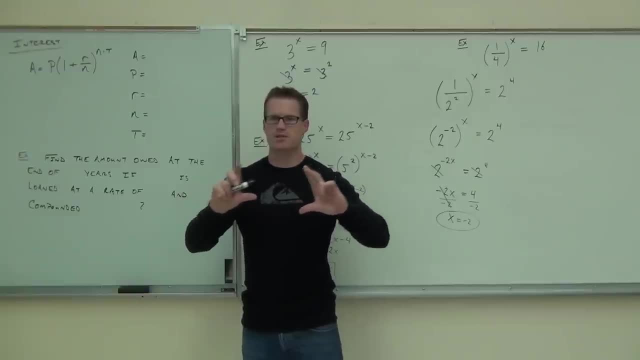 True, If you don't put any other money, you don't take anything out. you're going to have $1,001 at the end of the next month. Do you agree? They're going to give you interest on $1,001.. 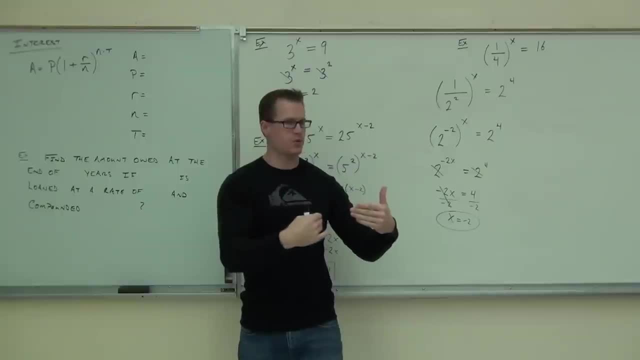 So they're going to give you interest on top of what they just paid you for it. That's called compounding. So they're adding interest to your interest, So they add it to your account, then you get interest on that amount. Then it knocks you up a little bit. 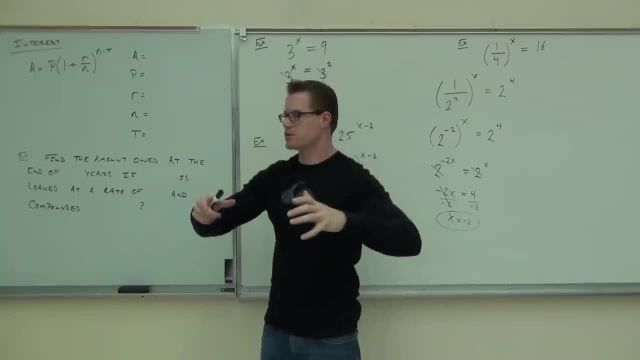 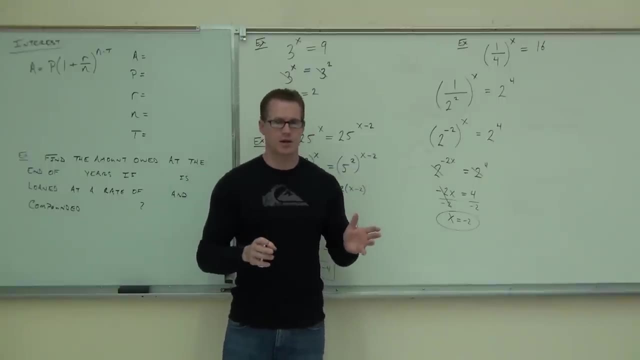 Then you get interest on that for the next month. That's being compounded. Do you understand the idea of compound interest? Same thing with the credit card. okay, Let's say you bought something for $10,000 and you don't pay anything. 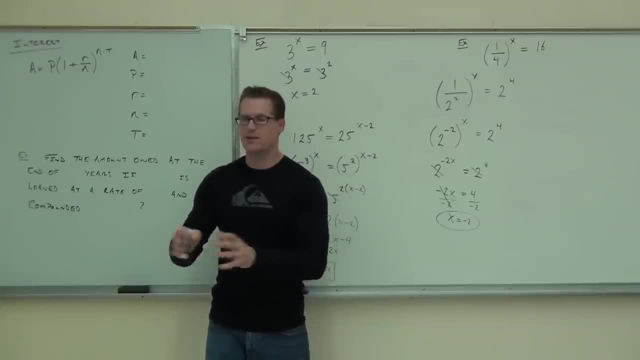 They're going to charge you interest on that- that $10,000- at the end of the month. Then the next month you'll get charged not only for the $10,000, but the $10,000 plus the interest they tacked on there. 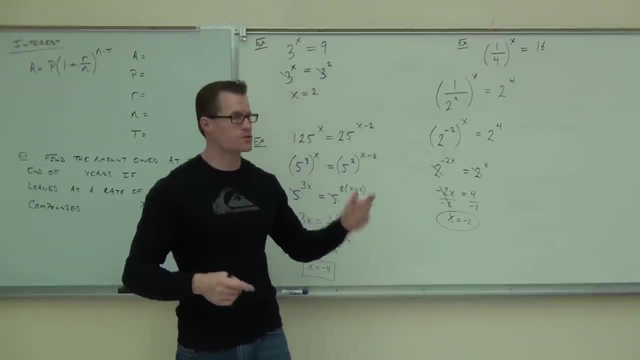 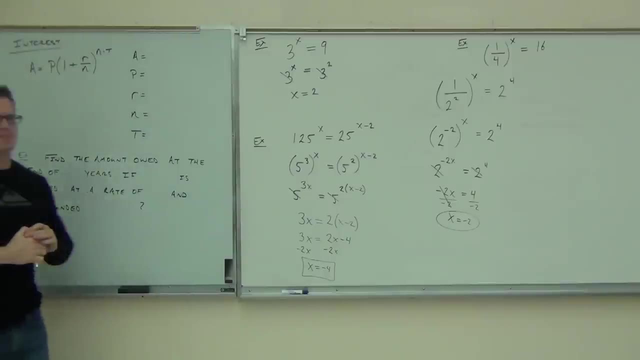 And it's going to keep going. It's going to keep building very, very, very fast. That's compound interest. Now, how we use this is this formula up here. You need to know what the letters stand for. The letter A stands for the amount that you're going to have in your bank account. 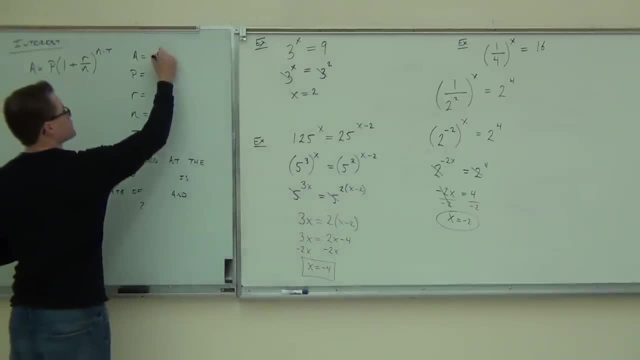 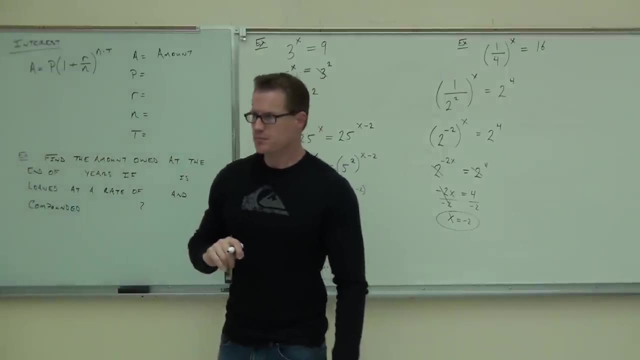 or the amount that you're going to owe after a certain amount of time. So this is your amount P. that letter P stands for principal, Not principal like the guy- okay, Not the guy- that gets you in trouble in high school, or something. 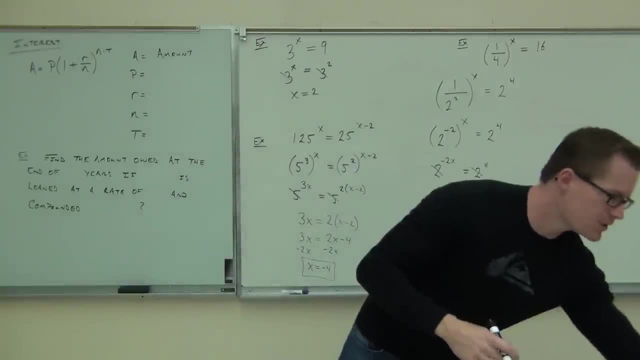 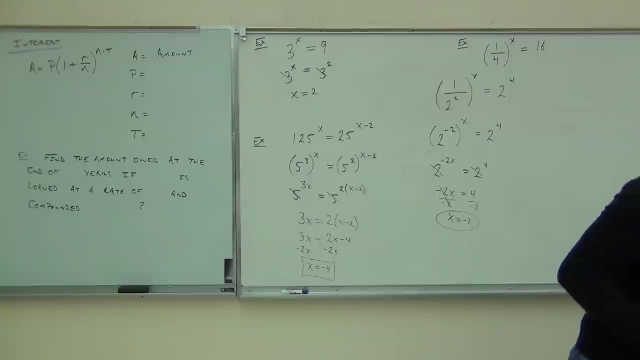 Not that type of principal. Principal like this is the principal. This is the principal. This is the amount that you put into the bank at the beginning or the origination of your loan. So it's the amount that you're borrowing or the amount that you want to save. 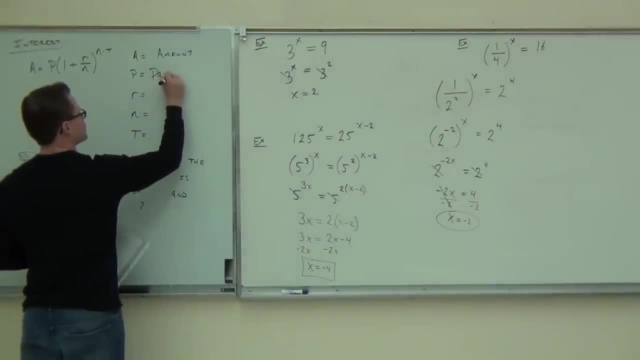 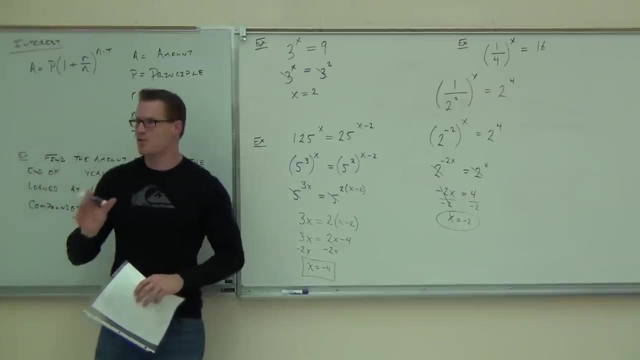 That's what you start with Now. I always misspell principal, so I hope that one's right for you. It's either A-L or L-E, I can never remember. I think it's the L-E, I'm pretty sure. 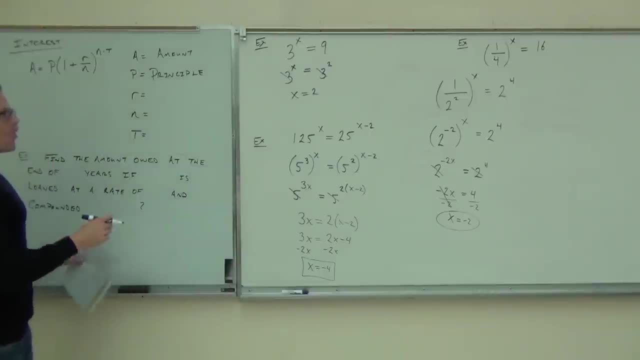 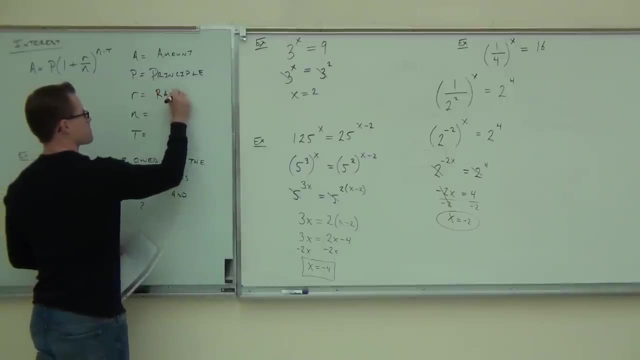 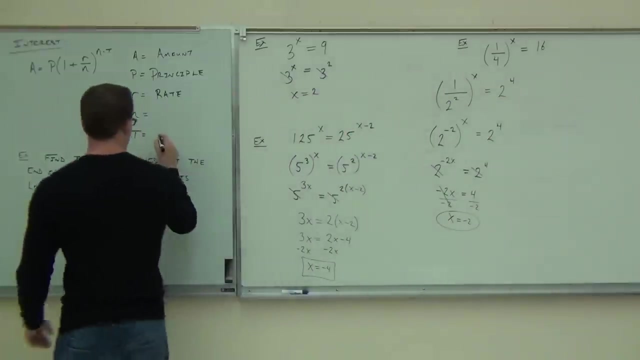 Yes, Okay, good, I pass R. R stands for your interest rate. It's going to be in a percentage. N is an interesting one. T is pretty easy. T is the time in years, The years you're going to have that loan or the years you're going to have your money. 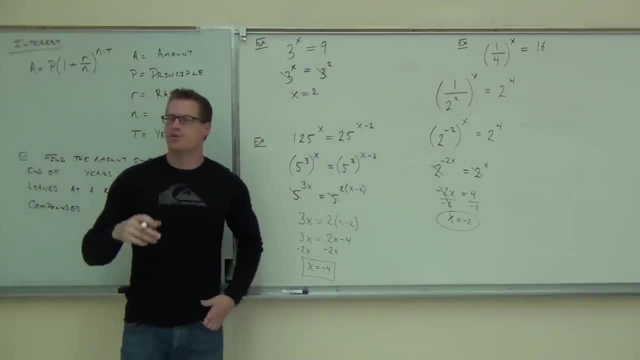 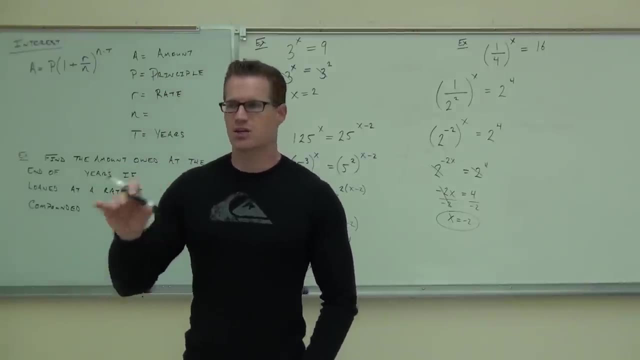 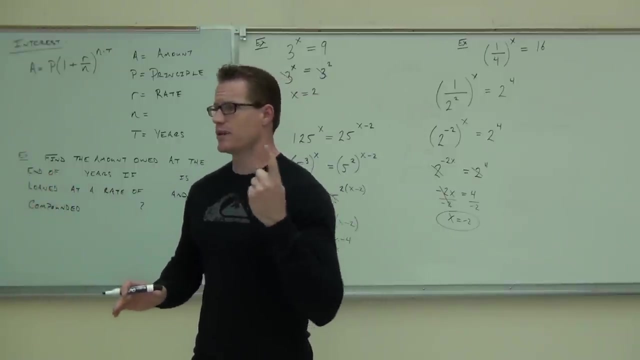 in the bank without touching it. N. N is the number of compounds per year. So let's imagine this for a second. If I say it's compounded annually, how many times is it compounded per year? Annually means once. Semi-annually would mean twice. 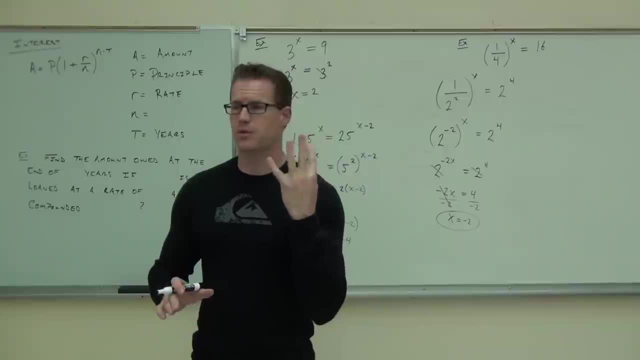 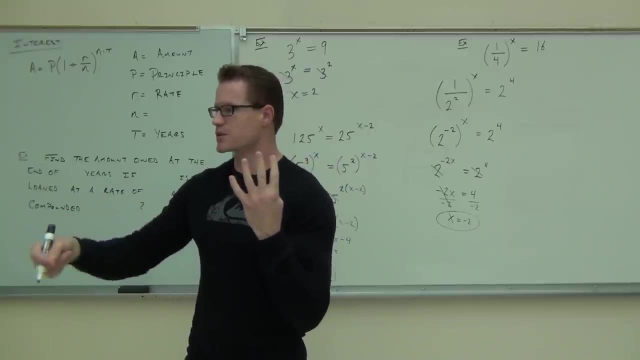 Quarterly would mean how many times Monthly would be how many There's 12 months in a year. What if I said weekly How many weeks are there in a year? It would be compounded 52 times How many days are there in a year. 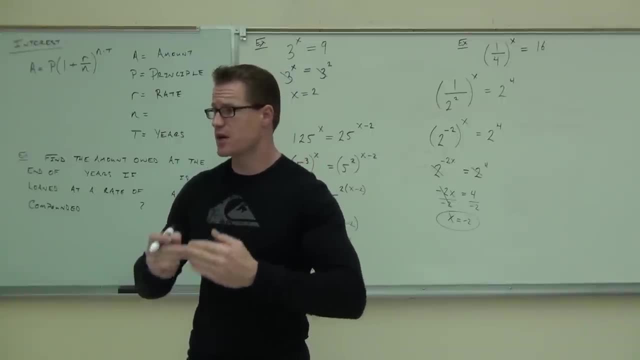 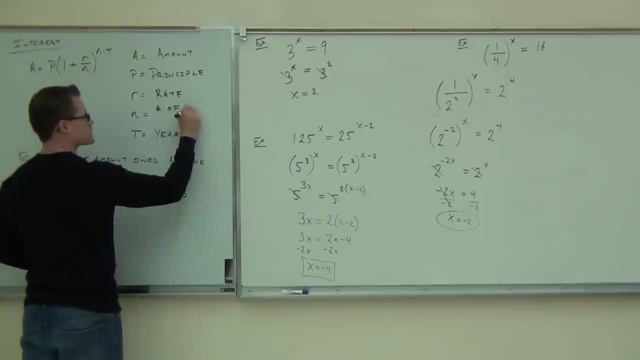 So if I said daily, it would be compounded 365 times every year- You with me. So the number of compounds. Now you're going to need a calculator for this, because you're not going to be able to do this in your head. 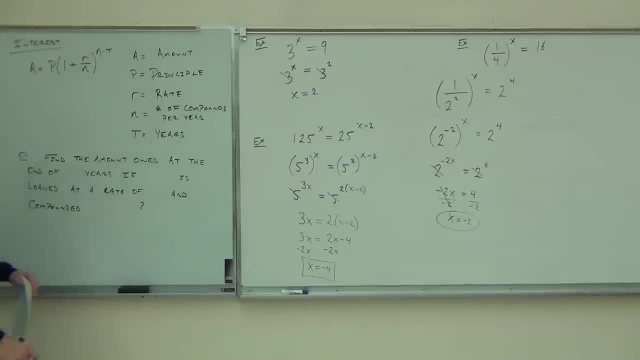 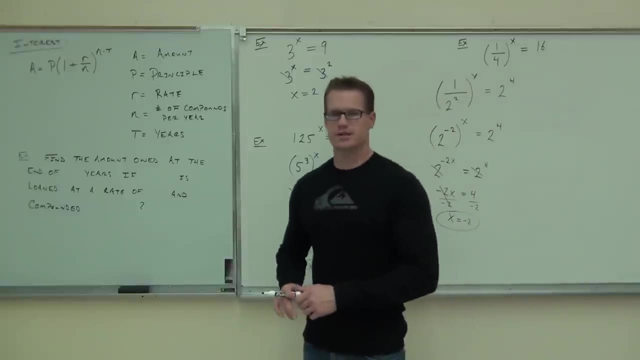 Let's go ahead and make up an example. You're going to buy a, let's say, a cheap car, All right. you're going to buy a used car up here. How many years do you want your loan? for Six years. Six years? Great, That's too much. Six years, Six years, That's too much. If, how much do you want to buy a car for Forty, Forty thousand dollars, Are you crazy? Okay, Thirty, thirty-four. 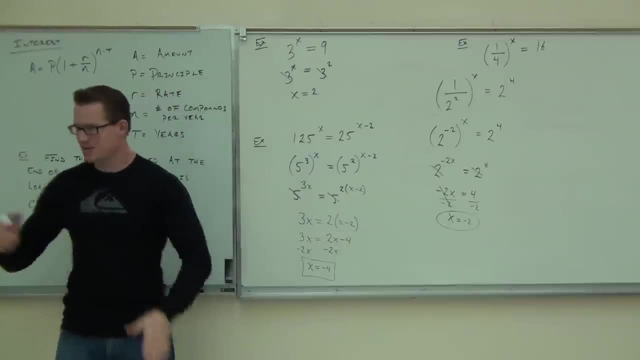 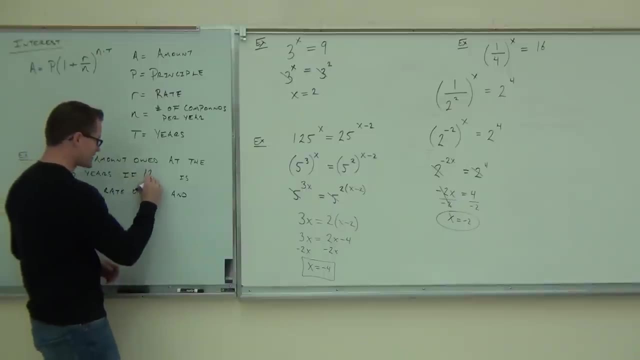 I said: a cheap car. Oh, twenty, Twelve, Twelve, Okay, Twelve thousand, That's a cheap car. Hey, I bought my car for seven, five hundred bucks. Oh, I don't think. floors, Oh my gosh. 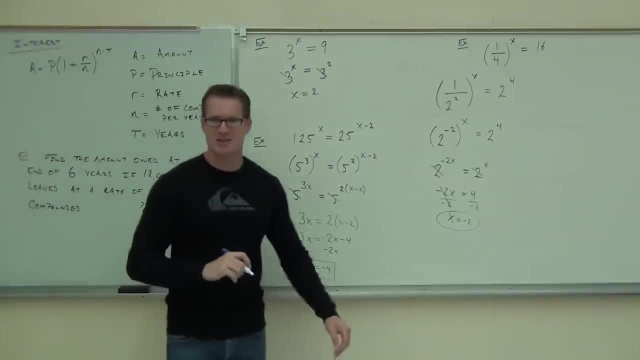 It's got twin turbos. It's zero zero. sixty under five seconds. Get the new one. It'll be the new one. Why It's prettier? It'll be the new one. It'll be the new one. It'll be the new one. 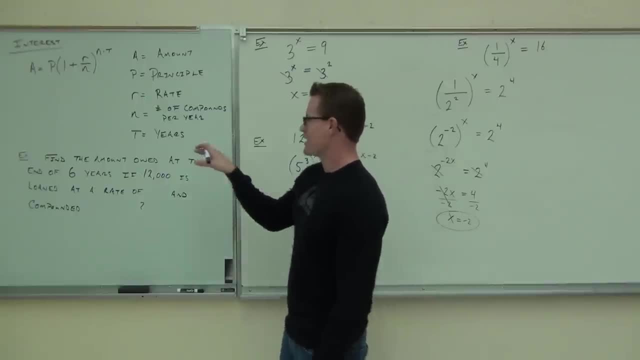 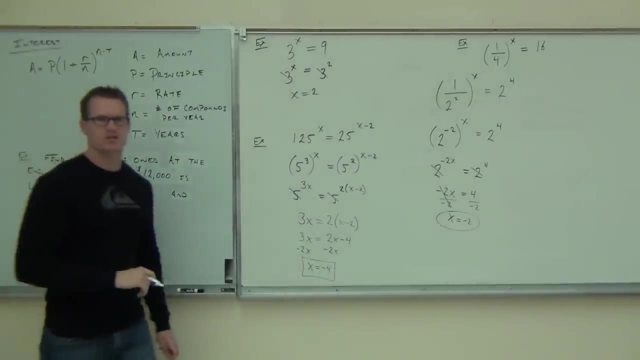 Why It's prettier, It'll be the new one. Okay, So find the amount loaned at the end of six years at twelve thousand dollars. is loaned at a rate of what interest rate do you want to pay Zero? 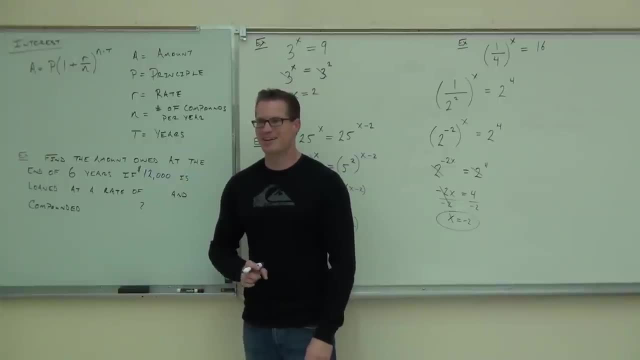 Well, you want to pay zero? Yeah, of course That'd be awesome, But you're not going to pay zero. Why not? Because they ain't going to give you money for free right now. Three, Three, four, nine or something. 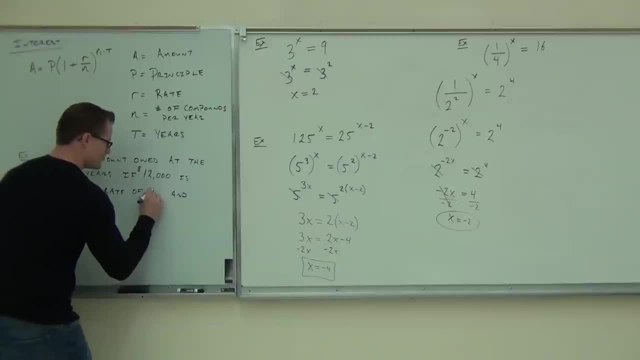 Real estate. Let's do something easy like five. okay, Five percent. Let's say: your credit's not that great, okay, They're not going to give you 2.9% financing, They're going to give you five percent. 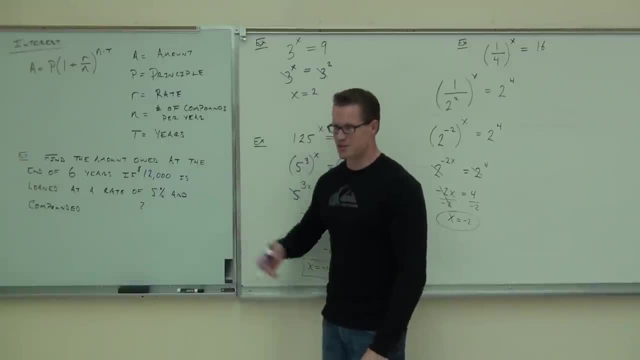 Okay, So they're going to give you five percent Okay. Okay, So they're going to give you five percent, Okay, And you're going to give them a back-up of 225.. Two dollars, Two dollars, Okay. 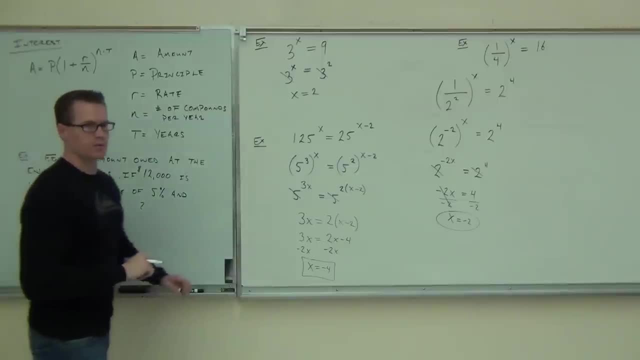 Nibs, Two dollars And one dollar. So if you got aional loan, you're going to give them two percent, Okay, Divided by the% of the interest rate And compounded. usually when you pay auto loans it's compounded monthly. 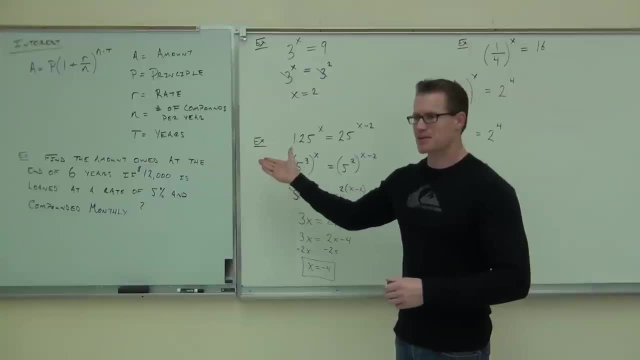 That is how a problem would look. That's how a problem would look On a test. So guess what? Yeah, a problem like that on a test. Find the amount owed at the end of six years at twelve thousand dollars is loaned at a. 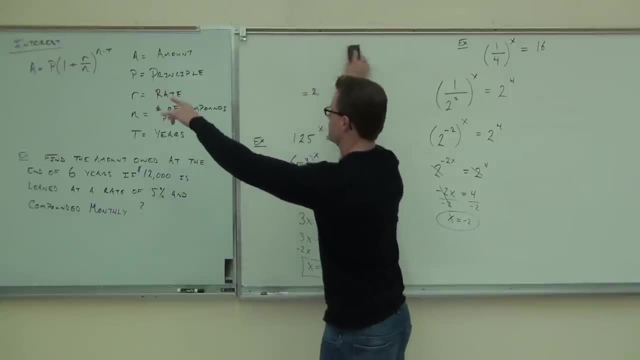 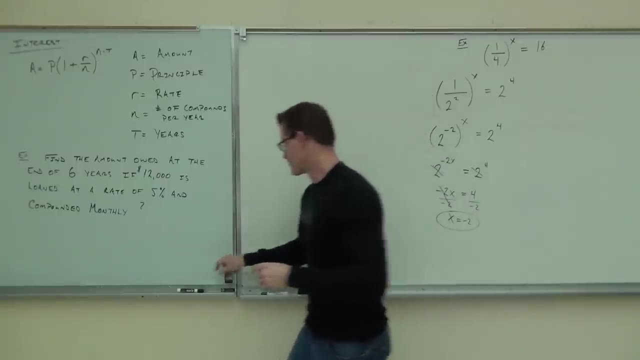 rate of five percent Compounded monthly. Can you fill out that formula with those numbers? This is the only example you get yet, so hopefully we get this one right the first time. First thing: do we know the amount? No, that's what we're trying to find. 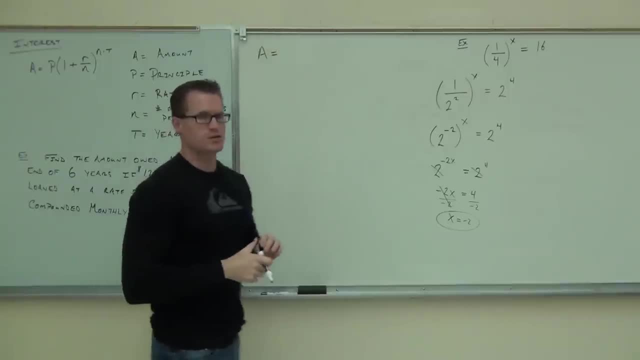 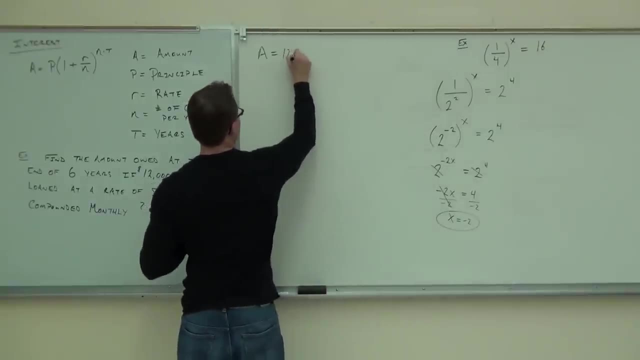 so we don't know what A is. Do you know what P is? P is your principal. it's how much you start with. How much did you start with here? 12,000.. So we're gonna have $12,000. 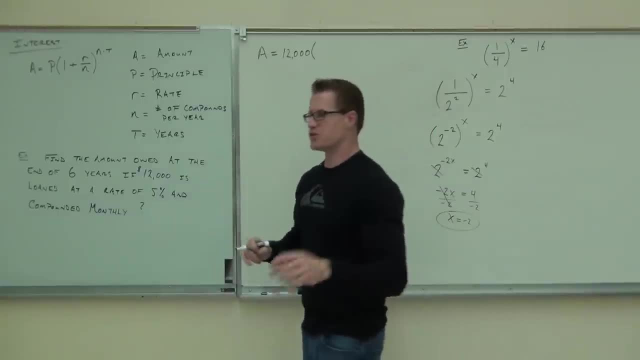 Then we have a parenthesis, because all we're doing is filling in that formula That one never changes And the plus never changes. How much is your rate? What would you say? your rate is Five. Now are you gonna put five? 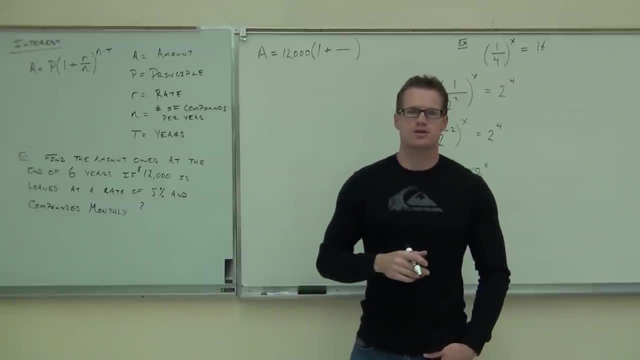 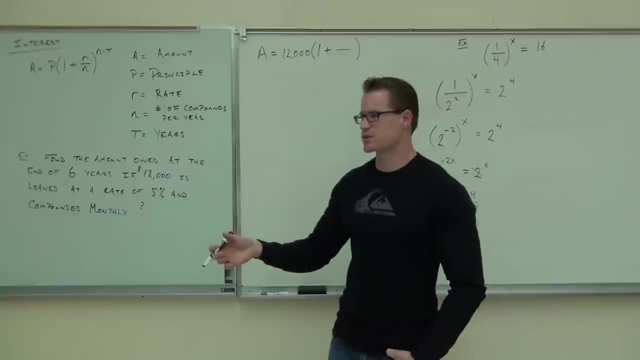 .05.. Why are you gonna put .05? Because it's interesting. So if I say 5%, 5% is .05, are you with me on that? If you put five, that's gonna be like 500% interest. 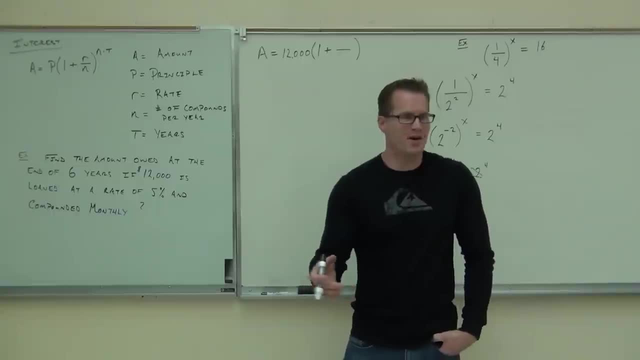 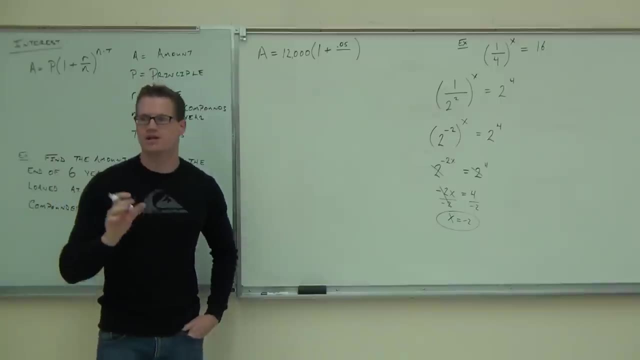 No one's gonna pay 500% interest, right? You'd be so broke buying this car. it'd be ridiculous. Now this is .05, because that is your rate. rate is .05.. It's a percentage. You translate that to a decimal for your equation. 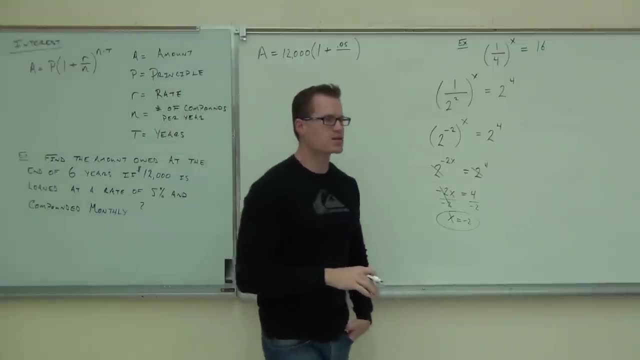 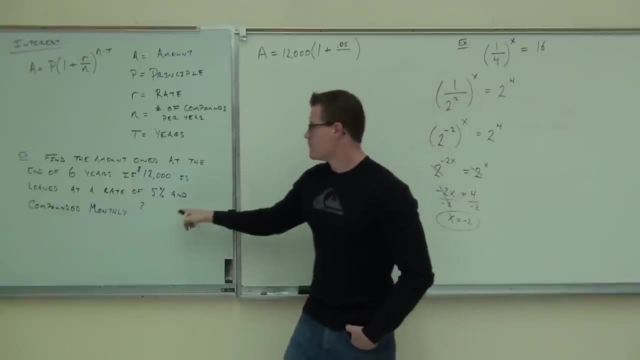 Are you okay with that one? What is your N? N's the hard one that people get tripped up on. Usually, percent is fine, unless they just do .5.. You're not gonna do .5,, you're gonna put .05.. 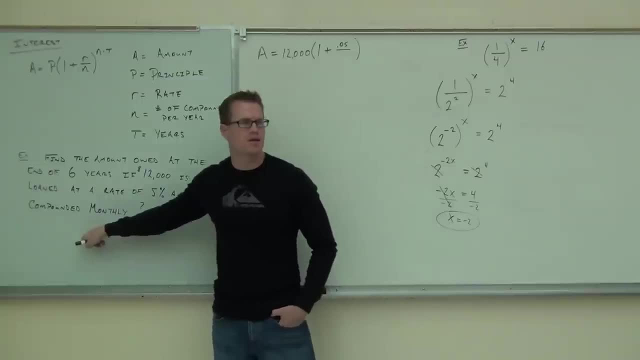 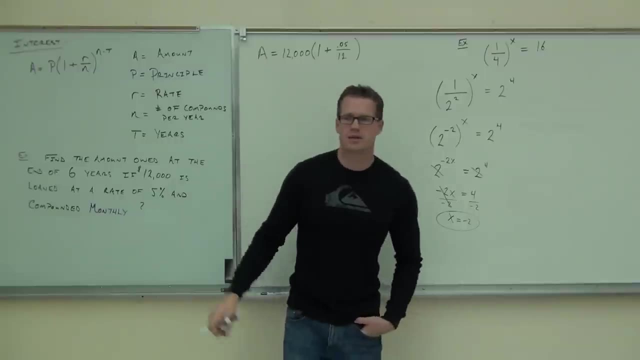 Monthly compounded monthly. this is how many times you were compounded a year. How many months are there in a year? 12.. Then you're gonna put a 12 here. Also, notice that your exponent is N times T, And so you're using that number twice. 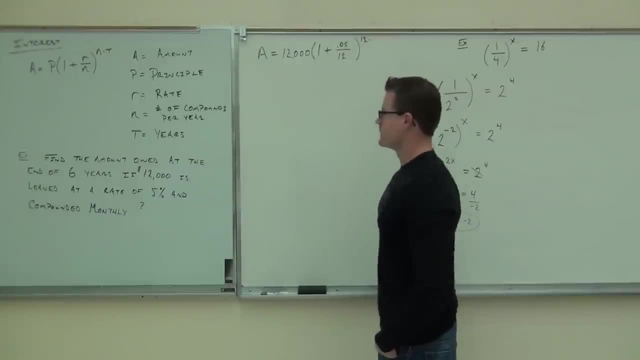 If you have 12,, you're gonna put a 12.. If you have 12 here, you're also gonna have 12 here. that's your N times T. What's your T in this case? Six, Six years, okay. 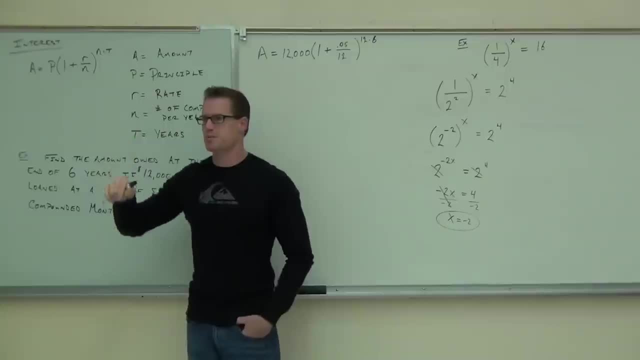 How many people feel okay with filling out the formula. Now that's all great, but you gotta be able to do the math right on your calculator. This is a calculator problem more than a math problem. Here's how you do it without having to round. 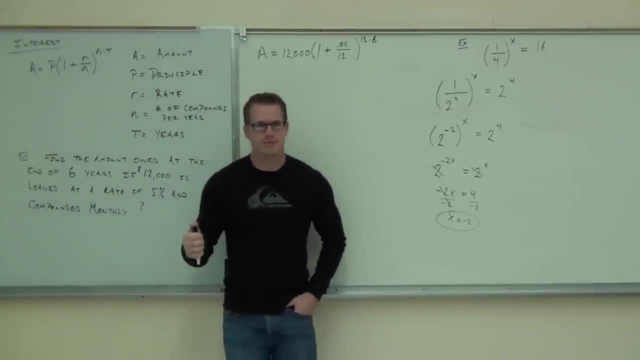 because you cannot round this. If you're, let me ask you a question. If you're in the car business or banking business and you go, well, I don't really know how to work that right, so let's just round it. 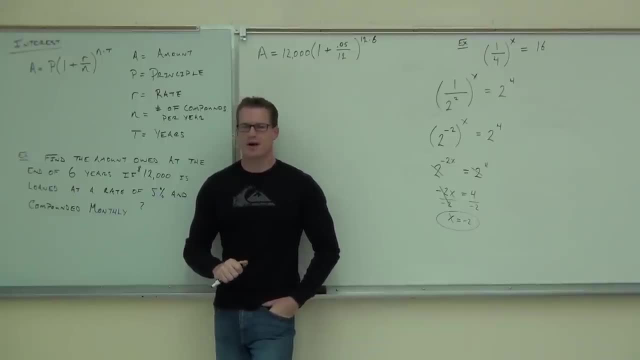 Are you gonna be in that business very long? No, If you're off by a penny, you're probably gonna get fired. Okay, cuz banks don't mess around. They want to the penny accurate, I want to the penny accurate. So you can't round any of these numbers, none of them. 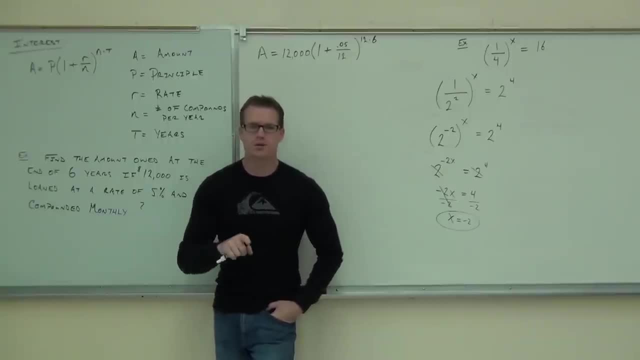 Are you with me? Can't really round any number. The only thing you're gonna do first, without doing this all in one step. I'm gonna show you how to do this all in one step right now. You're gonna want to know that, right. 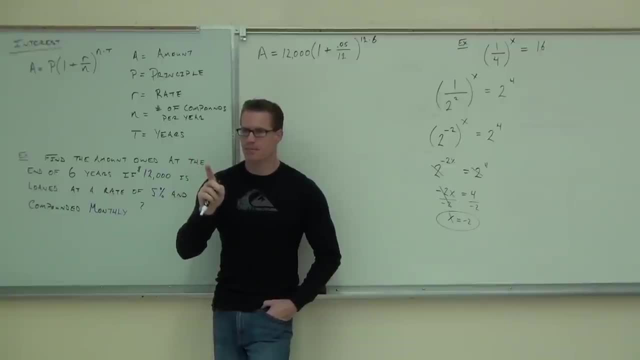 Cuz you don't want to write down a whole bunch of long numbers. Let's say you do it all in one step besides the first one. The first one is figure out what that number is first. It'll usually be something pretty easy like 12 times 6, or. 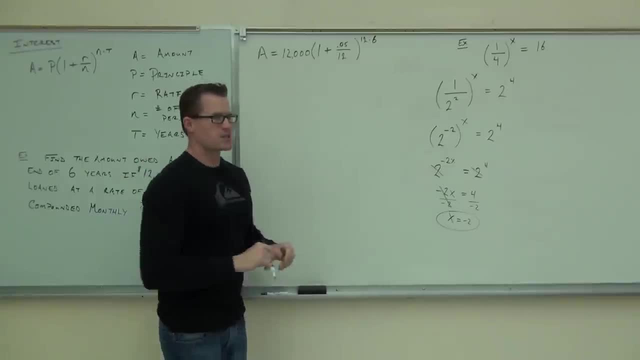 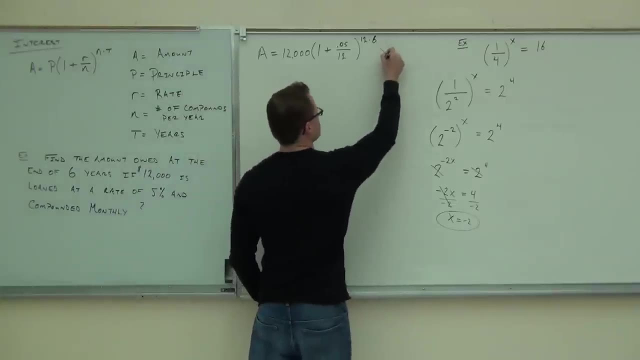 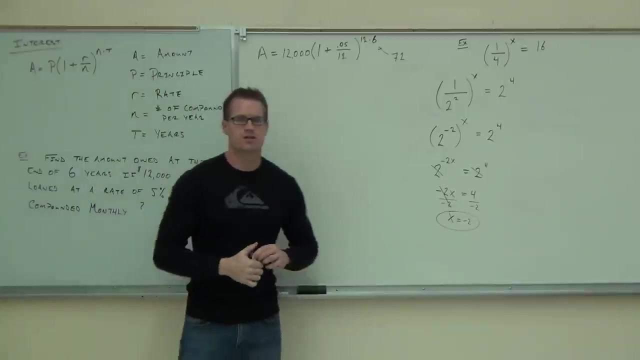 it'll be an integer number, it'll be a whole number: 12 times 6,, 12 times 72,, 72?? So you're gonna write down 72.. Now follow me carefully. Here's how you do this. 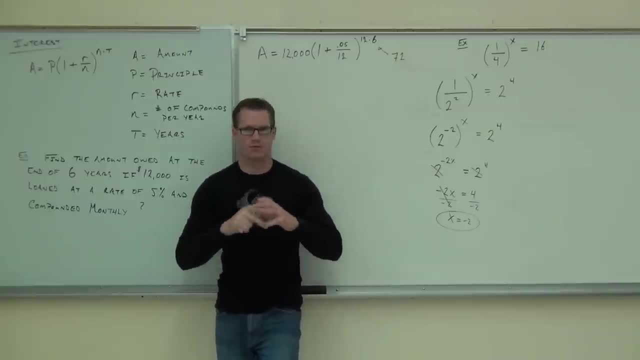 You're gonna do this all in one step. Just listen to what I'm. I'm gonna talk about your word from the inside out. We're gonna do this a little bit different than how it's written. First thing you're gonna do: you're gonna do this one. 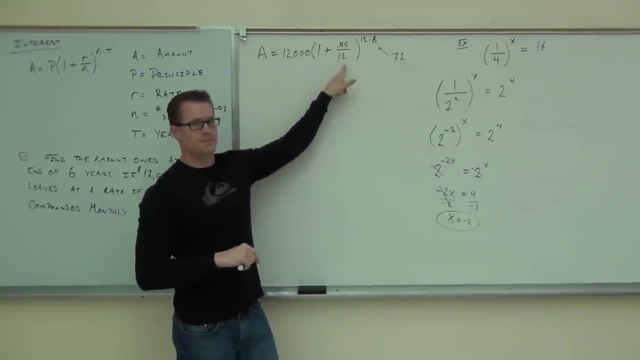 So on your calculator, plug in .05.. You got it. Divide by 12. Press equals, Add 1,, so plus 1. That's you right here, right now. Press equals, You should have 1.0 something. 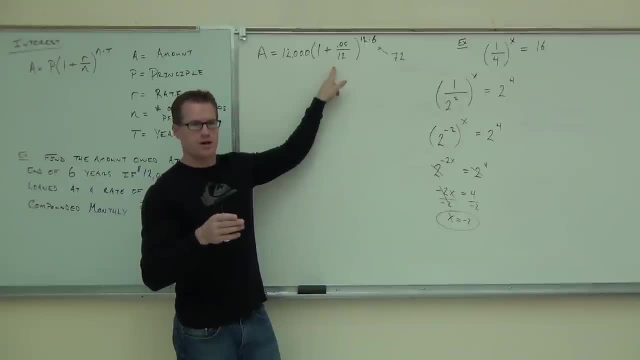 0.05.. 0.04.. You should have 1.004.. You have that Mm-hm. Okay, now find your exponent button, say to the 72nd power. That's why you need a calculator. 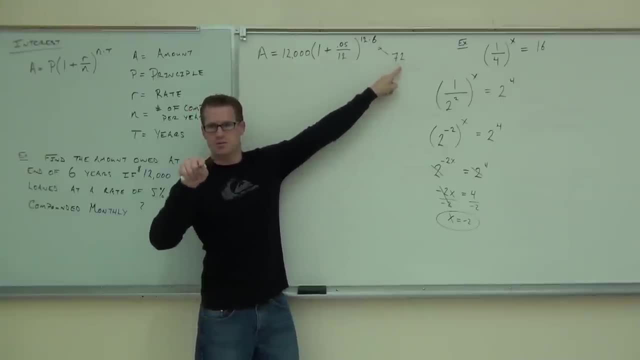 To the 72nd power. So to the 72,. did you get that? Mm-hm Press equals 0.34.. How much 0.34.. 0.34? Anybody else have 0.34?? 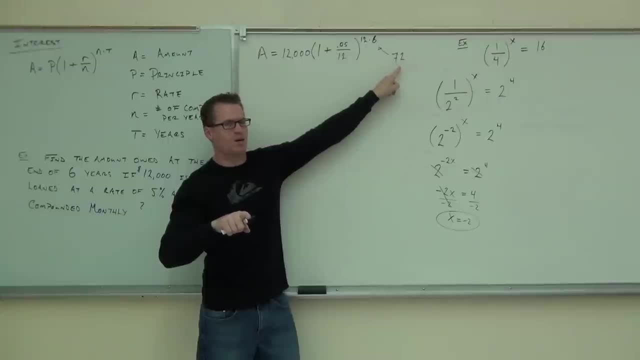 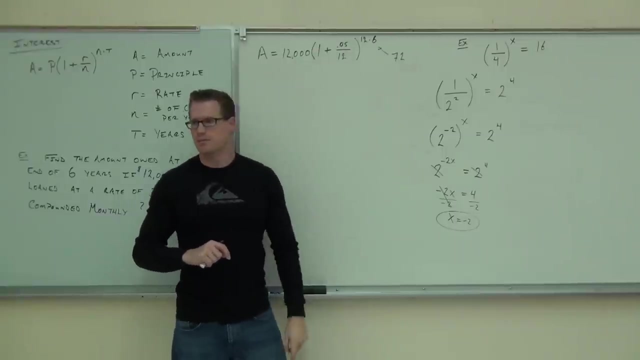 To the second power, To the 72nd power, 72nd, so to the exponent of 72.. It should be 1 something, 1.14.. 1.34 something. You got that Now. after that, multiply by 12,000.. 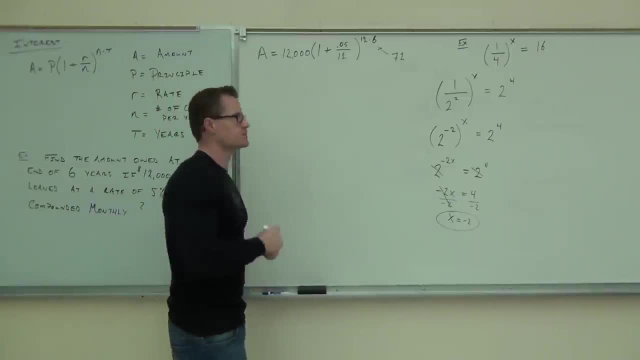 Press times 12,000, then press equals, And that will give you the amount that you're owed all in one step. If you didn't catch that the first time, watch that video again or come and see me after class and I'll show you how to use your calculator. 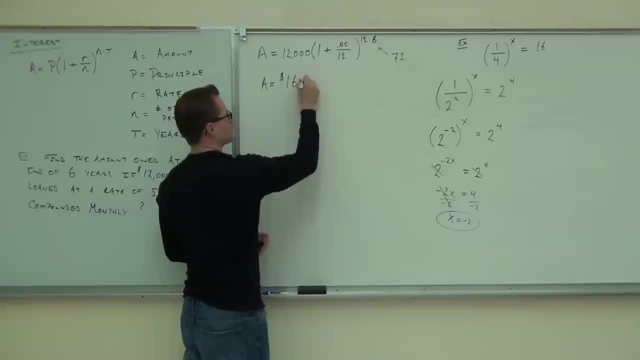 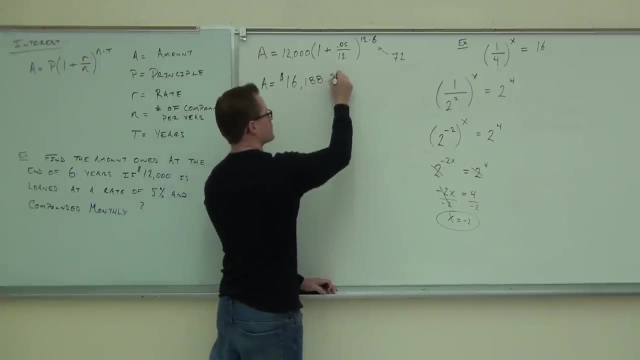 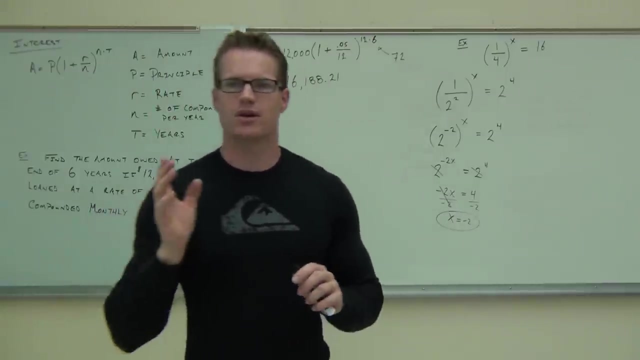 How much is it? 16,000.. 188.. Point what? 21.. Is it rounded correctly? You need it to the penny accurate. Now, this is what this implies, though This is not a realistic example, because when you have a car loan, you usually pay some. 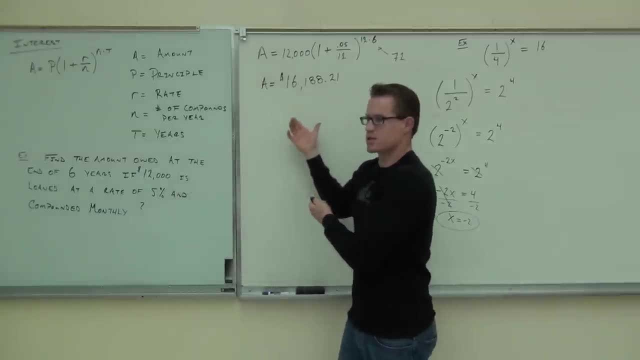 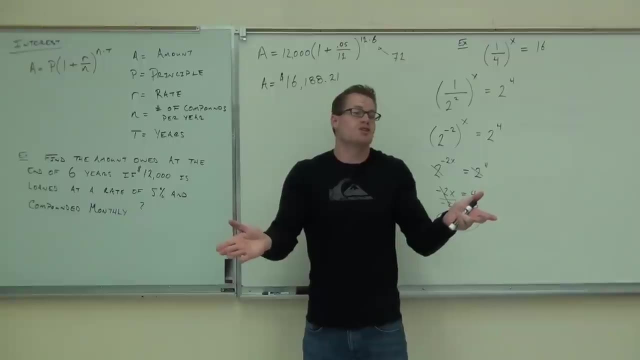 each month, right? So I mean, you're not going to owe this at the end of six years? This is how much you would owe if you didn't pay anything. and they said: you don't owe us a dime, Just wait for six years and pay it off. right then? 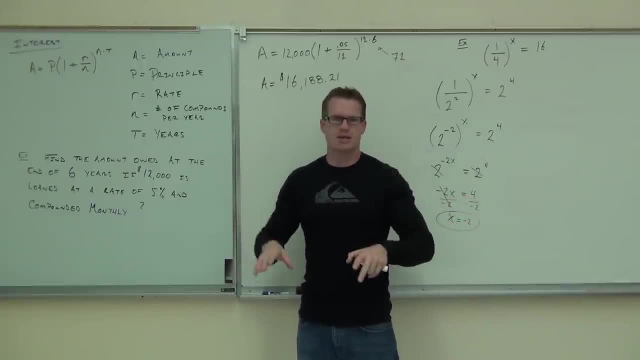 That's how, like the furniture stores work. When they say: you don't owe us anything, You don't owe us anything- No interest, No payments For four years. Then at the end of four years they go: now you owe us the money. And you go: my couch is a piece of crap. now I don't want to pay you five grand for my couch. It sucks. They go sorry. Yeah, that's how they work. Car companies usually don't work like that. They say: you owe us a little bit each month. That way you don't just default at the very end and say: I'm not paying you a dime. Ha-ha, Take the car back. It sucks now. So then I can do that. 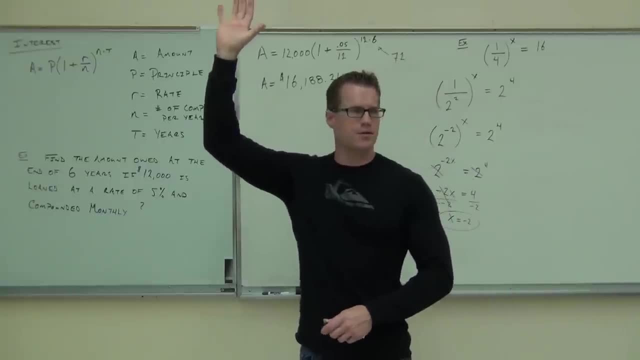 How many people understand our idea here. Now, the only other thing I've got to show you with this second example is I'm going to show you how to do it. So what I'm going to show you with this section is: this is the thing. 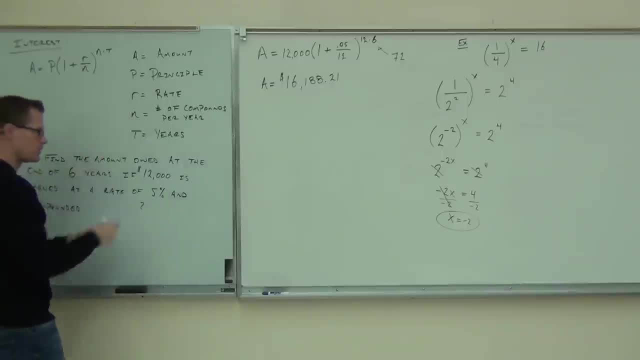 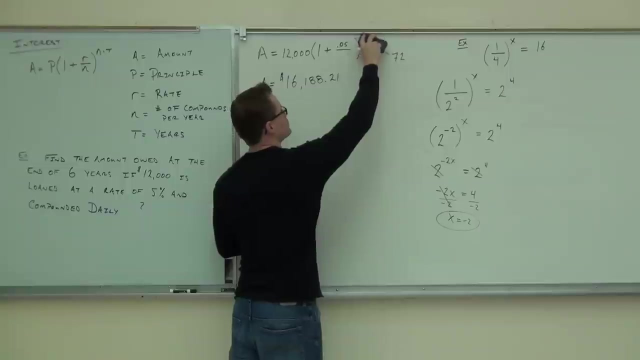 Everything can change, But this will change the value of your amount. What if I said now, compounded daily or weekly, Let's do daily. If I do daily, what does our n change to? Nothing else would change. Now, if you want to do that real quick, 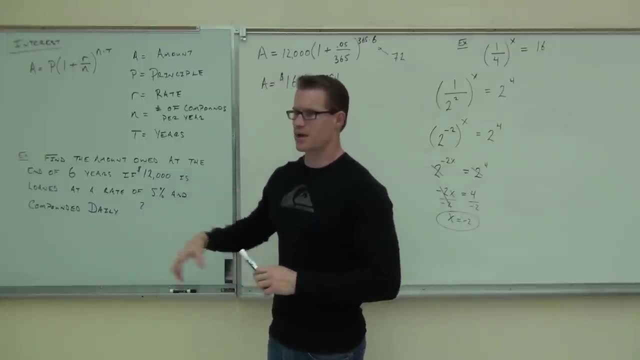 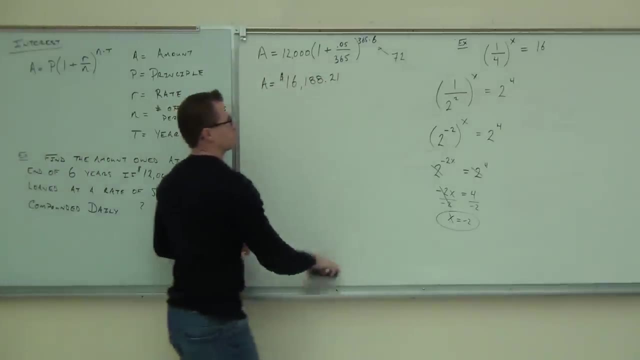 Why don't somebody do that? I'll write down what weekly and semi-annually mean for you. Do that real quick and find out if this is much different. Okay, So do the same operation that you did. Of course you're not plugging in 72 now. 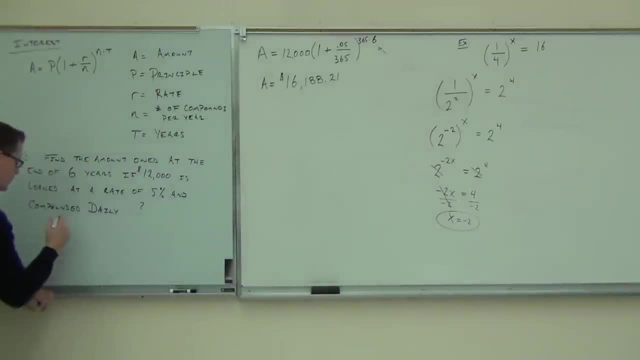 You're going to plug in 365 times 6. Okay, And then it's going to be $2,500.. You're going to make $3,500. And then I'm going to choose $5,000.. So here I have my $3,500. 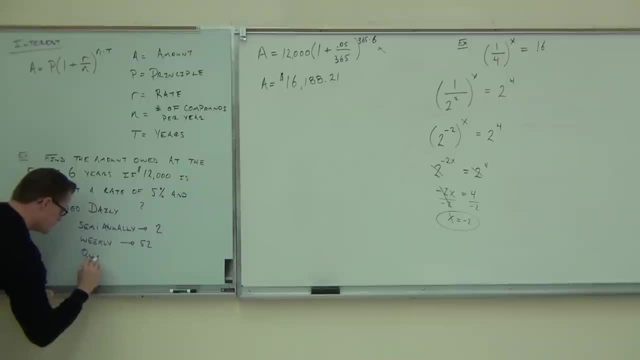 So here's my $44,500.. This is going to be $3,500.. There are still $5,000, but I'm going to use this much. Let's do it $3,500.. Again, this is a little different. 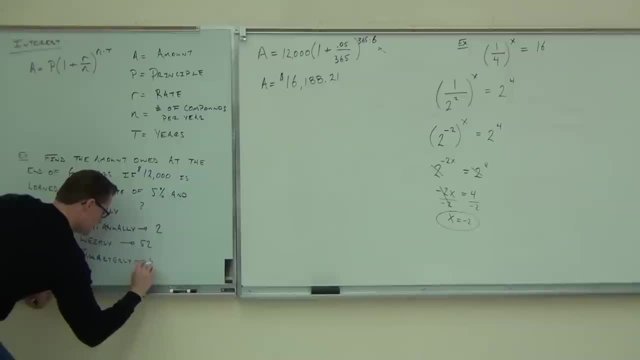 Here's my $3,500.. I'm going to use this much more. Let's take a look at the last one. So we're going to do this much. We're going to take a look at this plus. So I'm going to go out. 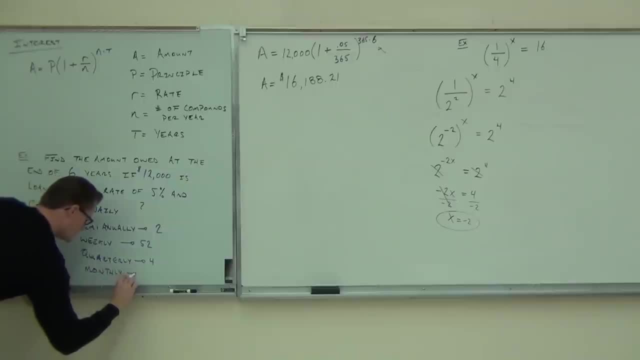 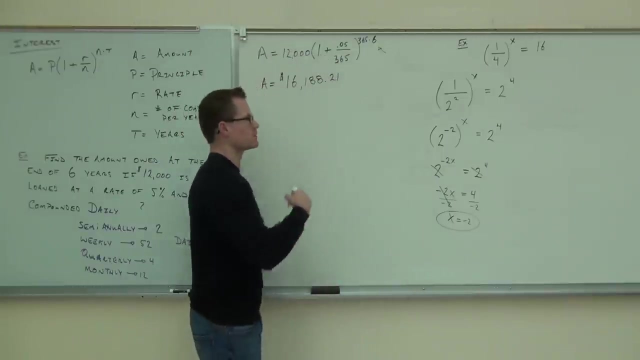 I'm going to drag it, I'm going to go down, I'm going to go up. Did anybody get it Should be 16,000, like 200, something, Almost. What is it? It's 16,197.97,, almost there.